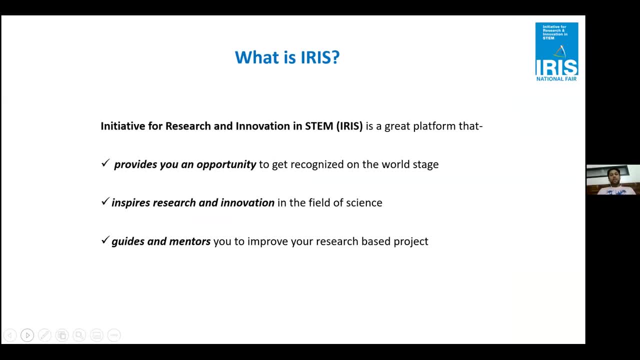 Thus, I would like to begin with. what is IRIS? Initiative for Research and Innovation in STEM is a platform which provides you an opportunity to recognize on the world stage. We inspire you to research and innovation in the field of science. IRIS guides and mentors you to improve your research-based project. 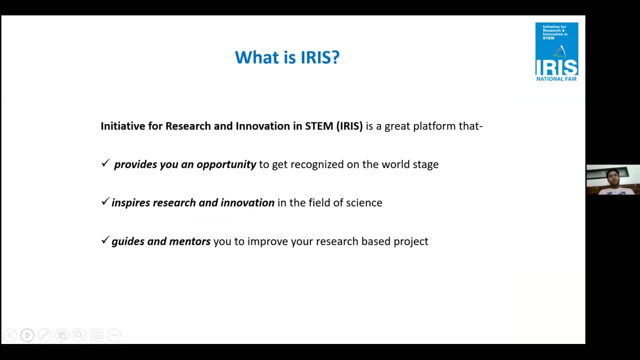 IRIS. we invite students to participate in IRIS with a research-based project, Something which is novel, which has never been done by students before, Or something we would not suggest. Not a new invention, but something which has been done before. 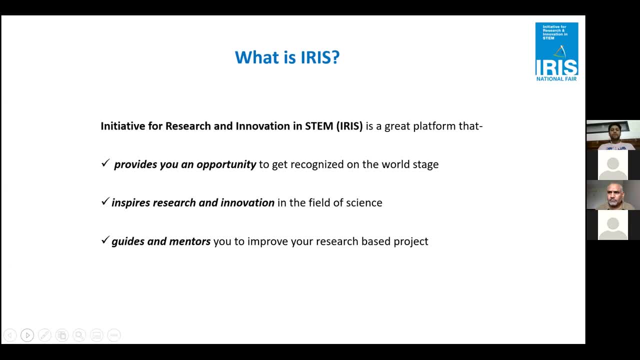 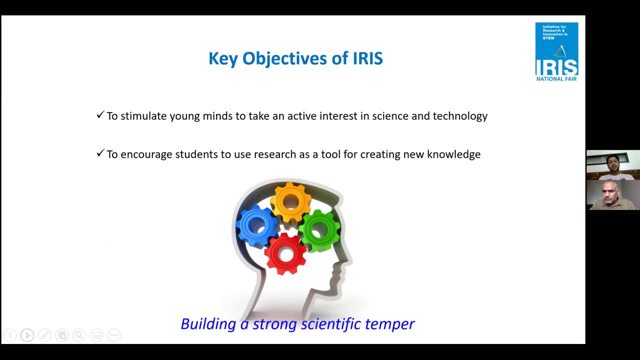 But you are bringing your own innovation in it. Our objective is to stimulate young minds to take an active interest in science and technology, And we want you to use research as a tool for creating new knowledge and build a strong scientific temper So that going onwards when you grow up. 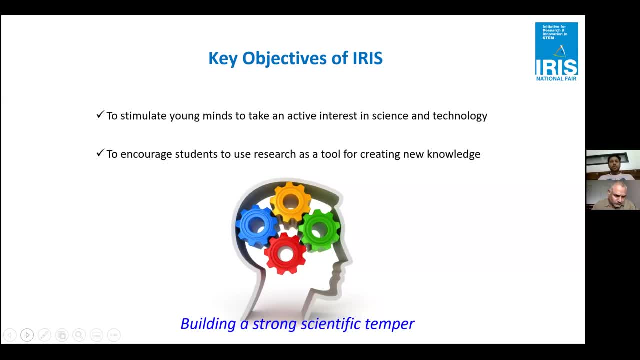 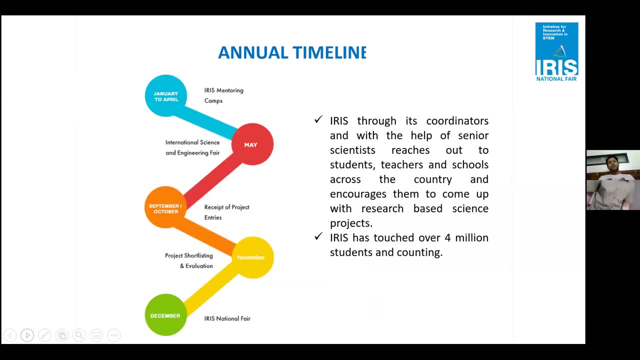 undergraduate, you go to your, you do business or you do any job. You use science as a tool, research as a tool and work more effectively. The annual timeline of IRIS: This is the time when we reach out to students and we ask you to work on your science-based project. 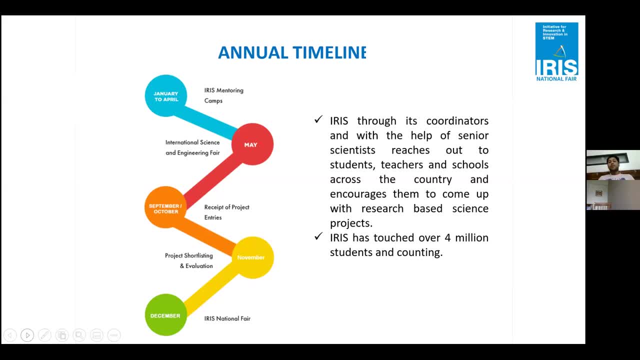 And submit your entries which are not yet open- We will be opening our entries very soon- And submit your project to IRIS. Once you submit your project, we have a panel of scientific review committee Which does project shortlisting and evaluation. From those bunch we select top 100 projects which represent in IRIS National Science Fair. 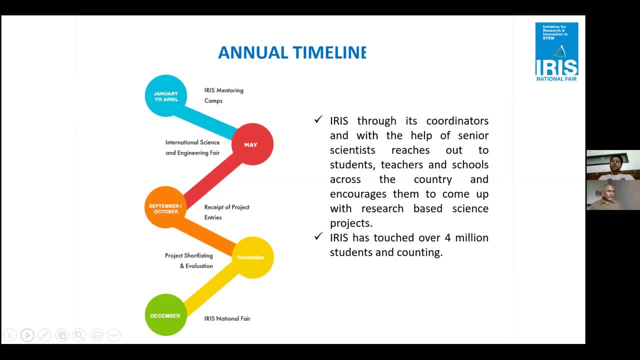 Which happens once a year. Last year, we conducted our national fair in the month of January. This year we are waiting for this pandemic to end To decide whether we will be going ahead with the national fair online or an exhibition session. IRIS, with its coordinators. we reach out to lot of students, teachers, schools every year. 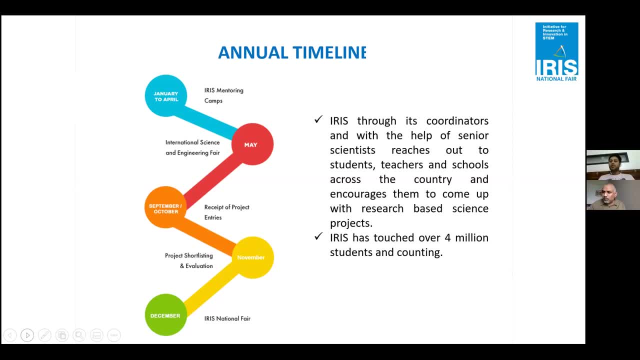 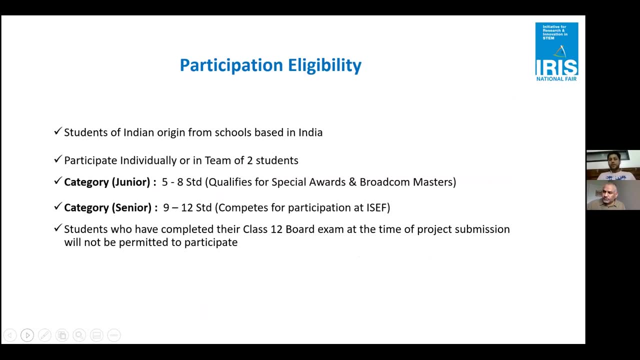 Till now, we have touched over 4 million students and we are counting. This is very, very important. This is very, very important for all of you: The eligibility to participate in IRIS: We allow students of Indian origin from schools based in India. 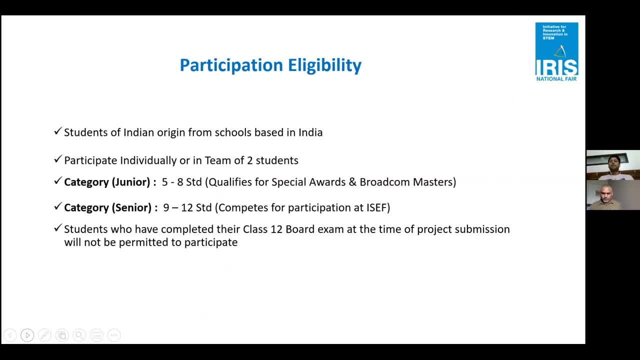 Please notice the point Schools based in India. There are schools- there are CBSE schools- which are outside India as well, And there are students who are Indian but studying in CBSE schools which are not in India. Those students are not eligible. 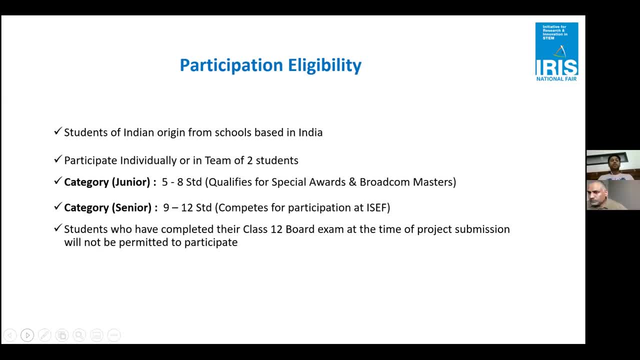 Hence we have written very clearly: Students of Indian origin. Also, if there are international students who are studying in India, They can be of son or daughter of some working professionals, of international people. They are not allowed to participate. Only students of Indian origin are allowed to participate. 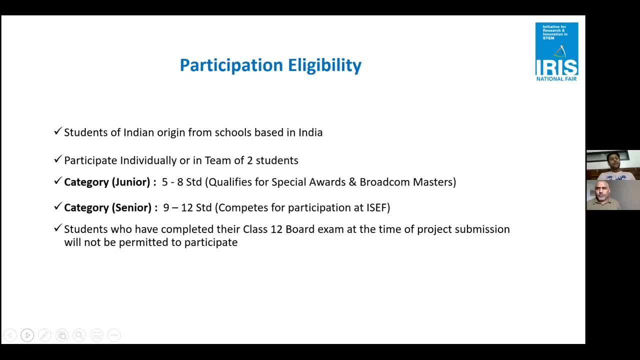 And those are from schools based in India. You can participate in two categories. One is Junior. Junior category is for 5th to 8th standard students And Senior category is for 9th to 12th standard students. Junior category students do not compete for ISEF. 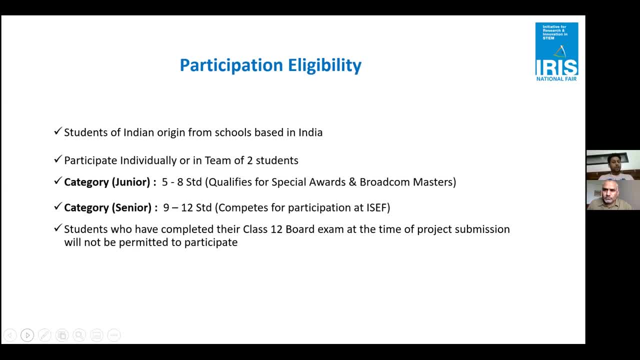 They win awards, But special awards in IRIS, And they get an opportunity to get Broadcom Masters Award. Broadcom Masters is basically an award. We select only one student which goes to an international platform along with Team India. Team India, basically, are the winners who win grand awards at IRIS. 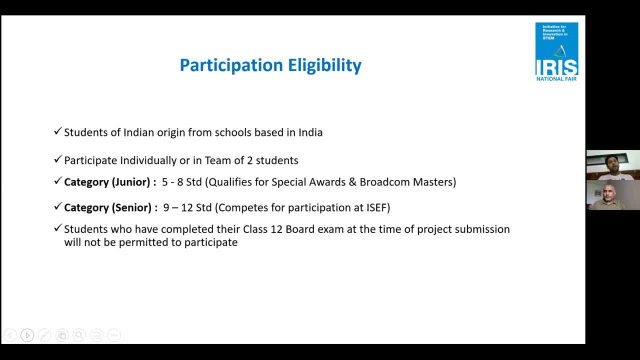 And Broadcom Masters winner also go with the team, But they have their own session at ISEF and do not participate or compete in ISEF per se. The Senior category students are 9th to 12th standard students. They are eligible for special awards as well as for grand awards. 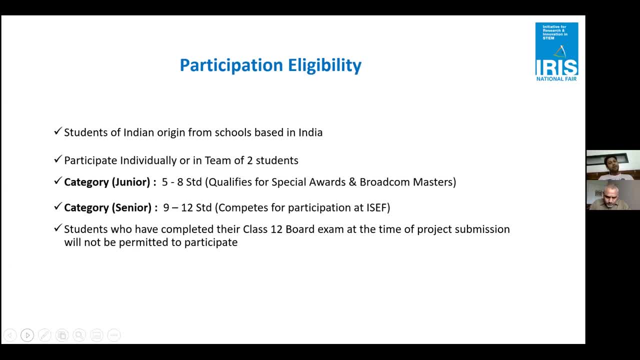 And the grand award winners go to ISEF. They represent Team India. The students who have completed their class 12 board exam are not eligible to participate. For example, this year the 12th grade students who have given their board exams in the month of March. 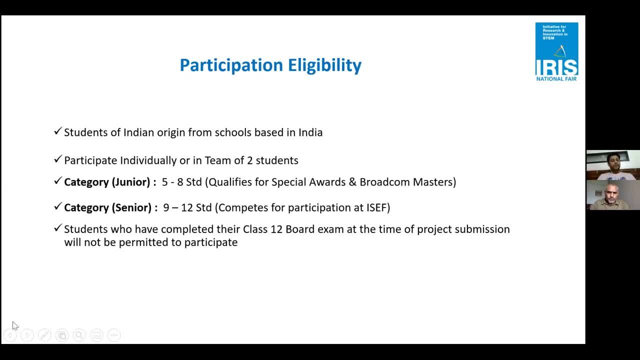 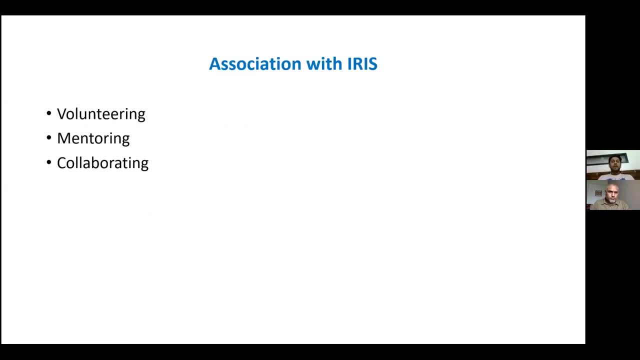 They will not be eligible to participate, But they are eligible to participate in IRIS. If you are an undergrad student or an IRIS alumni or a teacher. If you would like to volunteer with IRIS, you are welcome. You can send us emails or you can visit our website and register yourself as a volunteer. 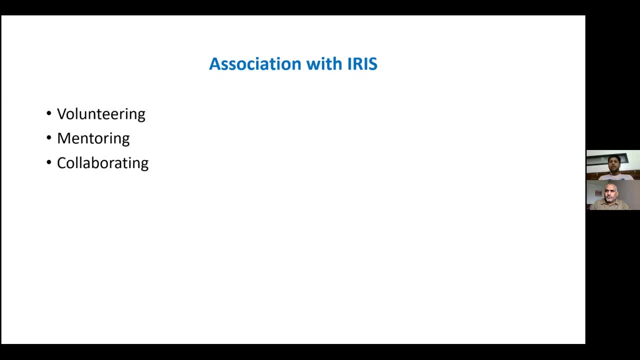 And you can support us in conducting our events. when we do- For example, we do IRIS National Science Fair, We do partner fair meets, We do workshops in schools- You can support us in doing the workshops and volunteer with us. Mentoring is only for the teachers or professors who are available and dedicate their time in voluntary work. 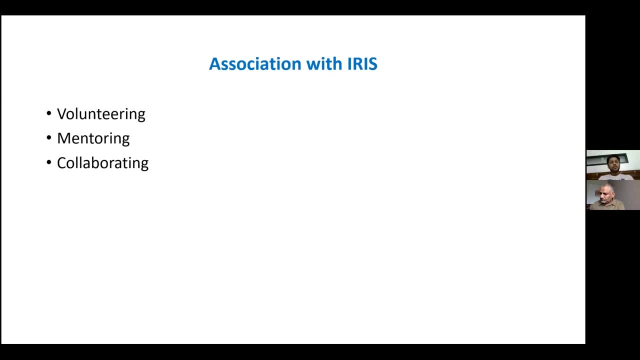 And support students in mentoring guiding students. There are a lot of students in India and they also contact us that they are not able to find right mentors for their project. You can register with us And you can be a part of mentoring team of IRIS. 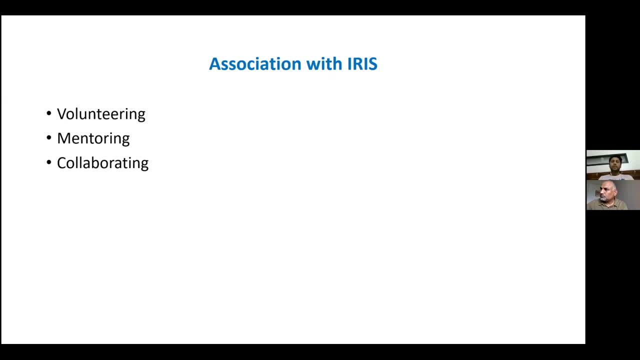 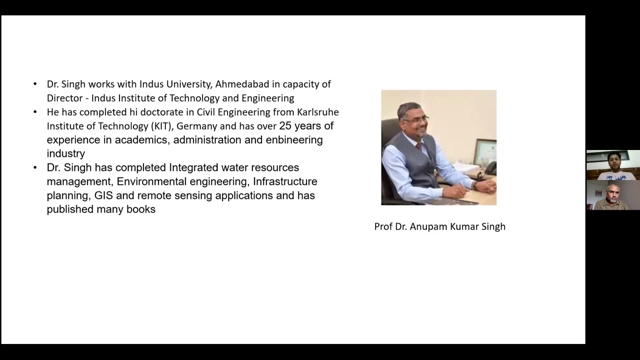 Then the collaboration. Collaboration is for the people who represent organizations, which can be government or private organizations, And they would like to sponsor IRIS or they would like to participate or support students in their projects. They are welcome to join us. Hence, I would like to firstly welcome Prof Dr Anupam Kumar Singh for joining us today. 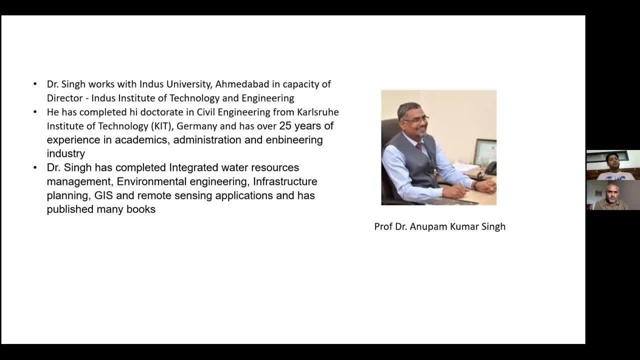 Our expert, Dr Singh. he works with Indus University, Ahmedabad in capacity of Director Indus Institute of Technology and Engineering. He has completed his doctorate in civil engineering from Karlsruhe Institute of Technology, Germany And has over 25 years of experience in academics, administration and engineering. 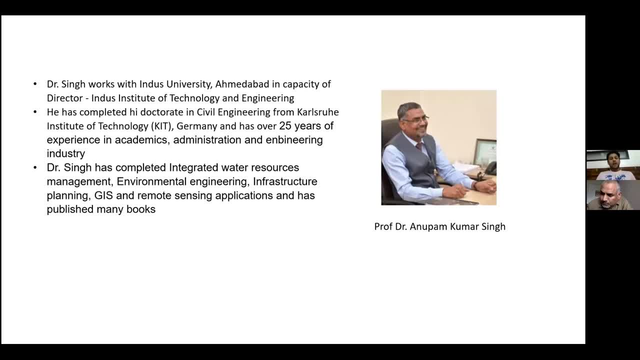 Dr Singh has completed integrated water resource management, environmental engineering, infrastructure planning, GIS and remote sensing application And has many books published by him. I would like to welcome Dr Singh. Thank you, Shrey, It's a pleasure actually. 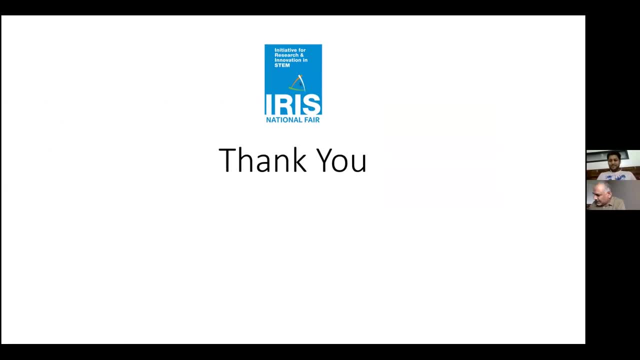 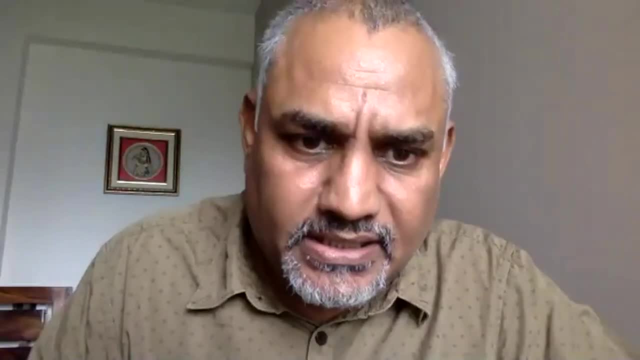 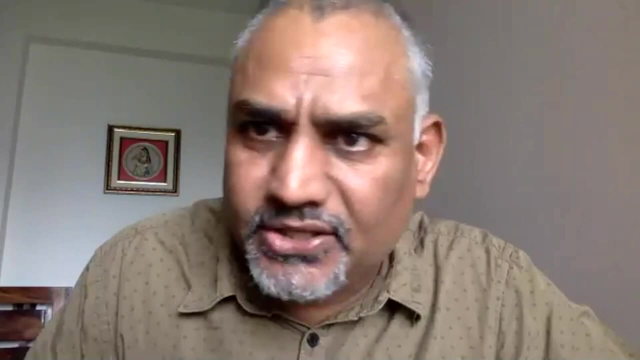 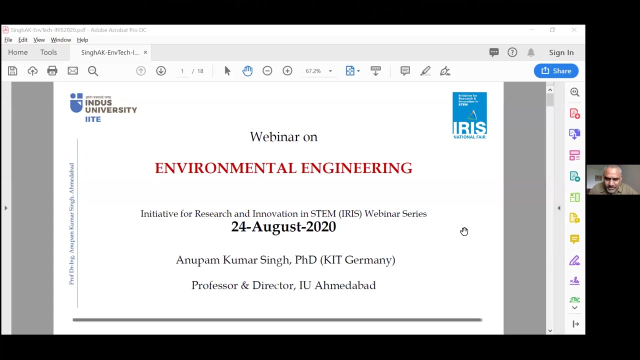 To be with Dr Singh. I love you And I know it's a, So it's indeed a pleasure. I would just take a minute. you know, I would like to share my screen with all the students who are Yeah. 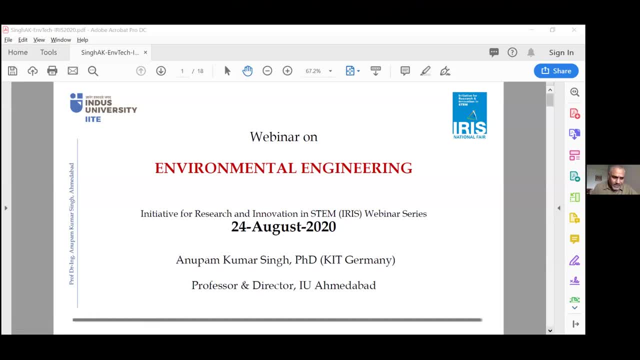 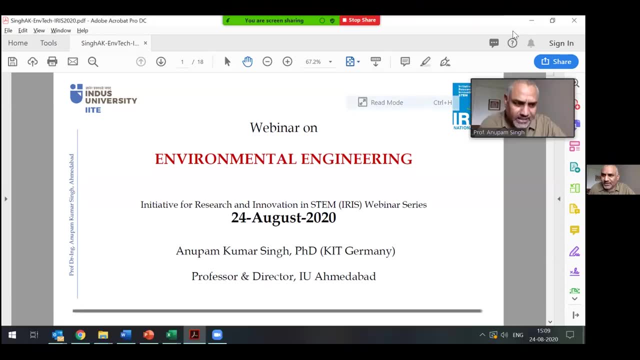 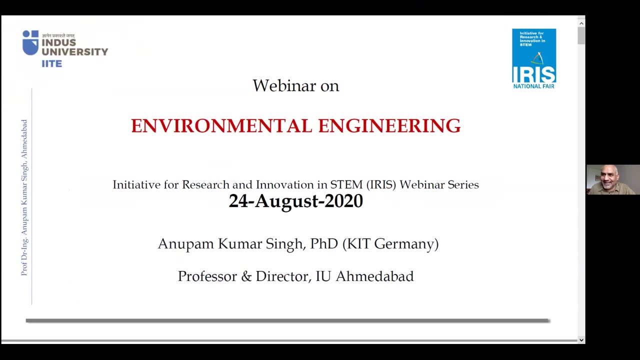 Oh wonderful, Thank you, Thank you, Thank you. Yeah, Thanks, Shrey. Thank you. Thank you, Thanks to the students. I tried to be a bit of a And uh by uh. it's a great pleasure actually for me personally uh to be with school students uh, because I often uh teach college students. 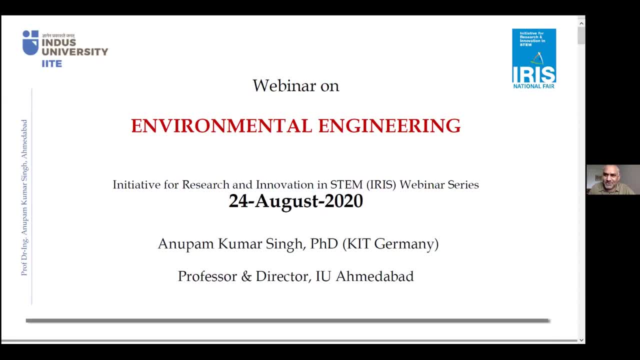 I teach engineering students who are at bachelor's level, who are at master's level, who are at PhD level, Uh, so it's indeed a great pleasure actually to be with these colleagues. I would like to put on record my thanks to Iris, Mr Shreyas Singh, who contacted me. 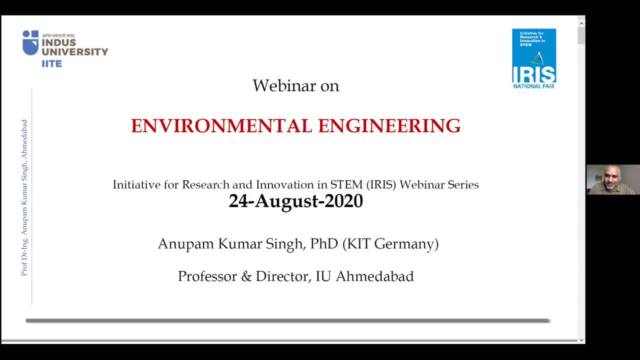 very early, and also Shashak Kumar, actually for this one. This presentation is just a tool for all of us not to go out actually of the way, but you all are free to stop me any time if you like, or you can ask me question at the end. 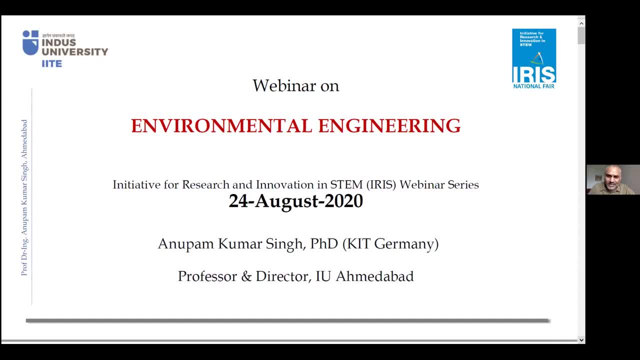 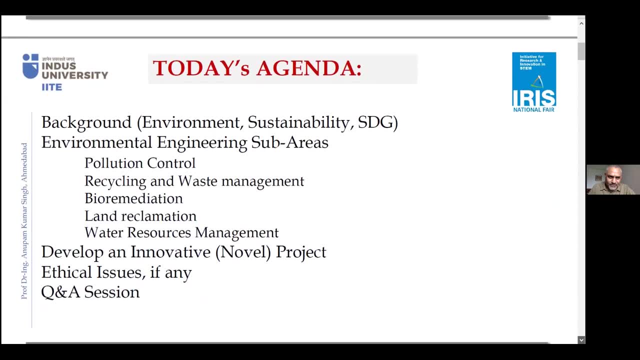 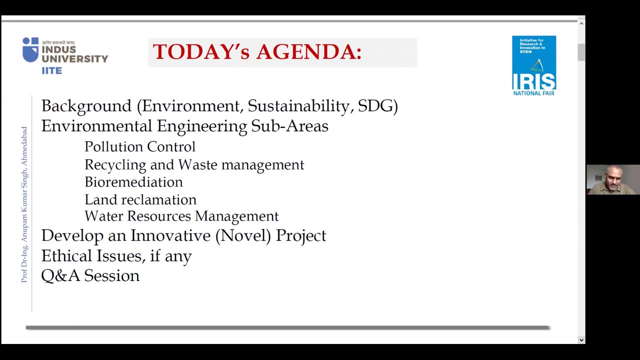 So the agenda for today is: can you next one, please? Yeah, so today's agenda is that I would like to talk a little bit about the environment and the sustainability and how various sub-areas of this environment are playing a crucial. 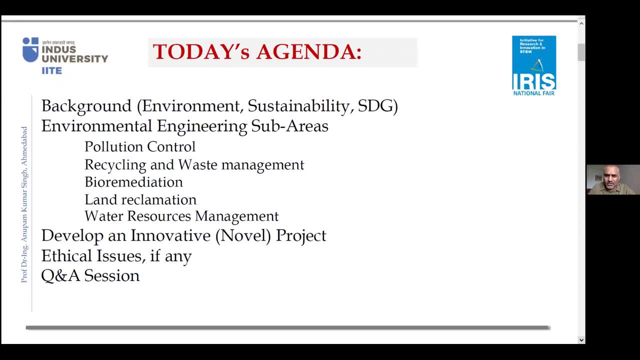 role actually for human habitation, when we know that this COVID has happened very recently and we know that this is not sustainable. We also know that it's putting a lot of barriers on our movement- not only movement- on our thought process, on our development, on our psychology and also, many times, on our capability. 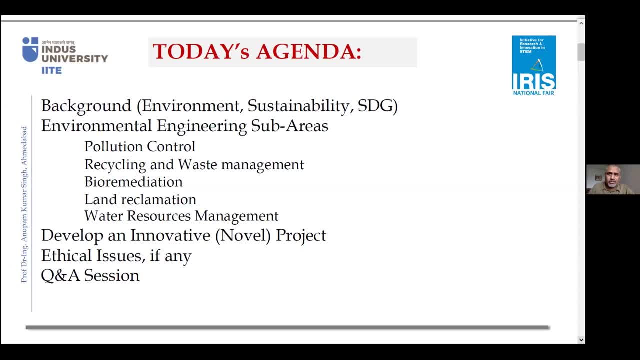 So therefore, actually, I would like to show you something you know, mainly relevant to India, that how this is unfolding, How can I work? or if I work in the other area, then how can I work? yeah, So I would like to talk a little bit more on that. 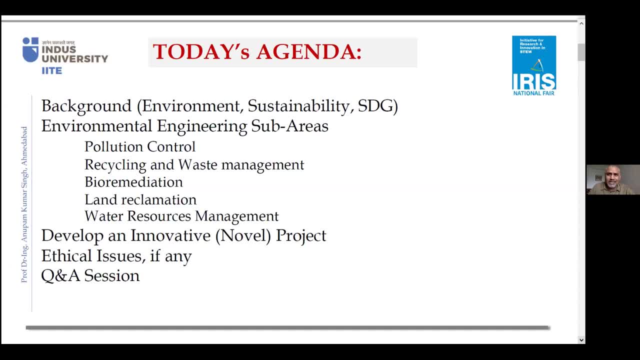 I have unfortunately not done much on land reclamation, but I think at the end I would like to discuss about that further. I will also give a first, A further idea that how to develop, because the projects which are being done right in. 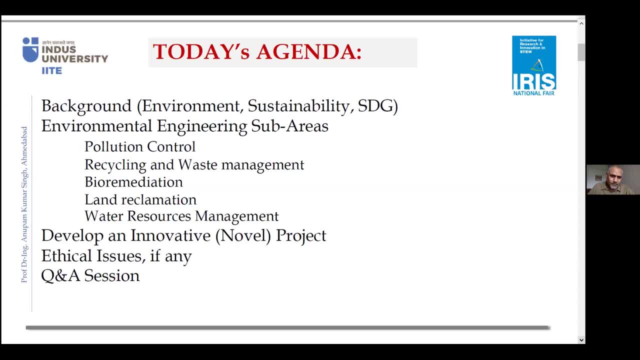 India unfortunately are not converted into a real prototype, or sometimes a prototype, then not in terms of to convert- you know those, you know ideas into prototype and prototype into product. And we have very strong now Indian patent aid system. you know under which some of 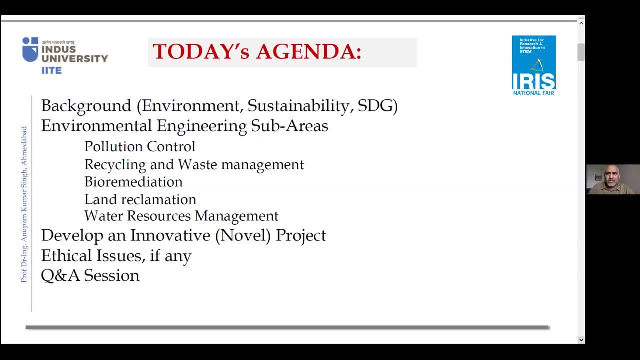 you could again, you know, try to convert this idea into your own name, you know, for at least next 20 years. And then there are a few ethical issues, you know, related to doing something or other, so I would like to talk that as well. 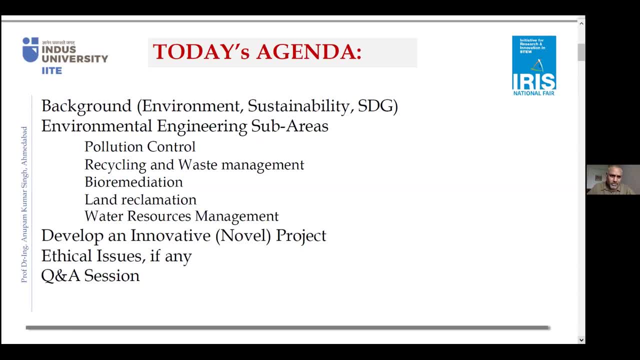 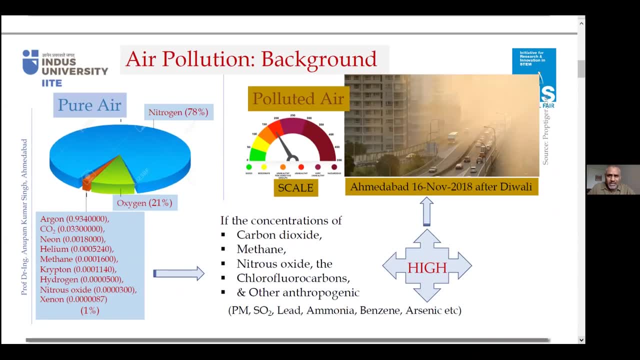 And finally, I will be, you know, open for question and answers. Next one, please. So when we see the sustainability, you know, we are often so-called confronted with daily reality in terms of so-called- you know, certain problems. that society, the society you know, 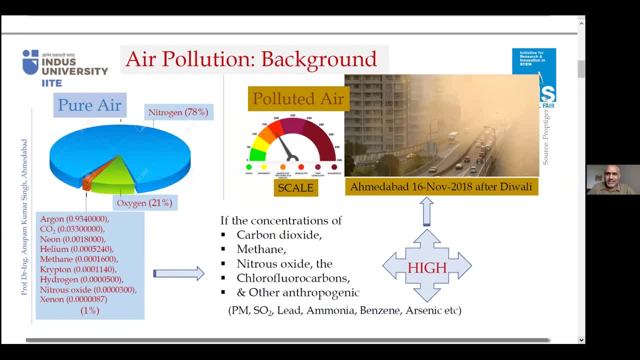 has to deal with. You know, You know Some of us might not have an idea of what that is facing. Now, when we talk about sustainable development, we say that sustainable development is the development, you know, which is doesn't compromise for the people who are supposed to come during. 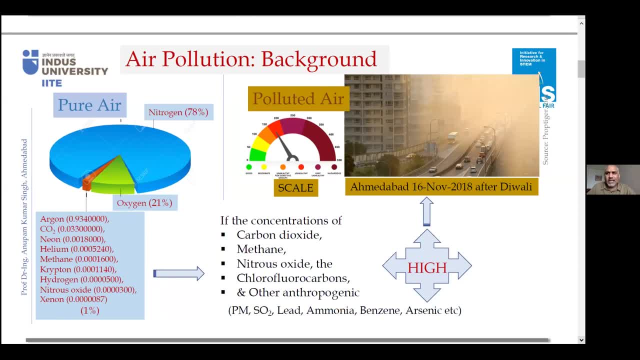 you know some point of time, let's say later. So this means if you are a school student, maybe, let's say you are going to Georgia, you are going to 발�onize, going to live 100 years, Yeah, so this means next 80 years. 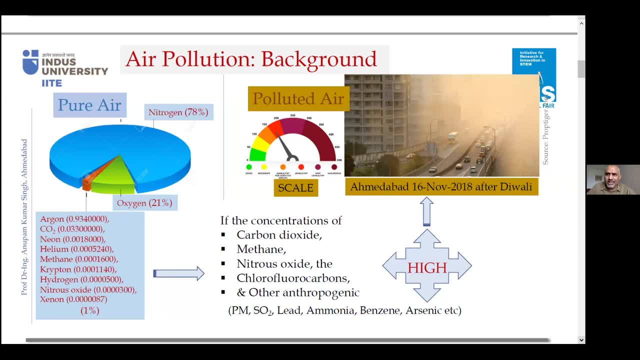 whatever the resources that we are having today, those resources must last for all of you, for next 80 years, or maybe next- let's say, I don't know- 85 years, right? This will happen only when we are conscious about today's need and when we are conscious. 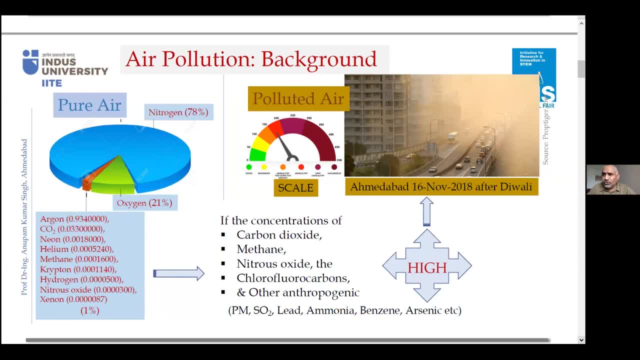 about issues you know, which are there, you know. So where is the presentation? I'm unable to see the presentation. Can you see the presentation? I am unable to see the presentation. actually, Yes, sir, Can you see the presentation, sir, live? 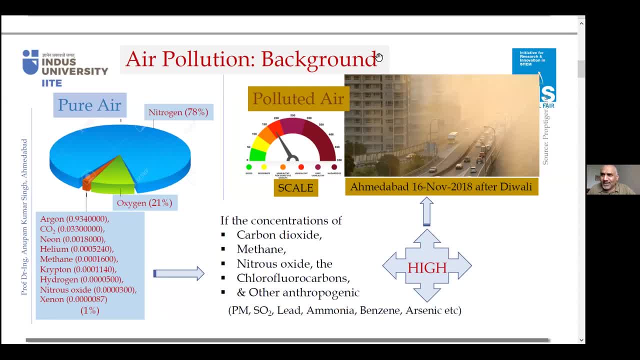 I don't know what has happened actually, because I am unable to see that actually. So, nevertheless, I have my own, yeah, okay. So therefore, the development has to be like that, yeah, And in other there are certain constraints. 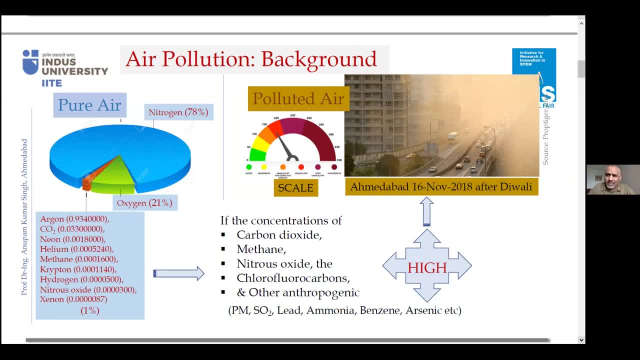 in that development, and one of the major constraints that we are facing today is resource availability and also second constraint you know that we are facing in terms of upkeep of those resources. So then we talk about the environmental engineering. Pollution is normally one thing. 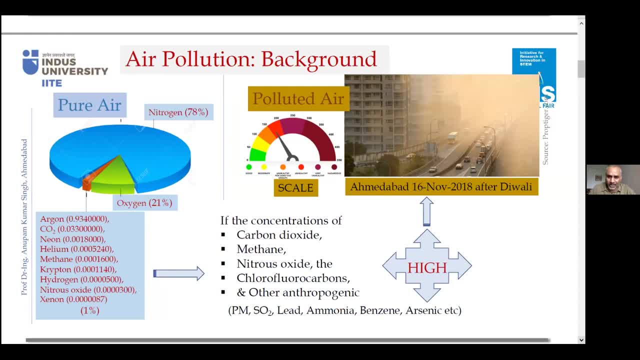 which comes to the mind of everyone, And I would like to focus mainly here on one parameter, which we call it air pollution. Now, many of you have studied in your, let's say, 9th, 10th, 11th, 12th, 10th grade, right. 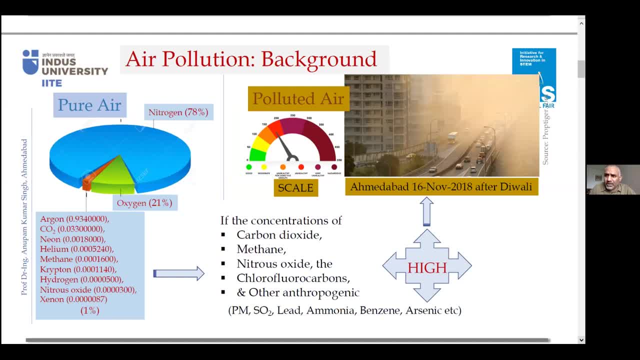 Any questions. standard that pure air is a combination of nitrogen, oxygen and other gases. So we say that nitrogen is approximately 78%, oxygen is around 21% and the other gases which are there, they are almost 1%, but are in a part of the frictions and mainly I have 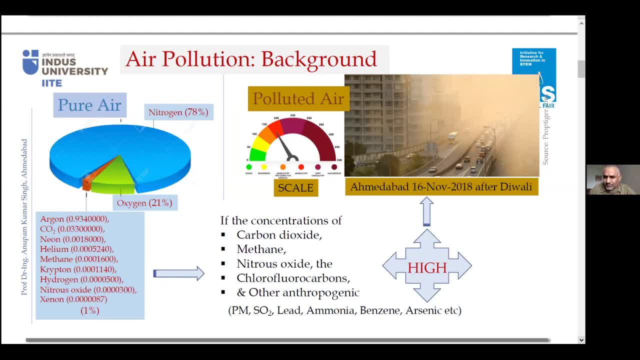 written there. it's the argon, carbon, neon, helium and like that. So what is happening when the concentration of these 1% gases actually changes? what happens? that our air actually become polluted. So even a small fraction of that can deter the air quality. 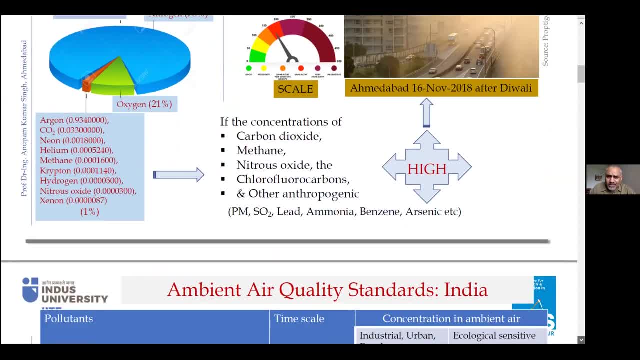 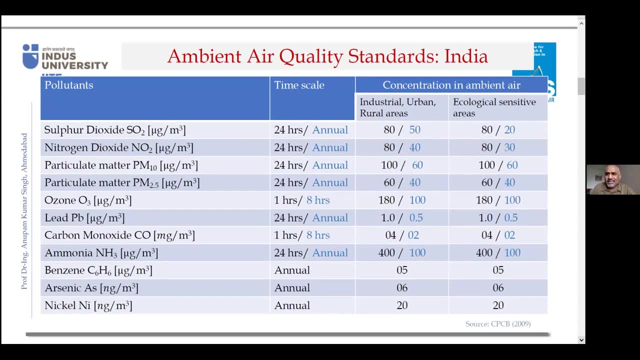 Now next one, please. When we are measuring actually this Ambient air quality- and I have brought some standards because there are often some standards- you need not to worry about these numbers. Just try to understand that there is an upper limit actually to these standards and there 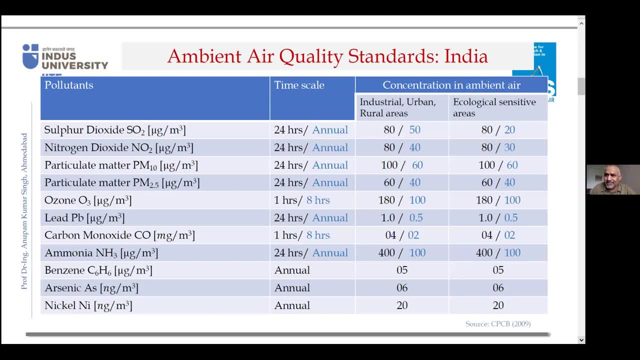 is a lower limit actually to these standards? okay, And these standards many times are either measured hourly or they are measured you know 8 hours or 12 hours or 24 hours, Or you know daily, monthly, weekly, annual, like that yeah. 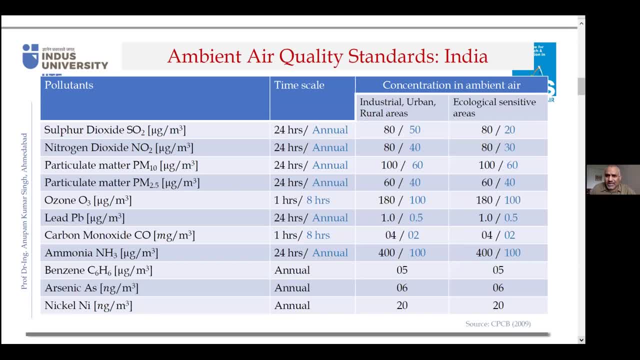 So, therefore, we have to make sure that, whatever the standards are there, actually we are able to meet these standards. The reason for meeting these standards is that most of, actually, the level has been kept in such a way so that these standards meet the sustainability criteria. 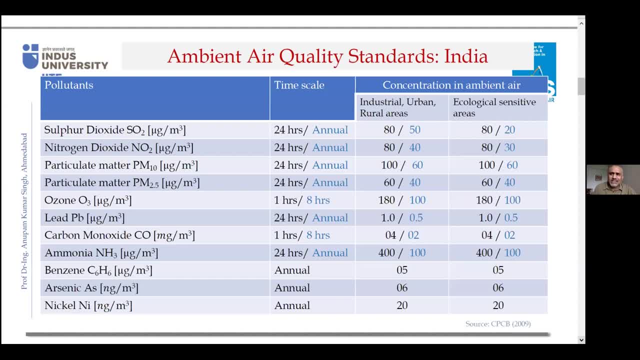 That's point one. Yeah, So I have mentioned in the beginning that development must be sustainable and therefore, if everything which is remained within the limit below this limit numbers which are given, then if it remains below that limit, this means the development is actually a sustainable. 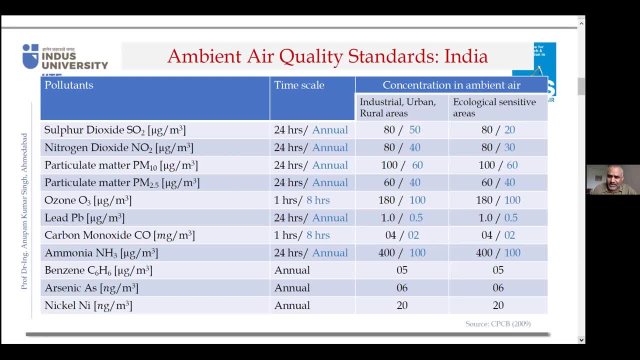 development. Okay, India has these different standards. India has this kind of a standard. If you go to Germany, their standards are approximately 25% better than other standards. If you go to Sweden, you will realize that their standards are maybe 30% better than. 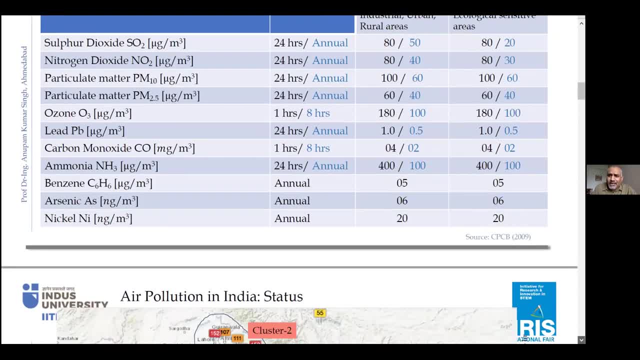 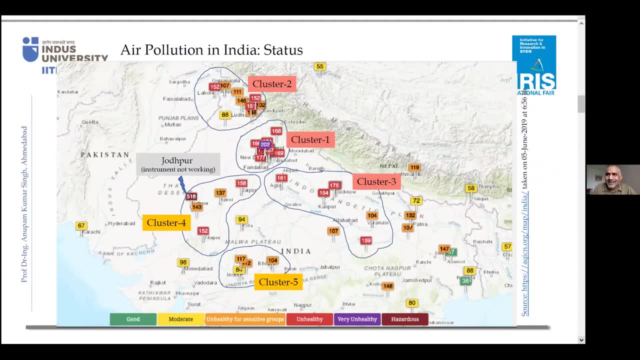 our standards. Yeah, Next one, please. So when we look at this air quality, air pollution, we call it air quality, you can say, because we are representing air pollution in terms of air quality, And I have told you that there is a lot of air pollution. 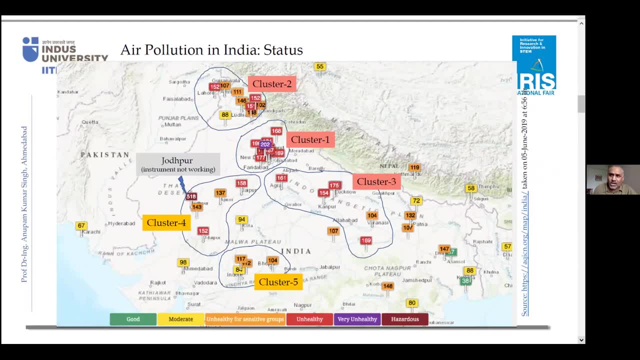 Yeah, There is a balance in terms of nitrogen, oxygen and other gases which were there, Yeah, So in India. if you see, this is the Indian map and you can very well see here that I have divided this entire India into different clusters. 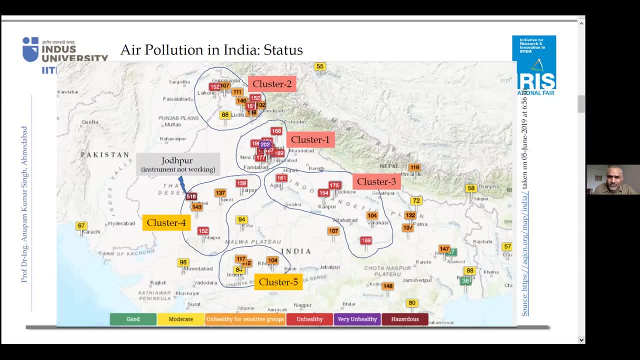 Right, So we have a cluster, Let's say, if you see the cluster, one which is we call it NCR cluster. This means National Capital Region consisting of Delhi, Faridabad, Kachipur- You know Kachipur- and Loni, and that entire area you know. 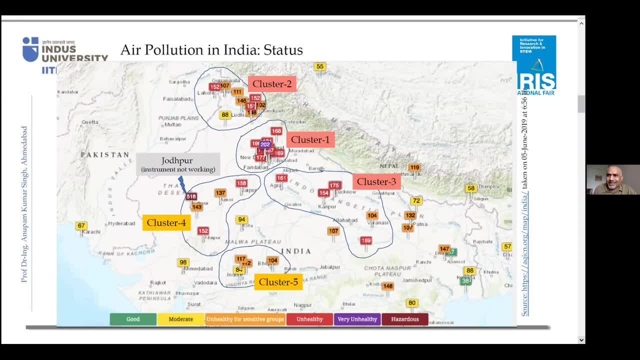 So this is one of the worst polluted actually cluster in India. Then we have another cluster which is in terms of the so-called in terms of industrialization. So we can say that this is Amritsar, Ludhiana, you know, Chandigarh cluster, cluster two: 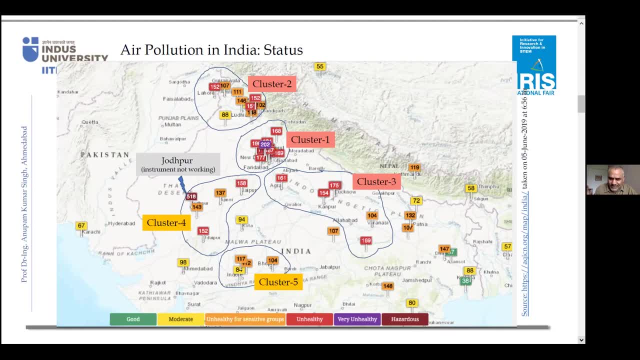 Cluster three: again, you know when we take is. you know we can say that it's like a Gangetic Plain cluster, you know, starting from somewhere- Agra, and goes until Banarasi, a little bit further down. 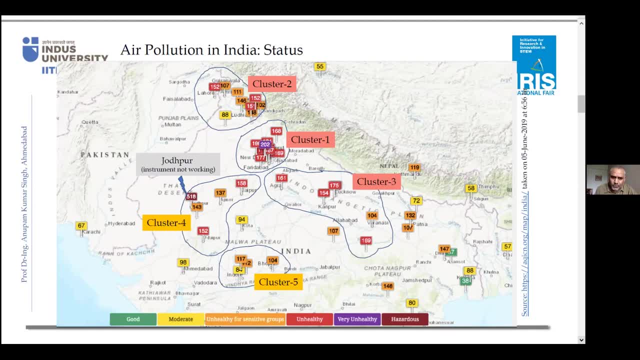 Then we have a fourth cluster, which is Rajasthan cluster. like Jaipur, you know Ajmer and like Pahid. And then we have another cluster, you know, which we call it Gujarat cluster. you know where? Ahmedabad, Baroda, you know Bhopal, Indore, kind of. 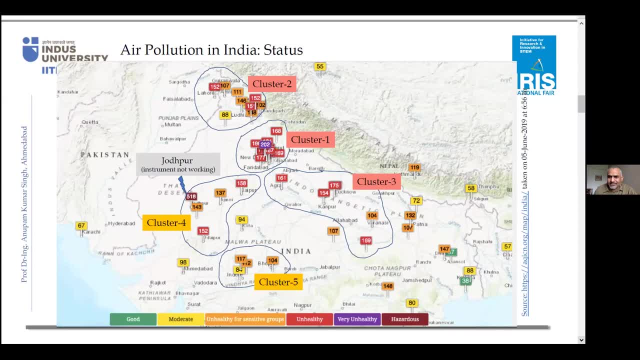 And then again there are clusters. Okay, So, yeah, Okay, So, just as a demonstration, you know, took this example so that it is possible to see that you know how we can classify this air pollution in various areas or in various cities. 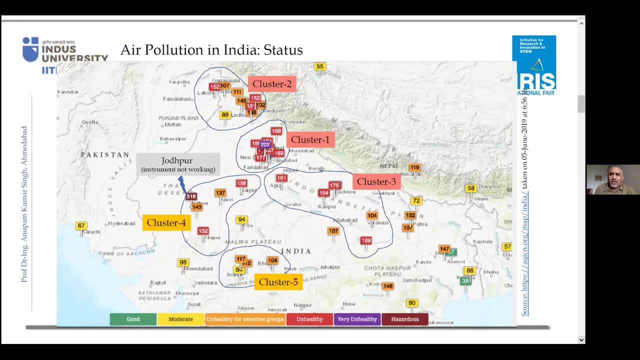 And then what kind of technologies which, essentially, are required in order to sustain our livelihood And those who are living in NCR. they can very much understand that. you know the air pollution is very important. They can very well, you know, comprehend and you know, can also tell that there are you. 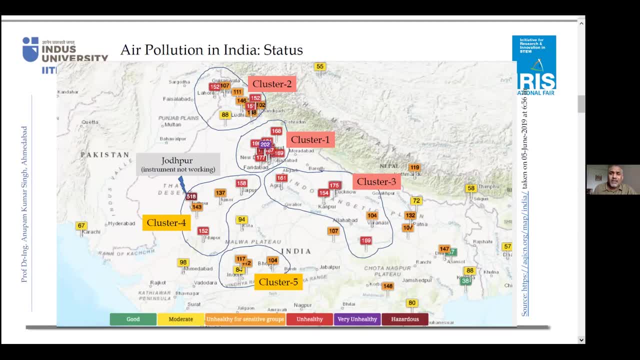 know days or even weeks, you know when we have a difficulty in breathing. Now, if somebody has a difficulty in breathing and you know these air pollutants are bigger one, you know they normally go into lungs and health system and then therefore, you 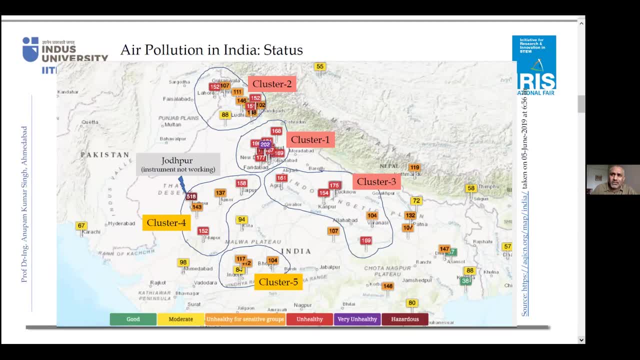 know, create one or other illness. you know, either in terms of asthma or in terms of other, you know. So there is a very good understanding. There is a very strong, actually, relationship between air pollution and human health And therefore, at city level, at cluster level, you know what kind of things are required. 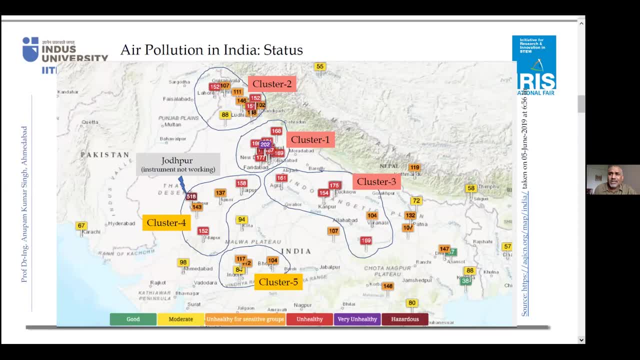 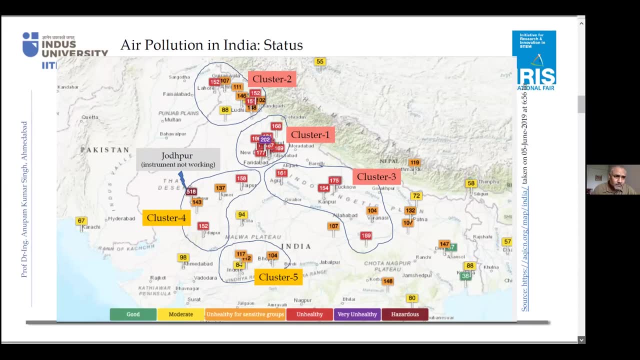 what kind of technology are essentially required. You know we can think for those and then we can, you know, develop them. Next one, please, Again, when we see the air pollution cases and experiences, you know we can see that. 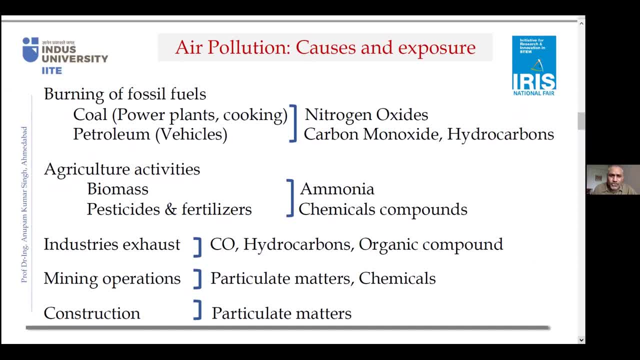 you know, there are a lot of things that are happening. There are a lot of things that are happening. There are a lot of cases and exposure. I will not go much into this one, but this is there actually And the idea here is that, you know, because of agricultural activities, as I mentioned, 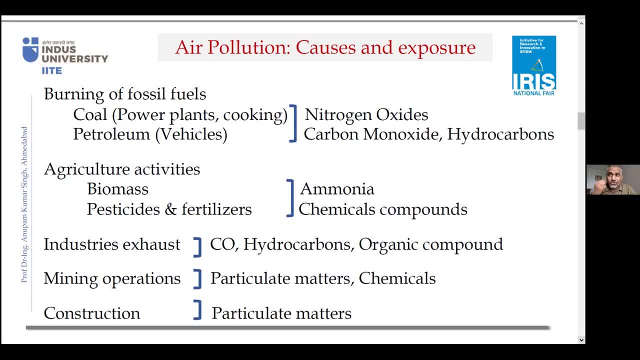 especially, you know when we are burning this biomass in Punjab and you know in Haryana or in parts of UP. you know this air comes to Delhi. you know because Delhi is a big city. The temperature is low. 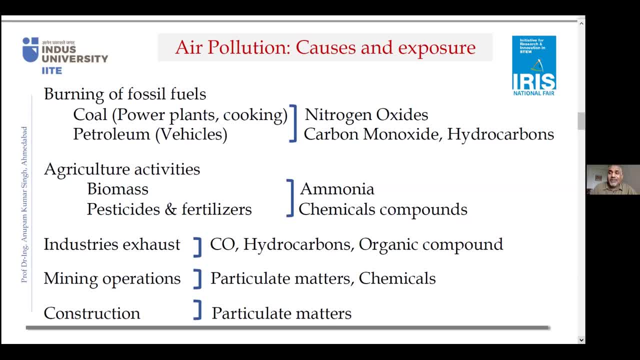 And once temperature is sorry, temperature is high. and when temperature is high it creates low pressure. And when low pressure is there, you know that the air moves from high pressure area to the low pressure area And therefore, you know all air you know which is in the surrounding area comes to. 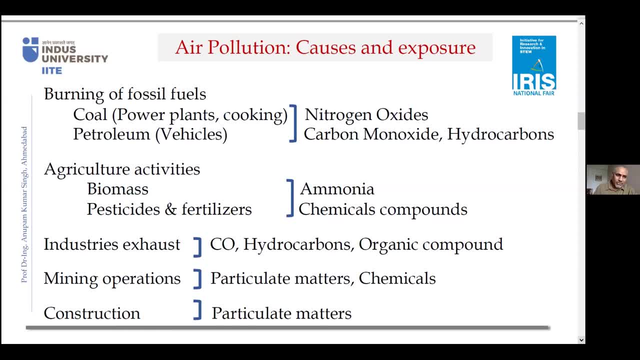 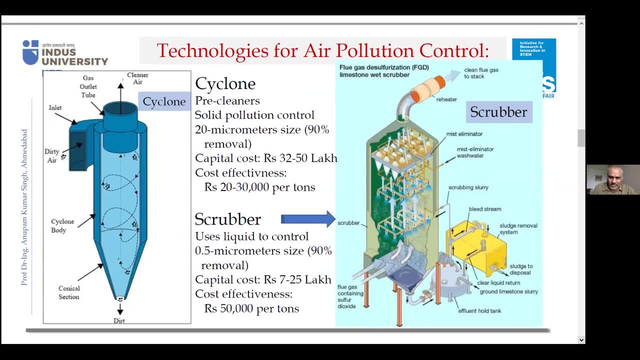 actually Delhi. Yeah, So that is one reason which I can actually give you. the next one, please. yeah, So there are some technologies for air pollution control And these technologies are, you know, one could make a small, for example, cyclone. 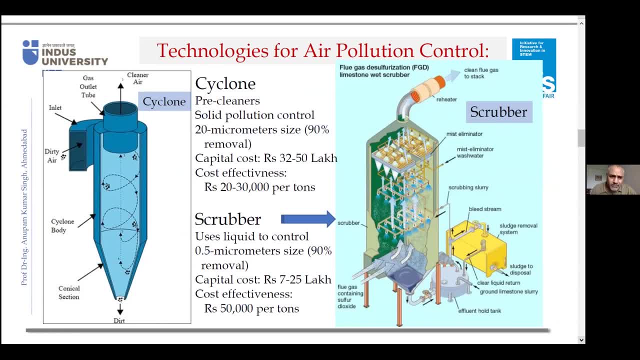 So you see that cyclone is a very simple system, yeah, where left hand side, you have a dirty air which is entering into this cyclotron, yeah, And this air moves, so called, into one direction. And once this air moves, then what happens? these small, small particles which are there. 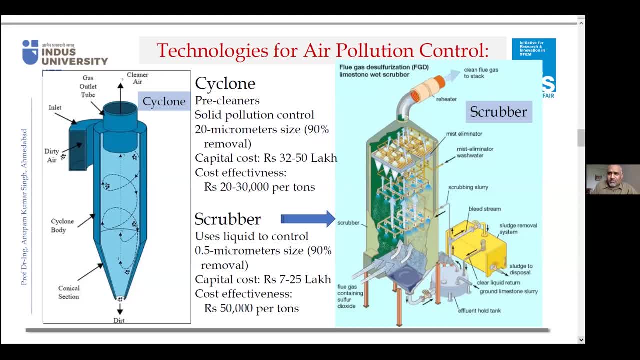 you know, You know, through a collision process, colloidal process, actually, they become bigger one, And since they are bigger one, they are heavy. And once they are heavy, then they precipitate down in the form of dirt. yeah, 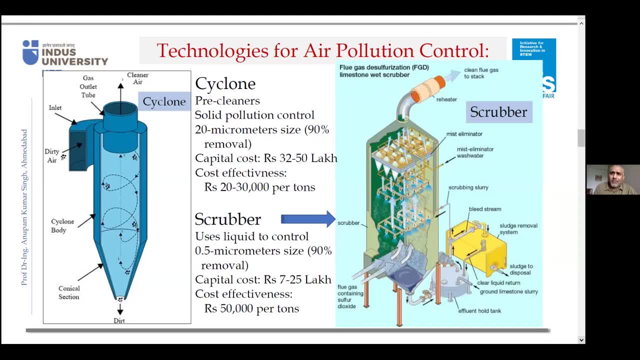 So therefore, in this cyclotron, the separation process actually of the dirty air and the deposition of semi-solids or solids, actually It takes place in the clean air which is normally now lighter air, you know, goes in. 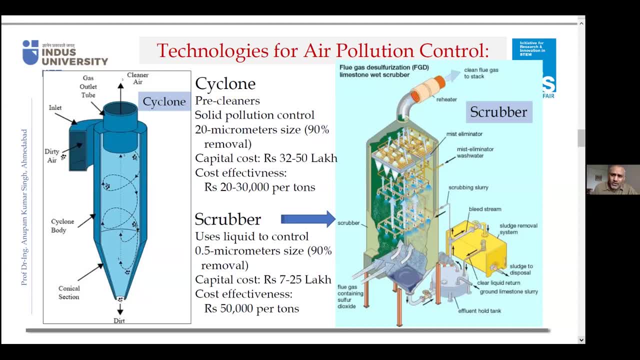 the atmosphere. Yeah, So this is one process. Now there is a possibility to actually improve the design of this cyclotron, because normally this is a simple, you know funnel kind of a thing. yeah, But I think if there's a possibility to so-called devise, you know, a new cyclotron based on 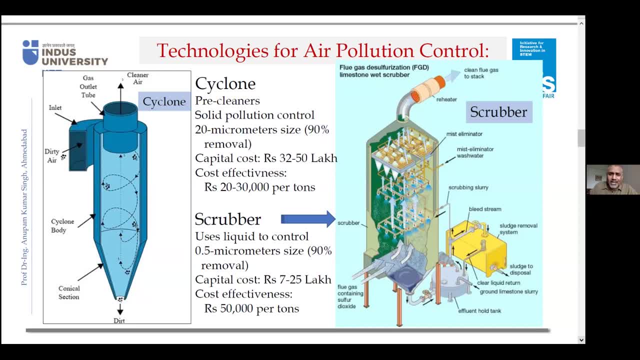 the principle of fluid dynamics- We call it Yeah- And therefore it is possible to remove even these. You see, here I wrote that the solid pollution control. this particle size is approximately 20 micrometers in size And this removes approximately 90%. 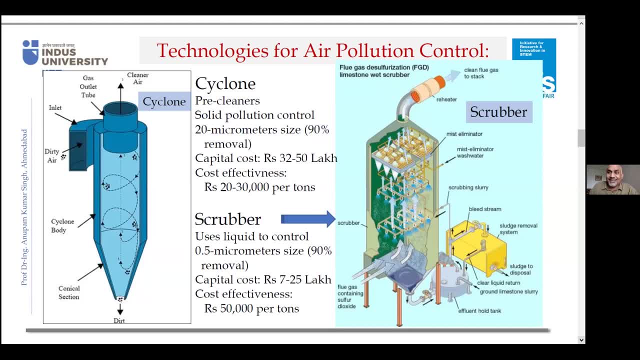 Now, 10% is still good in the year. Now, whether it is possible to improve the so-called efficiency: Yeah, From 90%, say, maybe 95%, yeah, then we can win a lot of cost actually, yeah, and also. 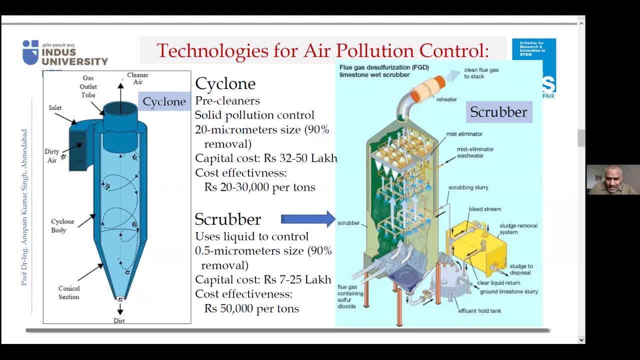 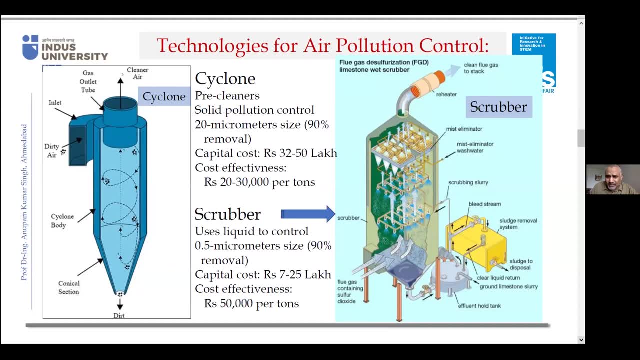 the cost in terms of air quality? yeah, Another example I'm giving you is shrubber. So what is happening that the mist actually here in this particular experiment, what we do is that we are bombarding the mist, actually in the form of droplets. yeah, and these droplets? 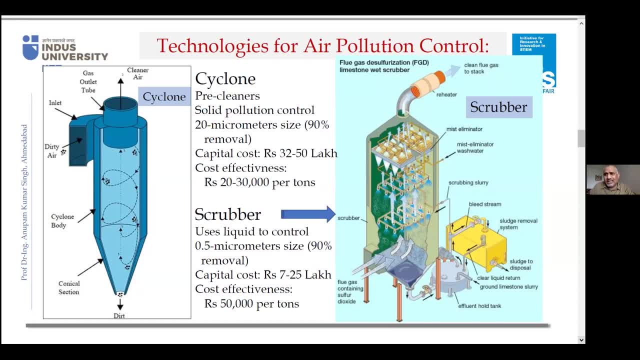 are really tiny droplets. Yeah, And these droplets together with so-called this, you know, air, which is again with the suspended solids, yeah, and so they together come and they form a bigger droplet and therefore, 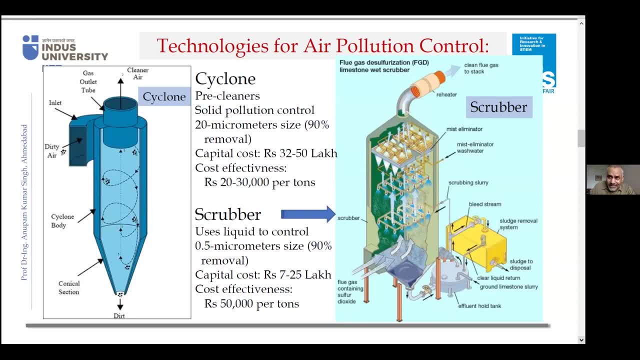 they fail down, And that's why students can see that when there is a rainy season, our sky is much cleaner than the sky during the summertime. Yeah, So this is the reason, and therefore we have the shrubber kind of thing. you know which? 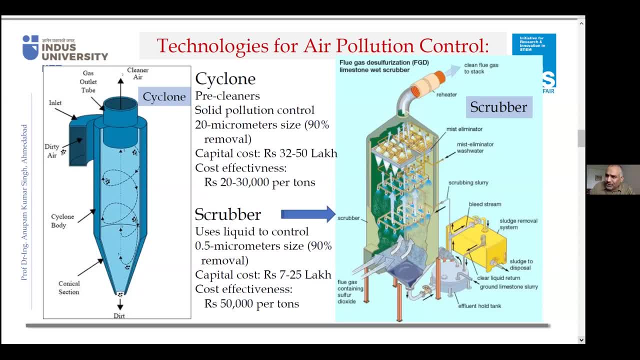 is very often used, even, for example, in Delhi Metro. they use actually so-called this shrubber technology for cleaning the railway wagon- yeah, or you know this? metro wagons- yeah. So such things are again available. 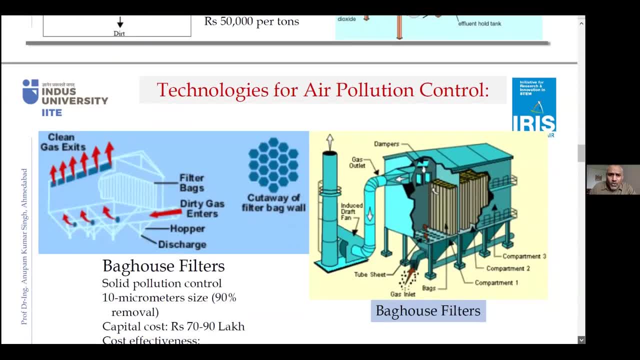 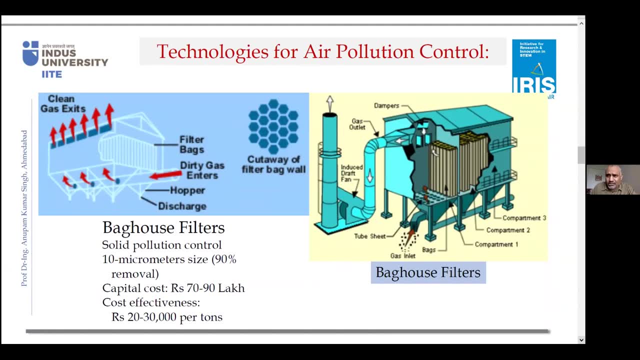 Next one, please. Now, another technology is actually- we call it bag house. So this is very similar actually to technology which is, I already told you. you know, this is very similar to cyclone kind of a technology. you know, again, there we have different compartments. 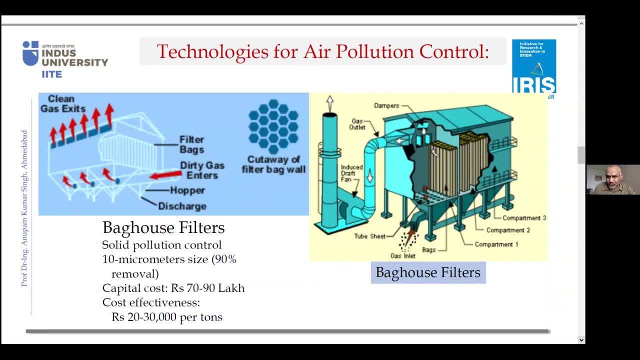 and then we have a medium. So medium means filter, medium. So, for example, if you see you have a tea and when we have a filter, actually we can, you know, put filter and pour actually the tea. 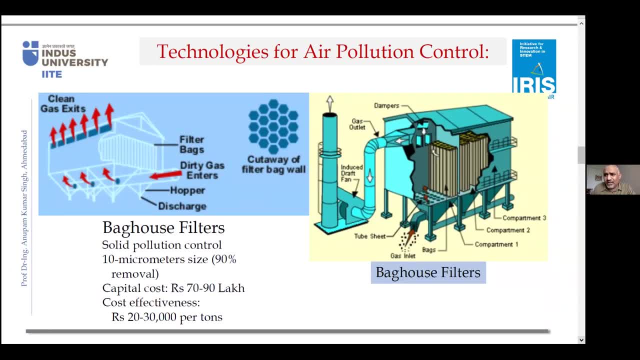 Yeah, Yeah, Yeah, And we can pour tea into that filter. and particles which are bigger than the filter size are often collected in those smaller particle size. they are actually when normally through the sea. So what we can do is that, in order to increase the efficiency of collection, we have to minimize. 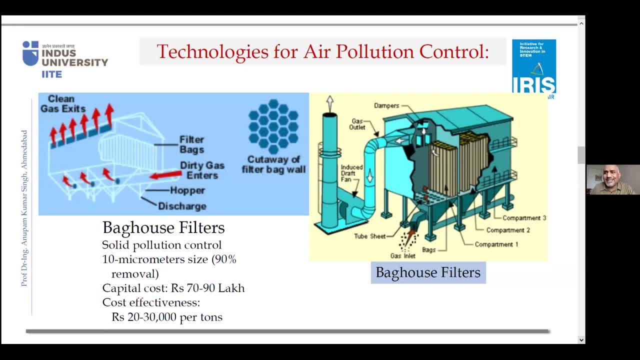 the size of the force of the sea. Now, if we have to minimize this size, is what will happen? actually, the efficiency, the, the volume of actually goes down, because if the, the flow which is supposed to happen through these open- yeah, i mean forced- the force size is. 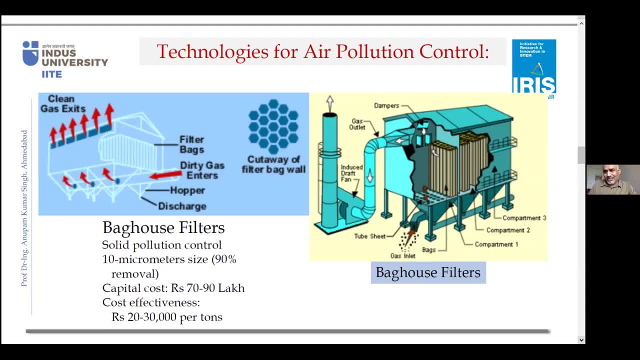 decreasing, then flow actually is decreasing, yeah, its force size is decreasing, the flow is decreasing and therefore the possibly the efficiency of you know such normally things goes, you know, down, yeah, so therefore we have this technology again. if you see that the removal efficiency of this technology is again very close to 90, now can we do something, because these devices are having huge cost? 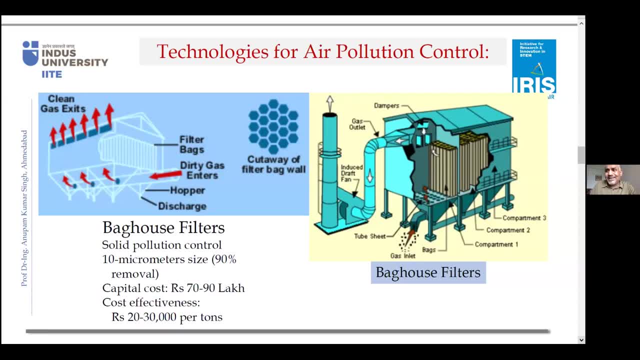 in terms of you know, and they have a huge volume because each and every industry now is per the state solution control boards. i am from gujarat, so we have a gujarat pollution control board. those who are from rajasthan: we have a rajasthan pollution control board. 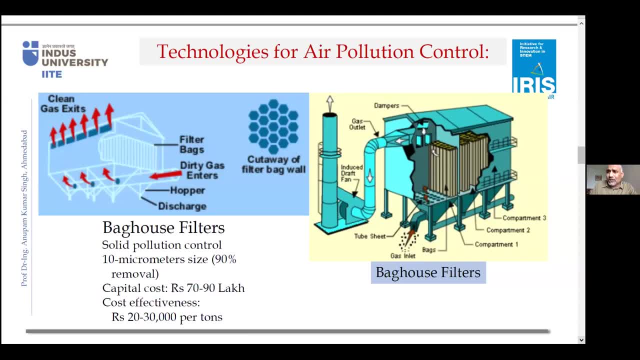 pollution control board and then we also have a central pollution control board. so what happens that these people- you know, they make sure that you know- these certain standards are very well met in order to actually work with, yeah, these devices, one can have a multiple filteration, which is real. 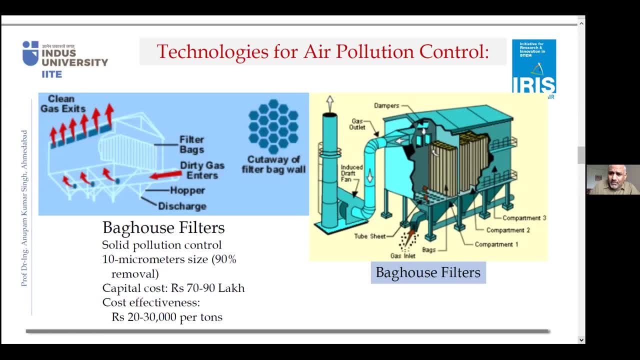 So I think the possibility that one can do something here in terms of these air pollution control technology. I thought that I will try to bring you one important sketch here, And this sketch is a typical problem that majority of us are facing at a thermal power plant. 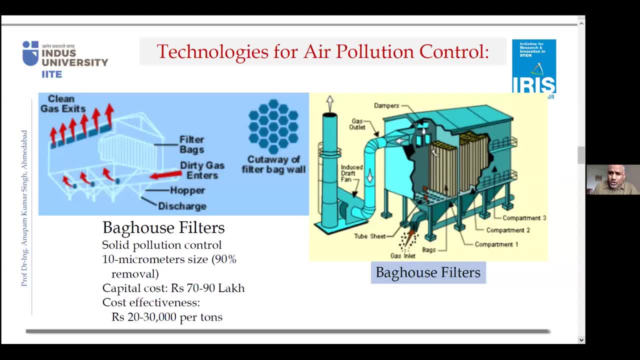 So this is a typical thermal power plant where coal is being crushed and also then fed into the boiler, The water is being circulated actually in the boiler and we heat that water, we make steam. Now that steam rotates actually the turbine and turbine rotates the generator. 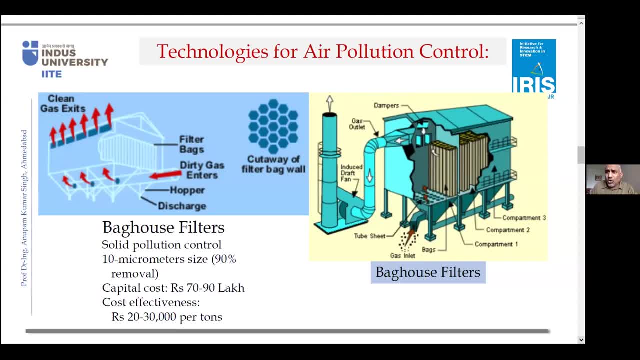 and therefore we convert actually so-called this coal energy into actually the electrical energy and then, through a transformer, we supply this to the grid. Now, if we see here in this particular process, it's we are very much aware that these thermal power plant produce. 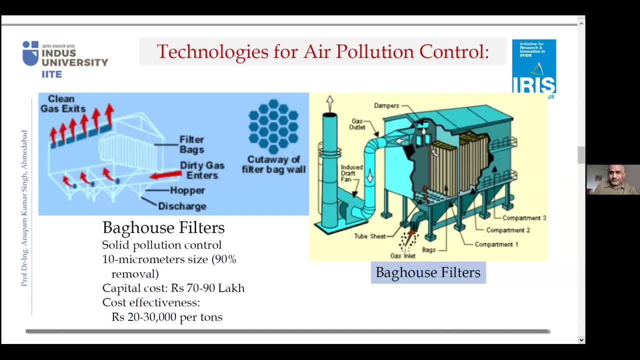 a lot of energy, A lot of, actually, air pollution. So is it possible to do something? is an integrated project actually for these thermal power plants? So, for example, what is happening? that when we are boiling the water, because water is being generated into steam, 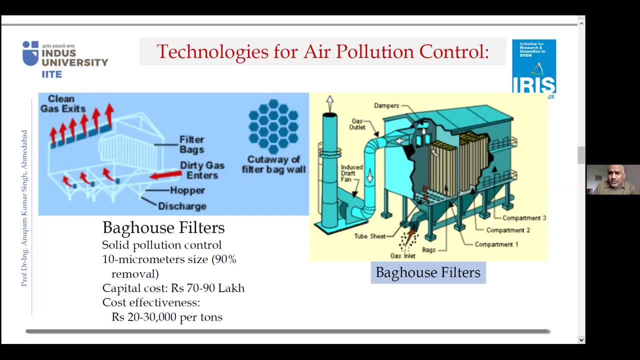 in that steam is being so called actually recirculated. yeah, Through the cooling top, cooling tower. so we have a cooling water. so this means a hot water need to be once again, you know, cooled, and then again it has to be actually supplied because the condensers are there. yeah, 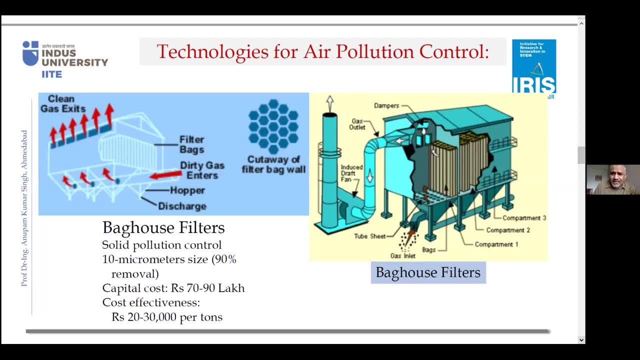 so what is happening actually? if you see typically such thermal power plants, the efficiency is normally low. i mean it was as low as 40 percent, which in the years has improved actually, and because and goes as high as two-thirds, you know this means around 65 to 70 percent, like that. yeah. 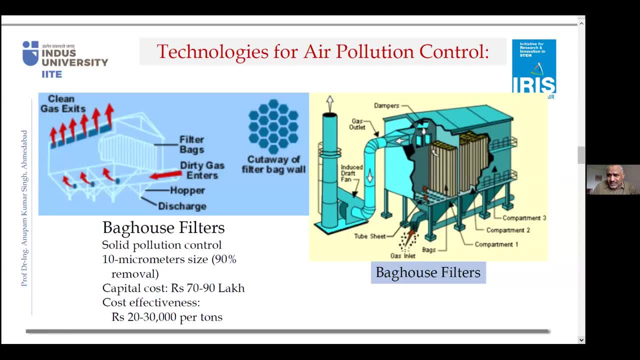 so there is a possibility that this steam, yeah, which is at, let's say, 110 degree, you know 120 degree centigrade, we can convert. actually, you know this steam because the delta is very high here, because normal general water, i mean the normal water, has a temperature approximately 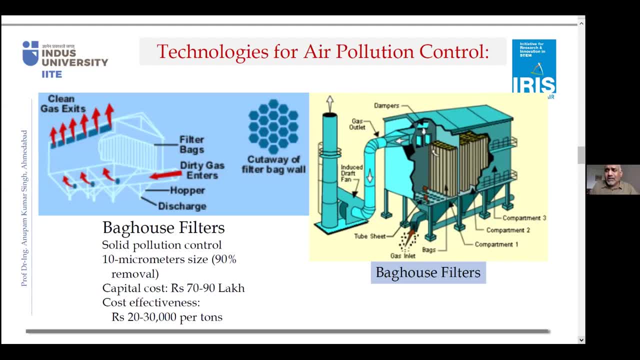 24 degree to, let's say, 30 degree here in india. so if your steam is at 110 degree, the gradient is approximately 70- 80 degree. yeah, so this 80 degree gradient can be very well utilized, actually for the purpose of so-called we call heat recovery, so we can use this heat that. 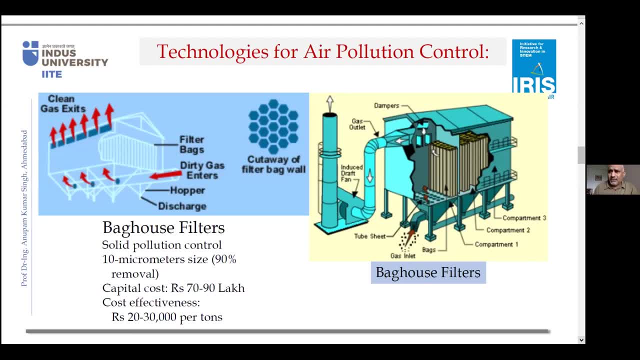 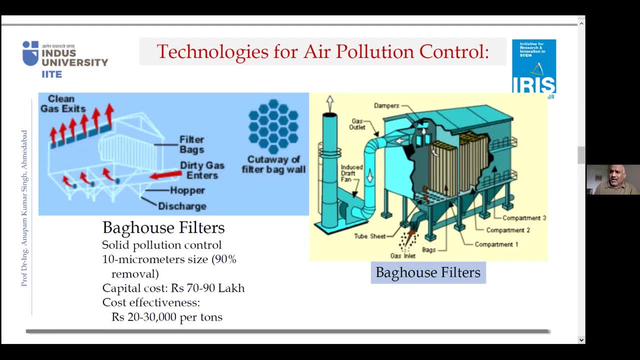 centrally heating system. yeah, in india also, actually, right now, you know, we have those inverter- we call them refrigerators now, systems which are there, you know. so there's a possibility to use this heat actually for some purpose and therefore i will, you know, suggest that there are some projects can be developed in that area. then again, uh, actually what i'm? 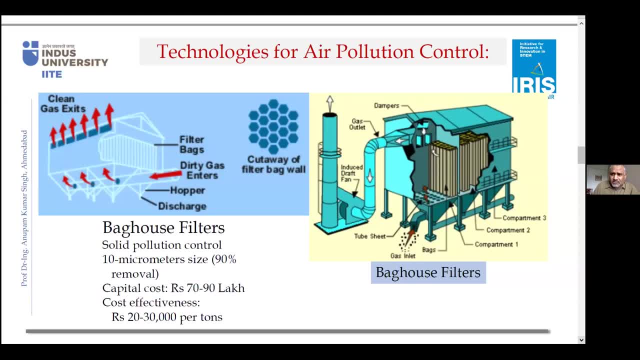 going to show you is that, as a, my heat sufficiently is broken, so that, uh, thishil 이야기 aïcha. well, in this context, there are reforms or changes to be made in production in either six zones to operate or only in the winter plums to operate, рублей, isage, Ziemiya and. 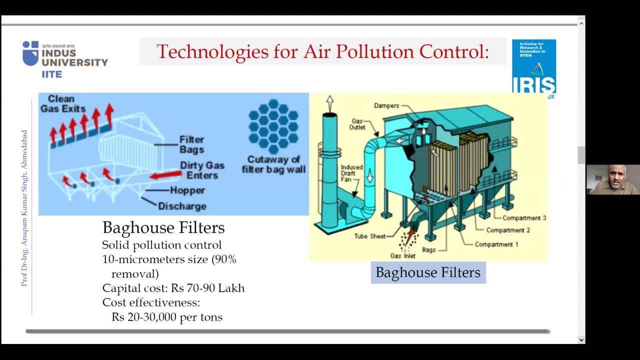 this will be an interesting priority for production. so the first point on this, but not also its safety, because if you, if you recall, in india- yeah, leaders, these- we watch the evolution of global changing teams and so the nations of the region that for the last two years they changed theirнопveli. 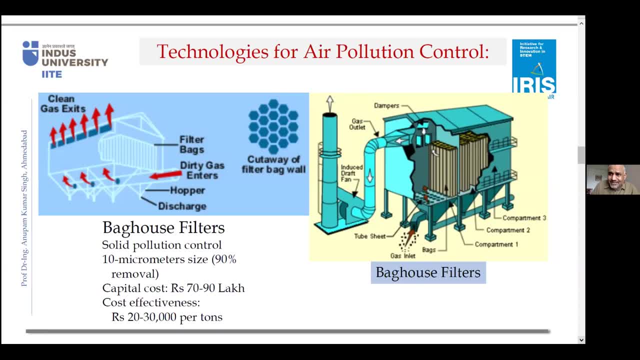 catalytic reduction of nitrous oxide gases. there's a possibility actually to redesign even. you know such devices or filters, you know, let's name them filter, you know. so such filters can be very easily actually one can devise them, yeah, or one can think in in terms: 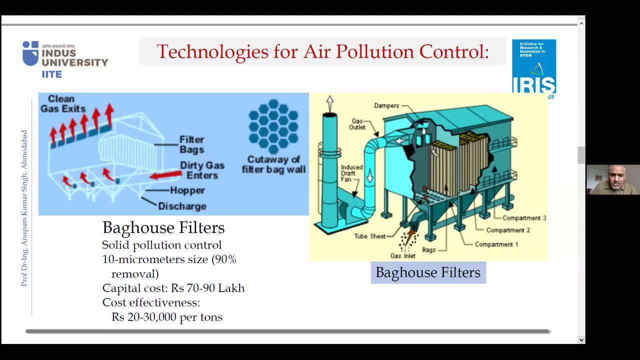 of devising. then we have these particulate matters, so we call them esp. this means electrostatic precipitators. yeah, so also there is a possibility that one can increase the efficiency, because the precipitator efficiency right now is around 98 percent. 99 percent, yeah, and several i have. 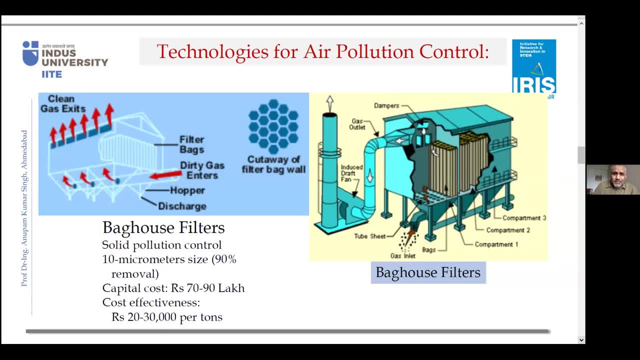 visited several uh cement plants. the precipitator efficiency in cement plants it's not more than at this juncture, above 90. so even in cement plants there is a huge scope actually in order to actually bin the collection- so-called- of these particulate matters. and then we have 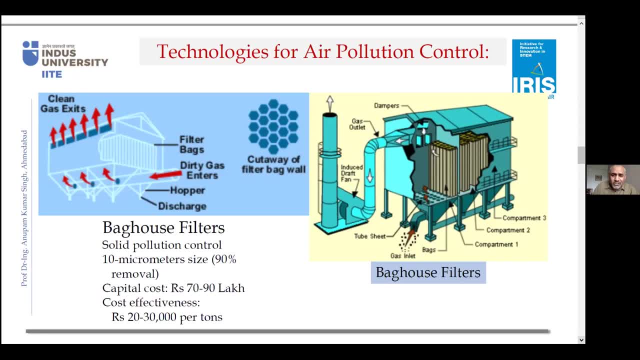 this fgd, which also reduces the sulfur oxide. so because flue gas desulphurification, sulfurization, so this flue gas desulphurization also there is a possibility, because the efficiency of, you know, this particular process is around 90 percent. yeah, and then of course we have 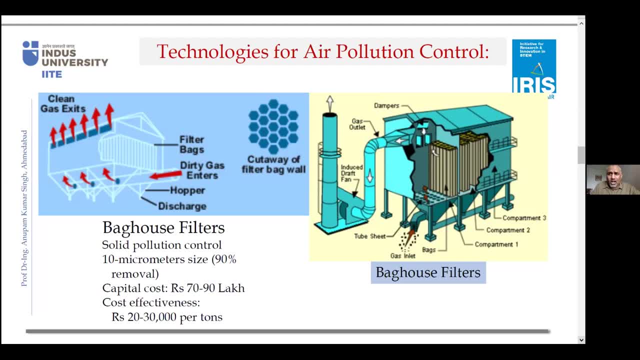 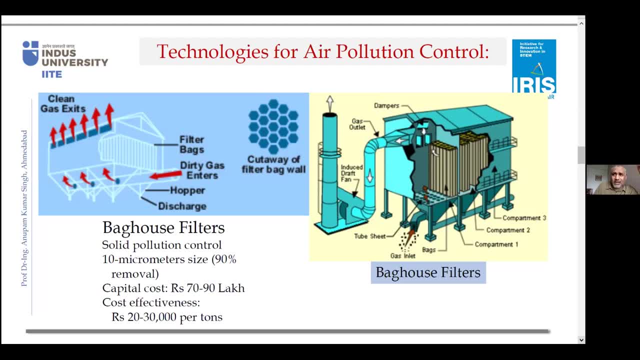 high, you know so. then we leave actually this particular gas in the atmosphere and, you know, through certain processes, you know, around 100 kilometers, sometimes 200 kilometers, sometimes 300 kilometer. later, actually this gas is so called being settled actually on the ground. you know so. therefore we have to, although there are monitoring mechanism every year, so people like 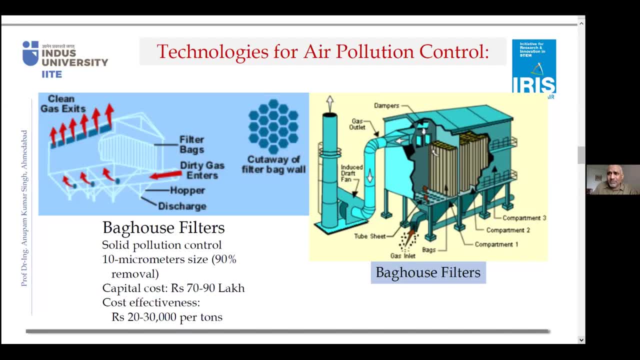 like me who are experts in this area. so we budget, you know, such uh monitoring, uh emission, monitoring, uh stakes, and we monitor each year and we also give a certification due to those companies. but still what? i feel that actually there is a possibility actually for all of us. 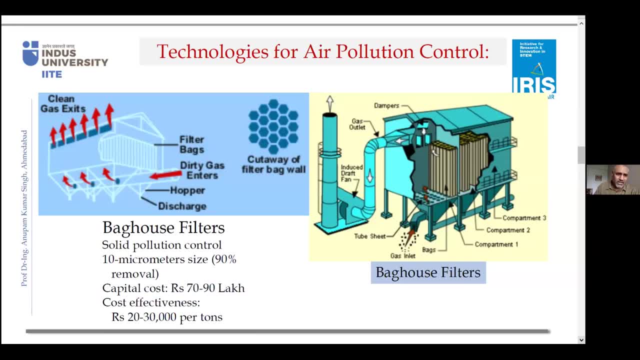 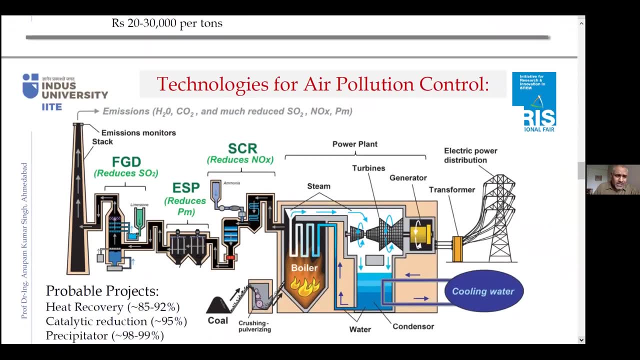 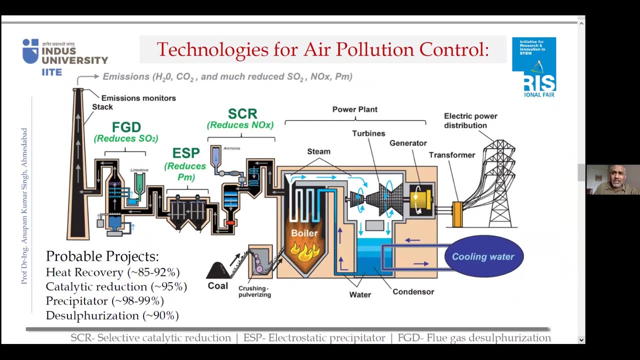 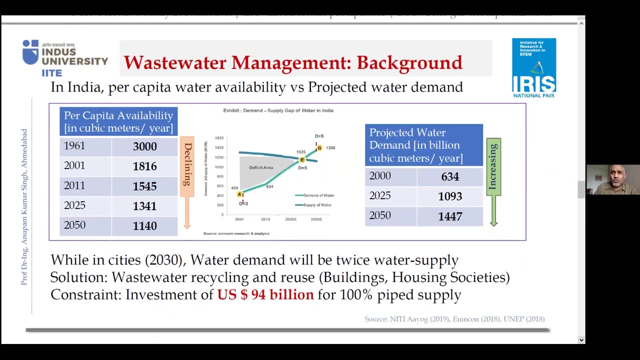 to do something very interesting and nice actually in this particular area. next one, please. yeah, my next talk is more into base water and i would like to show you that why this water is important for us. so when we say base water, this means best water is based, so therefore it has to. 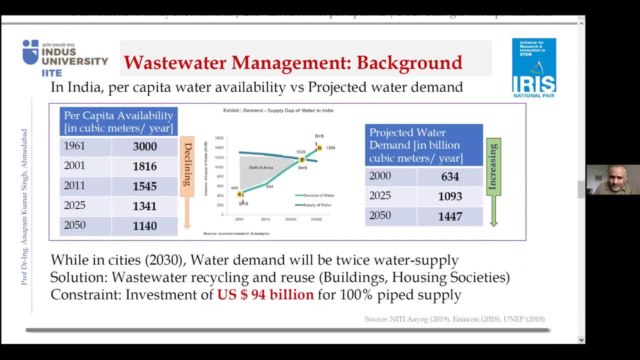 be thrown out. now i try to bring one figure here. so if you see, in the middle, uh, there is a chart, yeah and uh, which on the y-axis shows the demand, water demand and water supply, and on x-axis, in the middle, it shows the timeline time axis. so it starts somewhere, let's say 2000, 1990, 2001, and goes on to 2050.. 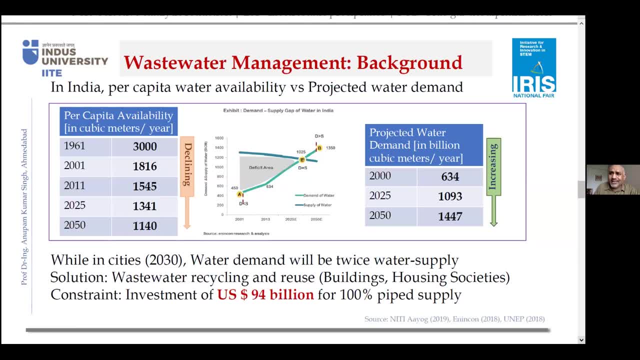 so niti ayog has prepared recently a report last year into. recently means last year, 2019, and they have given a particular data as well in this kind of evil: that per capita water availability and projected water demand. so when we say projected means this, is it has been so called assessed or estimated. 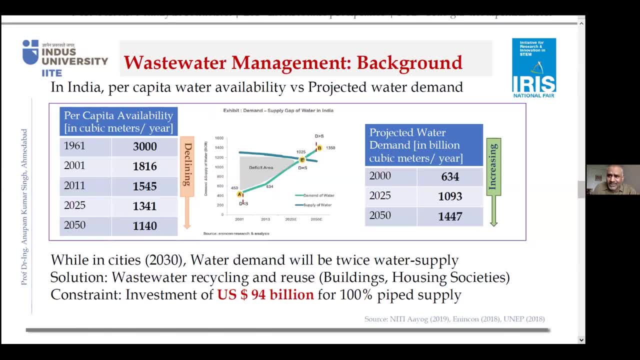 for the future. so this means, if we know something in 2020, is the actual availability or actual demand will happen in 2030, 2040, 2050.. So we use certain mathematics, we use certain interpolation techniques and, based on those interpolation techniques, 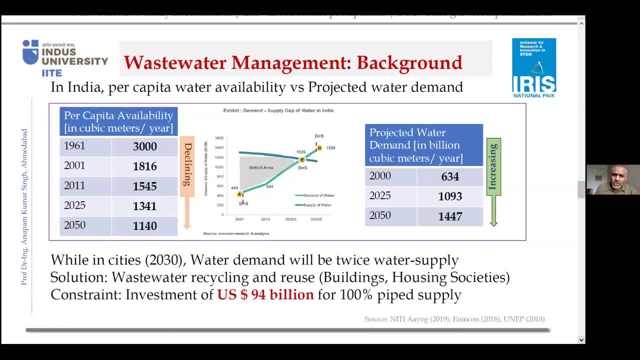 we project for future And so therefore, some of these figures beyond 2011 and 2016 are actually for the projected one. So if you see here, so I will like to request you to look left hand side, which talks about per capita availability. 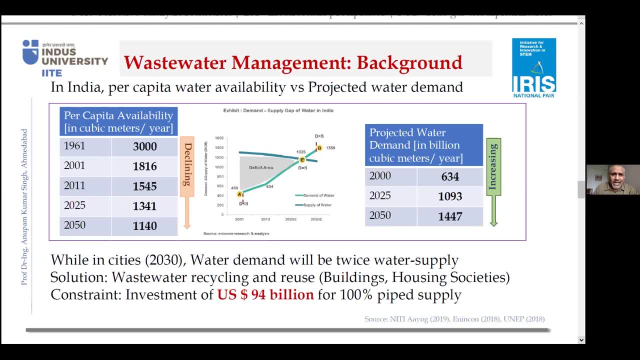 Now, per capita availability is a function here of number of people. per capita means number of people. Now you know that the population in India is increasing. therefore, if X amount is there, then per capita is the number of people. If X amount is there and if number of people are more. 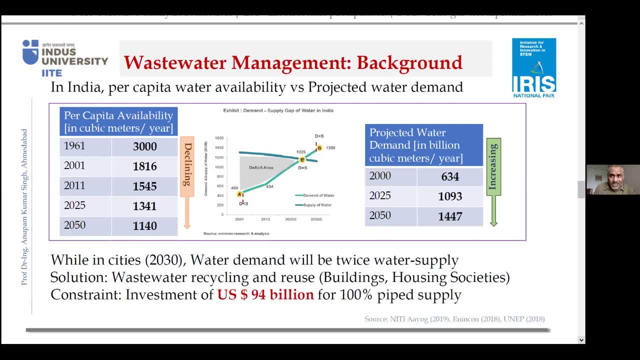 then availability decreases. okay, So also what is happening? that recently you must have seen that in India actually the rainfall is going down. Now the amount of rain in a given area is going down. This means per capita availability will decrease. So population is increasing. 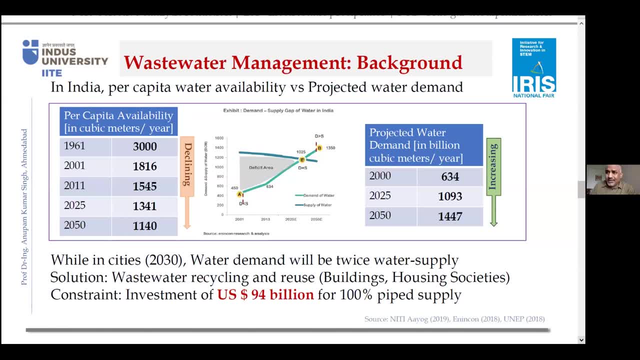 amount of water is supposed to come through rain. amount of water is supposed to come through rain. amount of water is supposed to come through rain is decreasing. therefore, per capita ability will decrease quickly, right? so the projection for 2025, in 2050, is 1341 and 1140 cubic meter per year. now they have also made a projection, if you see. 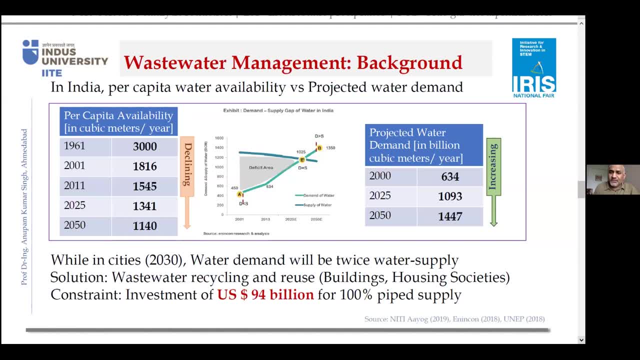 projection for 2025 and projection for 2050 says that the projected water demand will be 1093 and 25, but 1447 in 2050. this means what is happening: projected water demand is increasing and per capita availability is decreasing, and in the middle. this shows that 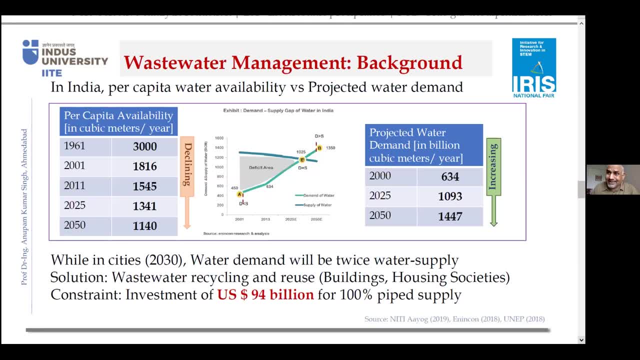 approximately at 2025, which is point e, where demand and supply. this means availability and demand will be same, and that may come very close to 2032.. now, in 2032, if my income is same, then my expenditures i am going to be in a big trouble. okay, so we need to win new work. 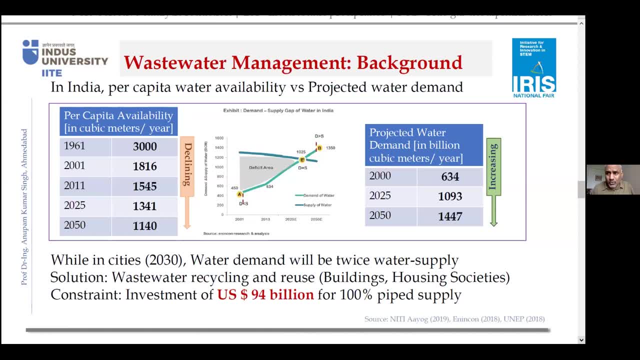 so the purpose of this is that new water. now, if you see, in our cities currently, the people living in cities will be almost two times because number of cities will increase. also people who are coming to cities. they are increasing. there's no harm in coming to city. 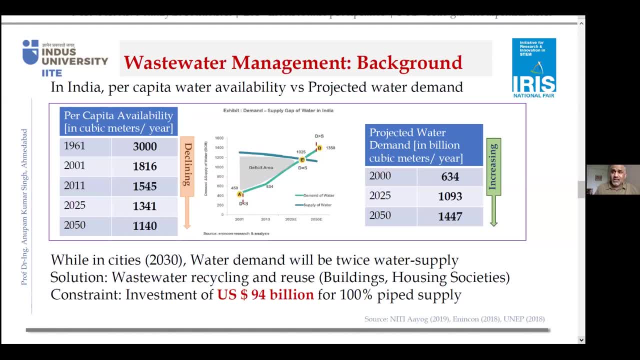 because cities are good centers for education, they are good centers for job, yeah, they are also nice centers. so everybody wanted to come to city because of these inherent regions, and one cannot stop anybody in like- unlike china- so therefore we have to prepare our cities well as well. so therefore, the solution actually lies right now in terms of based water recycling. 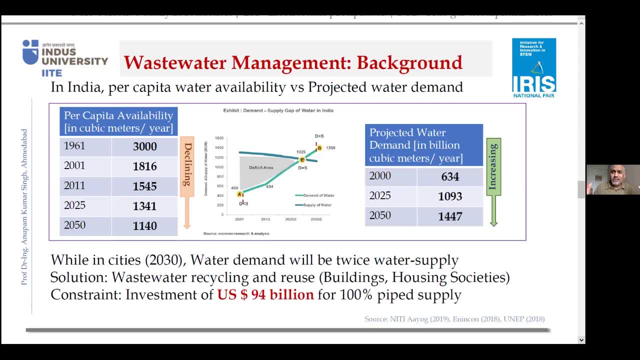 in reuse. so this means base water, which we used to throw out. now it's no more a based water, but it is actually a boom now. yeah, so we can use that. yeah, and then we can so-called reuse that, and the work is happening at building level. it's also happening at so housing society's level. 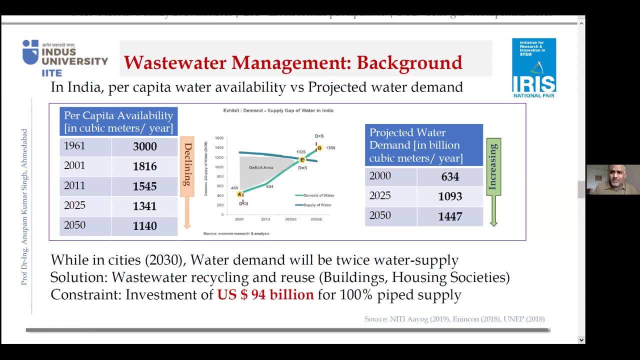 yeah, and where even the cities i'm from in the water in india, because the water availability is less, yeah, and water demand is very high. therefore, we started very much actually treating and using these technologies, but it requires money, so money is the constraint. actually, that's what i'm trying to write here. 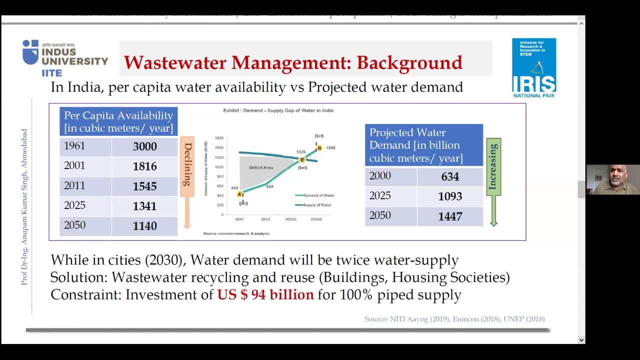 yeah, so there is a possibility to look some of the so-called new projects into this area. i thought that i will give you a little bit further. you know what is happening, that if you see in our cities- you know small cities- there is no wastewater treatment plant, even in delhi, for 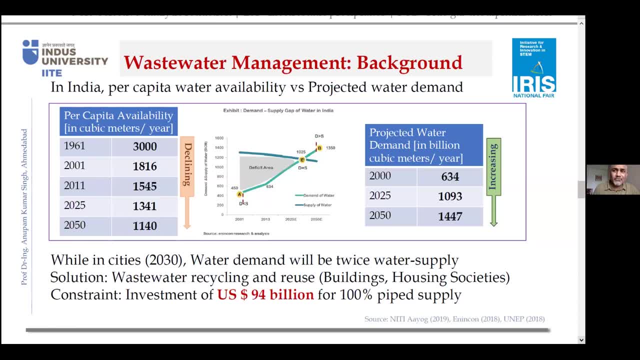 example, you know, right now they are just able to treat not more than 50 of their total capacity. 50 of their total capacity, and that's what in delhi is actually being so called flown in um, in our uh river. so i mean again, if such a problem is with a big city like delhi, what about the small towns? 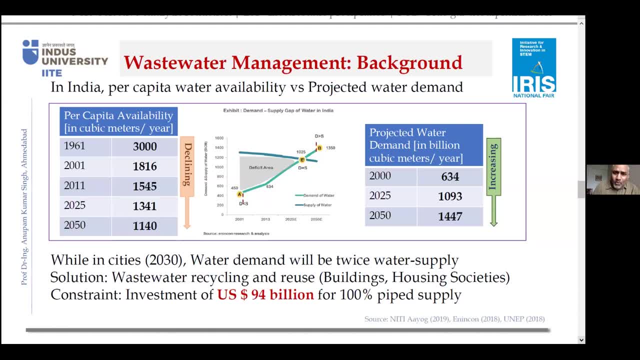 who do not have capability actually to work with india. so therefore there's a huge scope and i wanted to say here: so please look this uh graph, you know, which talks about technology, ecology, economy. i put this actually a graph for your understanding, because it's not only technology is important. 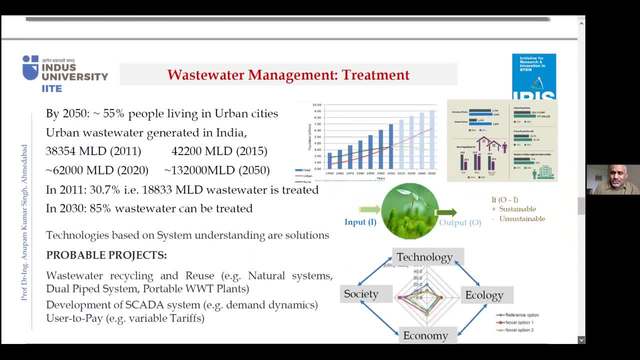 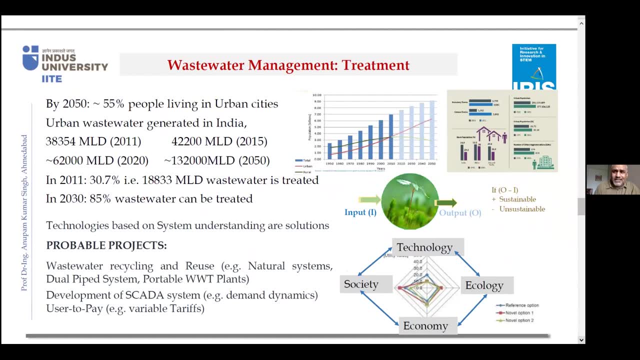 it's equally important for us is that the society you know which will be using this technology. so the technology has to be developed in such a way so that society finds is useful, so that it is actually saving our economy. so this means it's a cheaper cost and also it balances the ecology. ecology means here environment and complete i'm. 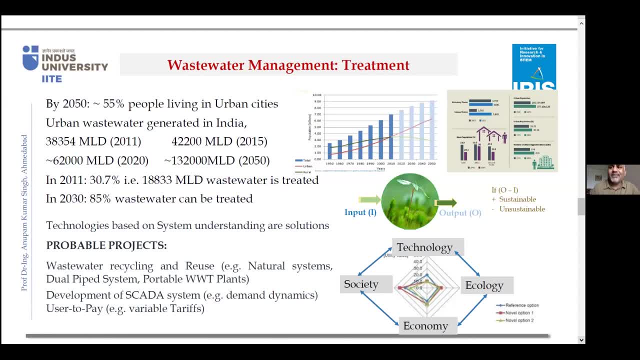 talking about complete ecosystem where we all live. yeah, so we live, humans live, animals live- yeah, plants live like that, yeah. so therefore, a balance is actually needed here, and therefore sustainability can be achieved only when we look into our past and say that the future is in the life of those things, and that's the bottom line. 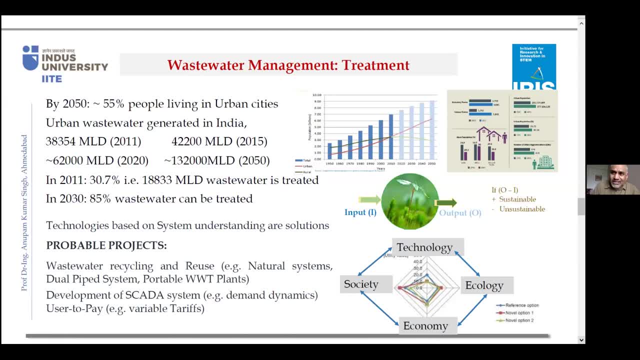 because if that doesn't happen, then we can't go forward up the mountain. so we need kind of sort of a natural or natural way to handle that in our future. so that's why you should look into those four parameters, so for you to justify your project into the area of wastewater treatment. 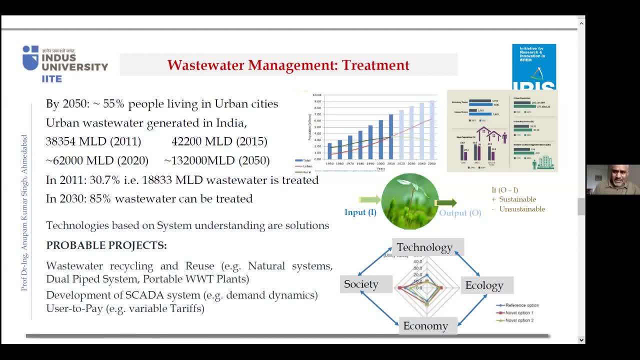 technology. i think you please look into these four dimensions. do not look. technology alone was not sufficient, but nevertheless, I think you can read that and we can discuss. So I try to list out some of the projects for you here, and one project which is actually is on wastewater recycling. 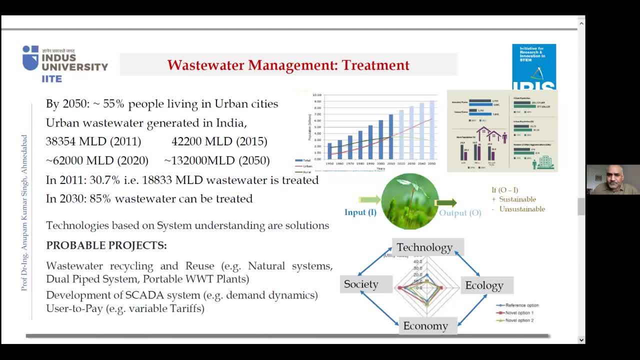 and reuse. Now, when we talk about this wastewater recycling, recycling means we are again, you know, bringing actually this wastewater to the standard you know, which is important either by. World Health Organization has given certain water quality standards. also, government of India has given certain standards. yeah, we call central public health engineering organization, so that has. 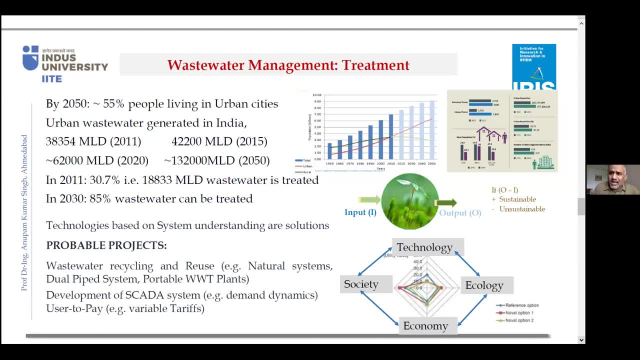 has given some standards, so those standards also can be compared actually. but we have to see that these systems are much more natural systems. this means they consider nature actually, so called for their treatment. also, what is happening? that in Ahmedabad? you know the society in which I am living. 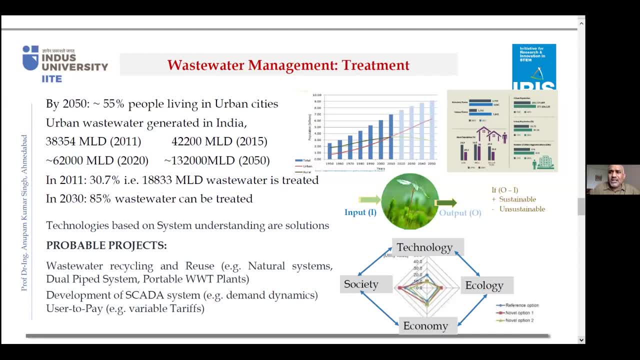 we have a dual pipe system. so this means especially for bathing, cooking and other users, we use actually the fresh water, while for flushing we use actually the treated water. so this means we treat that water and we recycle and reuse actually into the flushing system. yeah, so such things are very much possible. and also what is happening now. 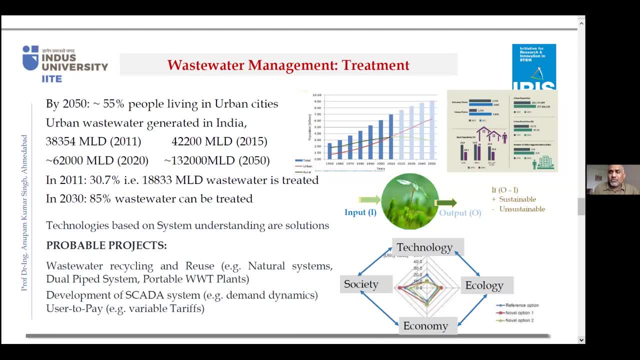 is that people started talking about portable wastewater treatment plants. so, for example, if I am having a single bungalow, yeah, then I can install a portable wastewater treatment plant and then I can use the water actually mainly for gardening or for any other purpose, rather than throwing that into the drain. yeah, so such things are very much possible. and also recently, government 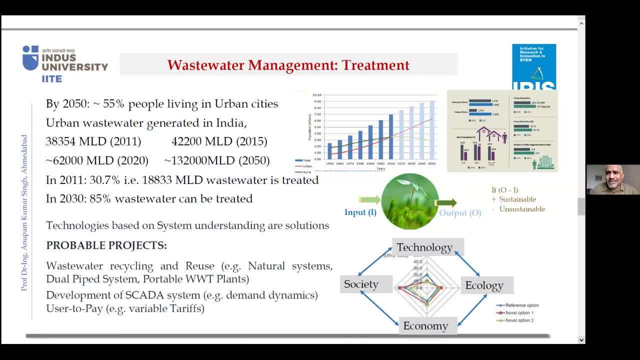 of India, through center for science and environment, has given guidelines that each, for example, institution, like university, must have a water treatment plant, a base water treatment plant, and they must have a liquid discharge plant. this means you cannot throw actually liquid out and you have to reuse it next, which is possible because when we will have this dual pipe system. 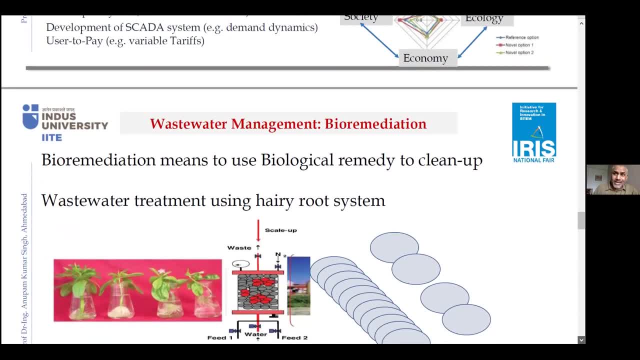 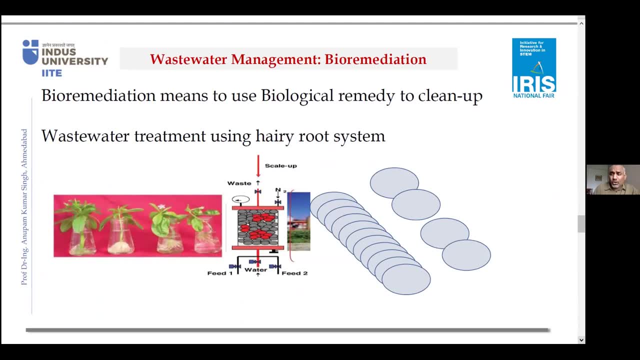 at building level and also, let's say, perhaps maybe later stage, at a society level or a city level, then we require a supervisory control system like algorithm based systems. you can so called close open or close-laze. close-laze, which area can be given first? 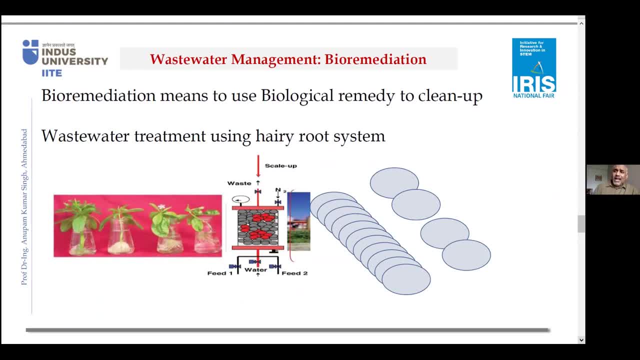 which area can be given later so we can have a demand dynamics and based on that demand dynamics some system can be laid. so therefore you can also look into project you know where, if you can write a good so-called code actually in computer. we used to, I used to do, actually I used to do- research. 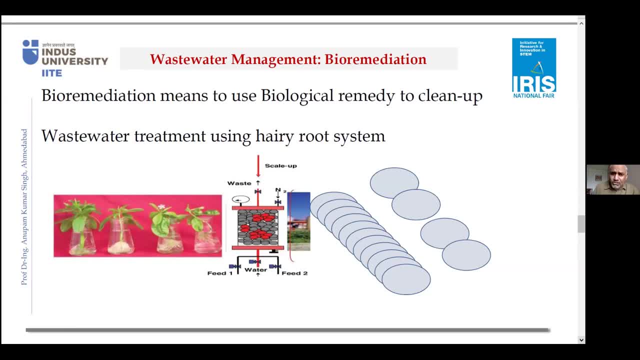 and today also my PhD students are doing that. so you can also code actually a system and then you know you can have those systems and which is again a newness actually, in those coding could be there and then user to-pay, so some sort of a system. when you have this SCADA system. 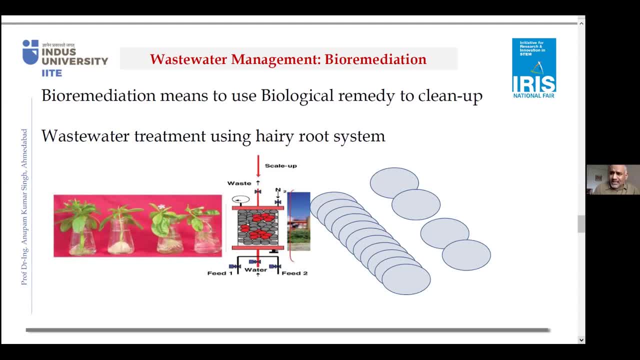 then you can have variable tariffs. For example, in Delhi, the Delhi government has said that if somebody is using less than 20,000 liters per month, he need not to pay even a single money. So such kind of systems are very much possible. when can be regulated? you know, when we have this kind? 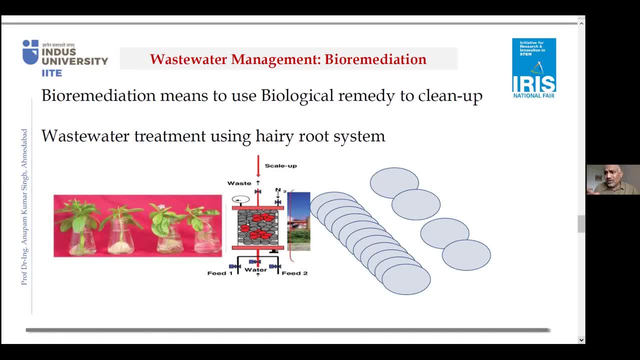 of a system. Yeah, So it's like a joint computer civil system. So a lot of actually so-called computer knowledge is coming into civil engineering And this can be done only by a civil engineer, because many times computer people do not understand. you know what is. 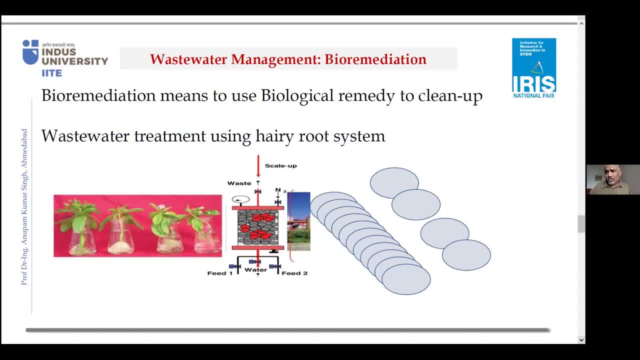 the SCADA system and what is the network and how losses are happening, and you know how to calculate head and things like that. you know. So even those who are intending to go for a higher studies. I think the intervention of computer is coming in each and every area. 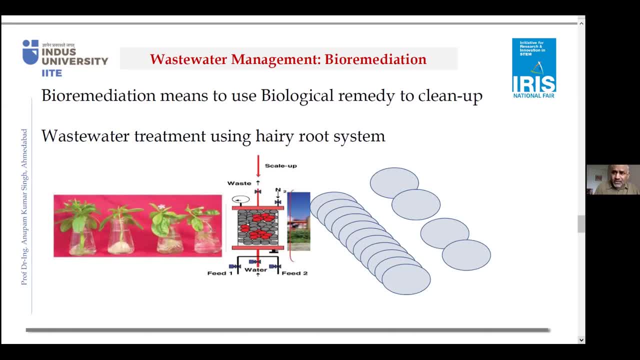 And therefore there is a possibility to do something based on that, especially for your city government. Yeah, So that could be also one of the interesting project, even for our IS. Again, wastewater management, bioremediation is happening. So what is happening in bioremediation? 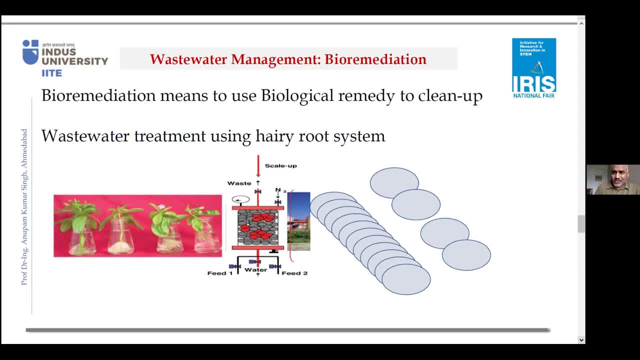 that we are finding actually biological solutions. So this means we are taking plants, for example, putting plants in the wastewater and the these plants are somehow, you know, cleaning that water. Or sometimes, you know, for example, there are plants you know which can completely suck the water and make the area dry, So that 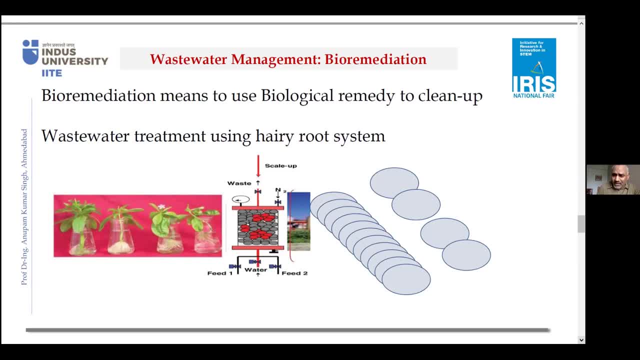 kind of things can also be done. So what we need to do is that we need to identify the plant, we need to identify the taste bed. Yeah, So a small area, one requires even kitchen also you can have, you know, that kind of a thing. 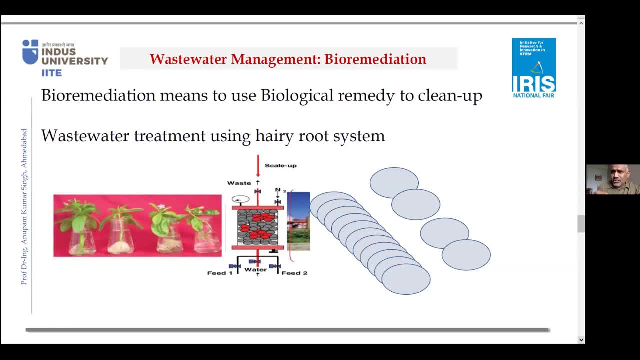 And then you see that, whether you know, this project is scalable, Yeah. So therefore one need to identify really these plants, you know. so there are many hairy plants which I'm showing you one of the example here, And therefore you know you can do the taste bed. 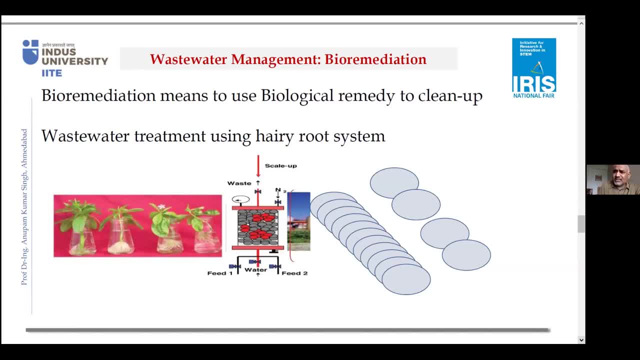 you can, you know, increase the distance, decrease the distance, you know, whatever things you like, you can do them. And there's a possibility in National Environmental Engineering Research Institute NERI in Nagpur. actually they have, you know, such taste beds available. I thought. 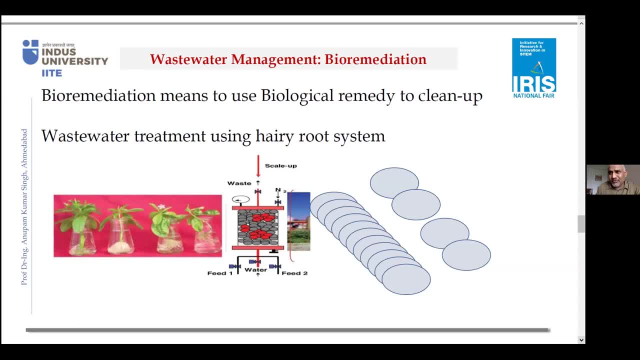 that I will bring one example, but since I couldn't talk to one of my friends, Dr Pawan, so I couldn't incorporate one of those things. Yeah, But I think the literature is available And in case you don't find that literature, you can ask Shreya Singh or you can ask Sasha. 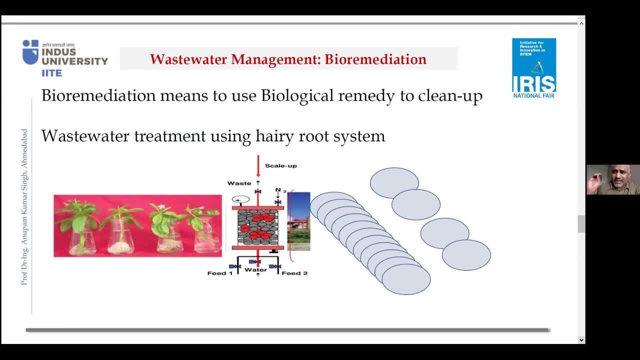 Kumarji, you know, they can always, you know, write me and I can, you know, send that literature, And I think you can read that as well. Yeah, The next one, please. Now the another area which I thought, that is water resource management. 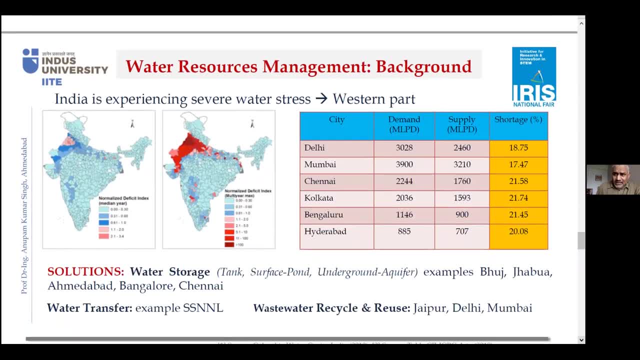 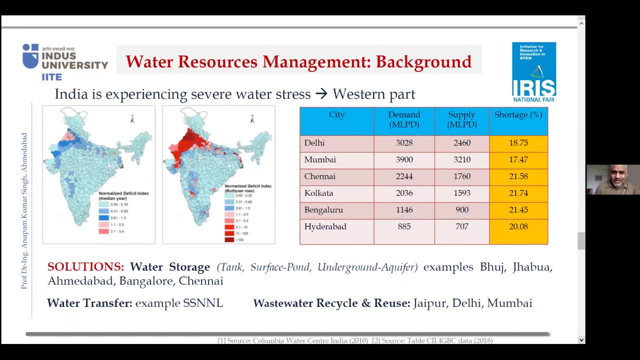 which is essentially important, you know, for India and because it's still. we have at least two third area in India is a rural area. we designate that as a rural area And, as you know that you know about agriculture is heavily dependent on on rainfall And 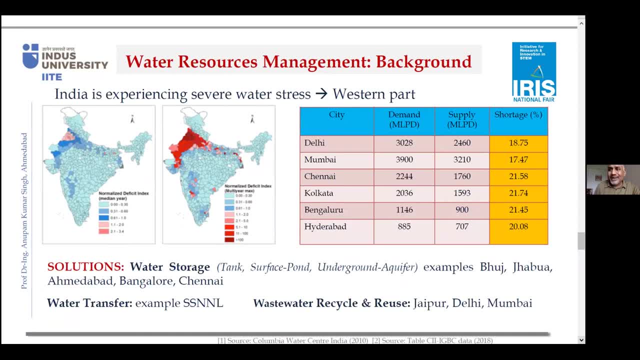 and that mainly so in the Western India. so I come from Gujarat and if you see here in Gujarat Rajasthan and also you know part of Haryana and of course Maharashtra and then part of Karnataka and Andhra is again you know the sites from Maharashtra. 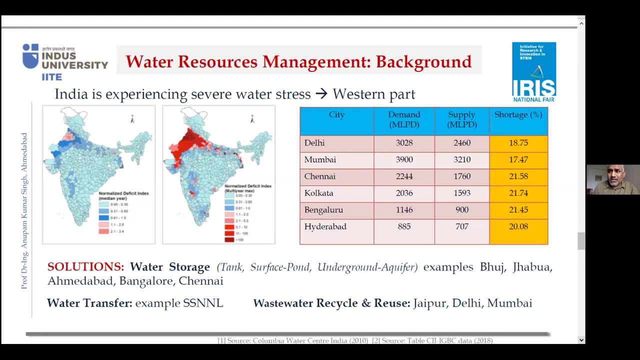 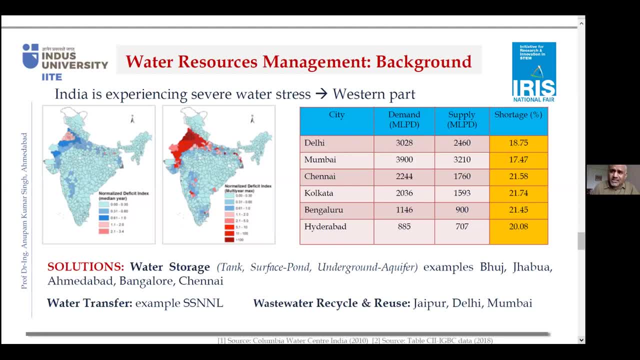 very, very good farmers are committing suicide in such areas. I think it's really a big problem, So we can also think about some solutions. Yeah, So I have given you this, this, this figure here in India, which is that you can even pinpoint your district from where you. 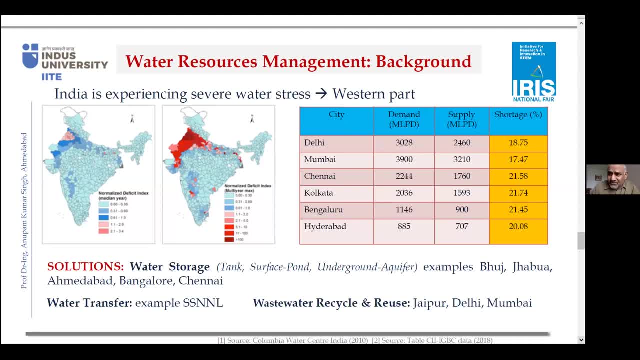 come and what is the condition of how much deficit it is, and likewise, And also the other. I thought that I will also compare actually this with the urban area. So I tried to bring our big towns, which India is having and 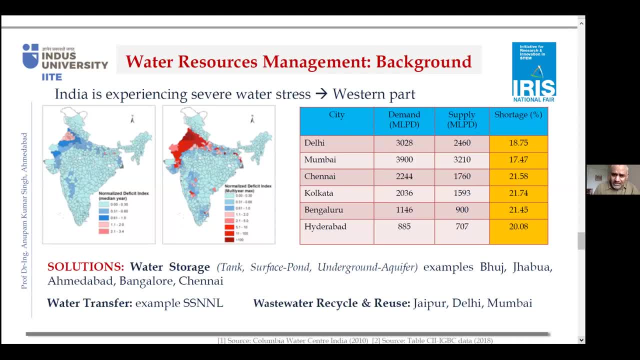 this data. I got from Indian Green Building Council, the data which is left inside for district level. I got from Columbia Water Center because Columbia University is doing research work here in India. I have been a part of that, such very so I mean this data. 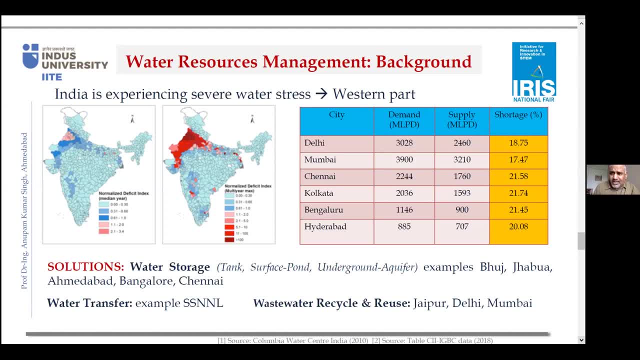 is from them And the right hand side data is from India, which is a part of that research work. So I mean this data is from them And the right hand side data is from India, which is a part of that research work. So I mean this data is from them And the right hand side data. 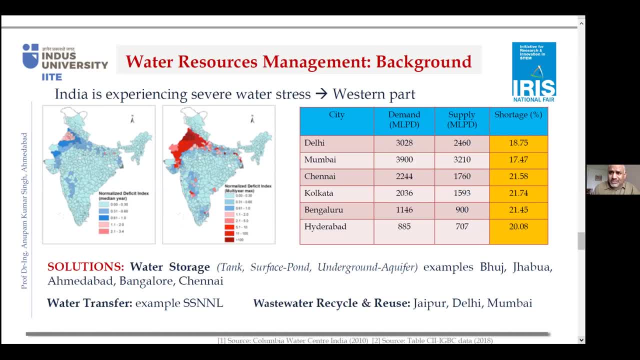 is from them And the right hand side data is from Indian Green Building Council, IGBC, which is one of the center of excellence of the Confederation of Indian Industry, CII, based out of Hidrobat, and they have given this figure And if you see here, Delhi, 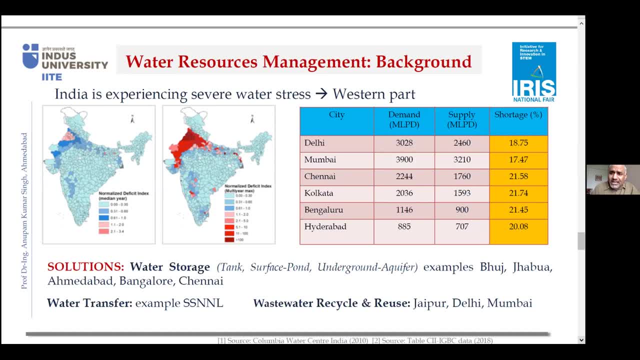 Mumbai, Chennai, Kolkata, Bengaluru, Hidrobat- each big city is in the deficit of so-called water. So they aresomebody is deficit. why 15 percent? the other one is deficit Y, it's a 21 percent. 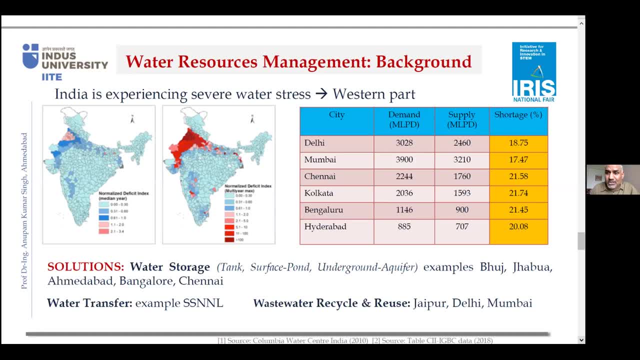 Each city is under deficit. The demand is much higher than the supply. Now we need really to go for think, for solutions which I told you earlier that we need to reuse and recycle, actually the water Right Now, when we talk about rural areas. 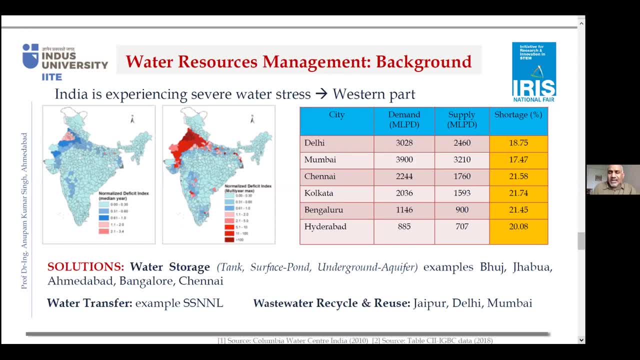 there are options and many of us know very well and many students- you must have visited actually one or other water harvesting structures or in terms of a bow, Here in Gujarat we call them bow and we have actually built beautiful bow in ponds, If you see here lakes for 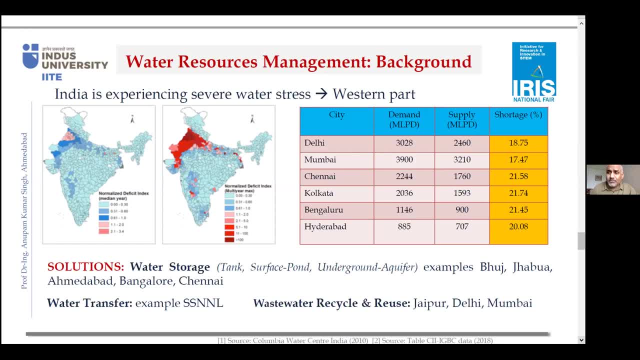 example, you know, Gopal has a big lake, and Udaipur, and yeah, so each city- has a lake. and in South India, especially in Tamil Nadu, if you see, we have an excellent system of actually having one pond connected with the other pond and the water in these ponds have been used. 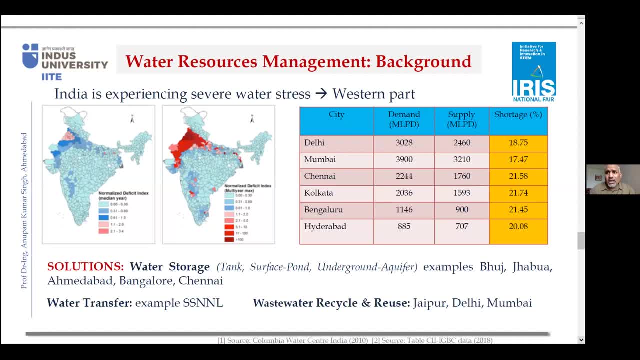 you know, for paddy cultivation, Again presents a best example of actually water cultivation. Yeah, We can store water in terms of these tanks, We can store water in terms of ponds, We can store water in terms of aquifer. Yeah, and I will give you a couple of. 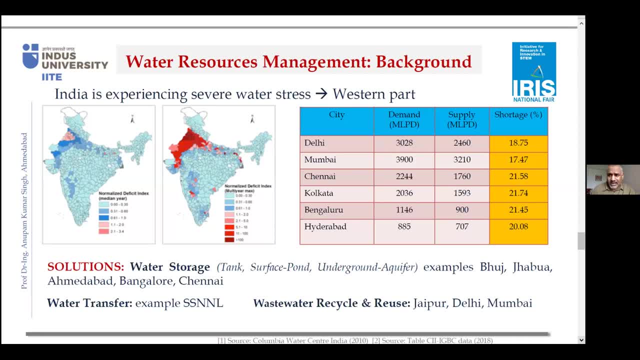 examples. you know how this has been done and you know those who are from Gujarat. they know that. you know. we have a bow system here, Rani Nibau in Patan. We have again Adalaz Nibau here in Nandabad, You know. so these systems are actually. 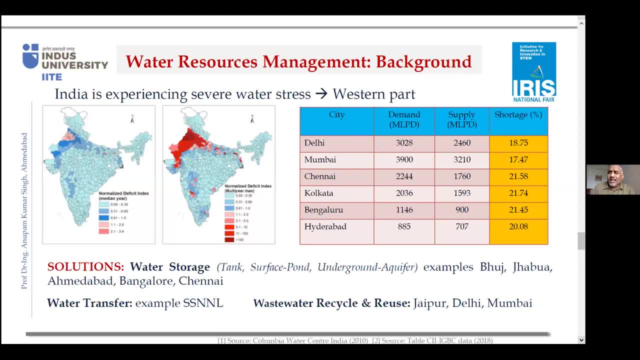 integrated groundwater recharge systems. you know, and one can I mean. they were never dried down, They were always actually having water. The only difference was that the water table was often going down, You know. so we can have those storage kind of a thing. Then again we have a water transfer schemes. 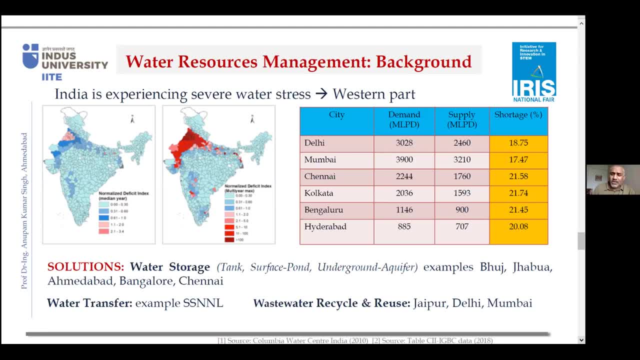 which are bit new schemes, Of course: Sadat, Saroba, Narmada, Nigap Limited. We are bringing water from Narmada River, We are recharging here in Gujarat, We are recharging the our Mahi River, We are recharging our Sabarmati River and we are 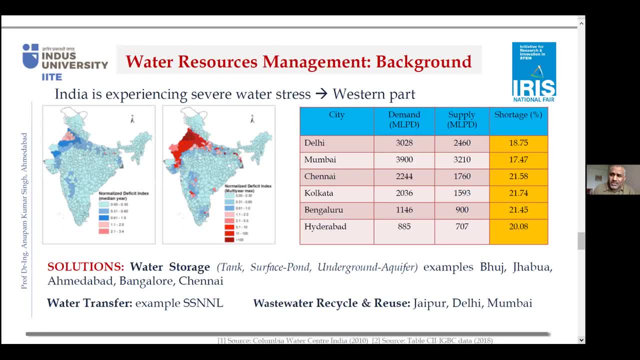 going further, the Rajasthan, and we are giving water Limited canal and then water recycle, reuse, and there are best examples, those who are from Mumbai, and there's a factory known as the Rashtri Chemical Fertilizer, RCF, you know So this factory, RCFI. 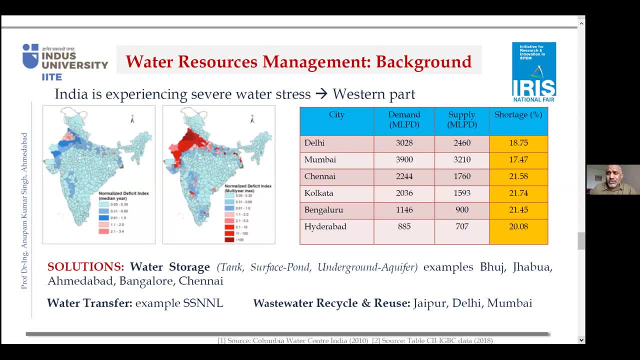 you know this factory is using actually base water for producing urea. Also in Jaipur, you know, we have a water treatment plant known as the De La Vaz- Sorry, base water treatment plant known as De La Vaz. We are reusing that water, base water. 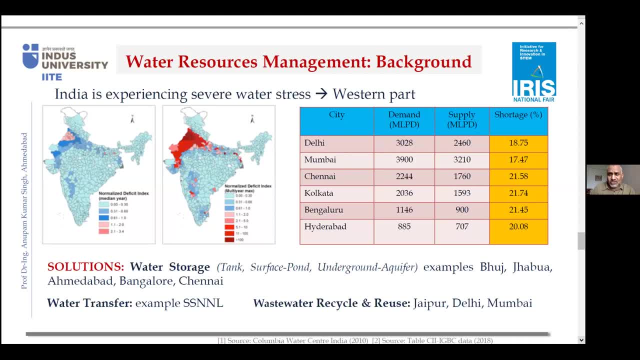 for agriculture in Delhi. again, those who are from Delhi, I can give you example, like the area which is very close to Sarita Bihar. you know, this complete area used to be actually irrigated by at the wastewater treatment plant from Okhla. yeah, so so. 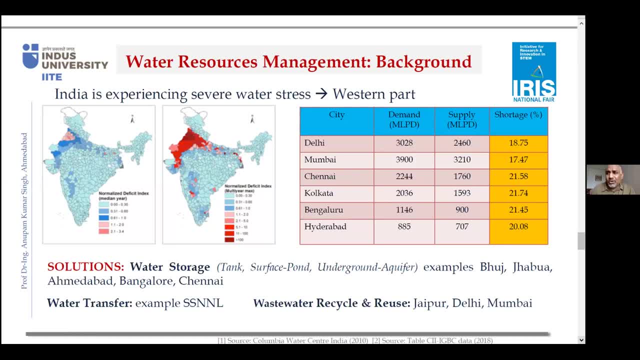 such based examples are available actually and I would like to take actually one or another. so I am taking one rural example and this place is known in the Jhabua, which is the district headquarter of actually Madhya Pradesh, adjoining with the state of Gujarat and also Rajasthan. so I did. 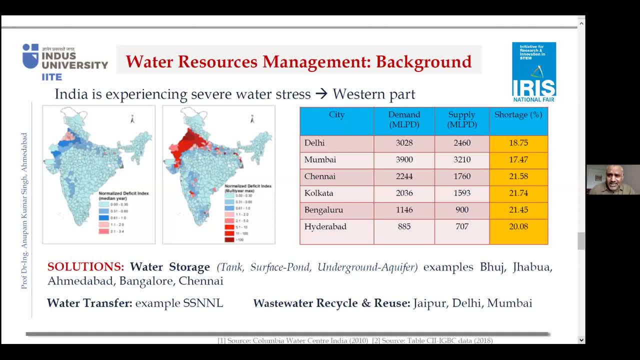 some research work here. so this area is actually, if you see here red lines which are extreme right side, you see that these red lines are the variability. so this year I received approximately 750 millimeter rainfall per year and some years actually this rainfall is 1200 millimeter and some years this rainfall. 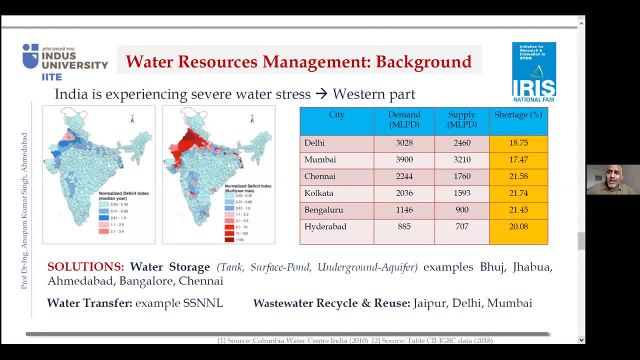 is just 300 millimeter. so if you see the variability, this is approximately 300 percent, three times more variability. so today, if my income, let's say, is 1 lakh rupees and I just received 30000 rupees, how will I survive? yeah, so that's the big problem actually of for water. 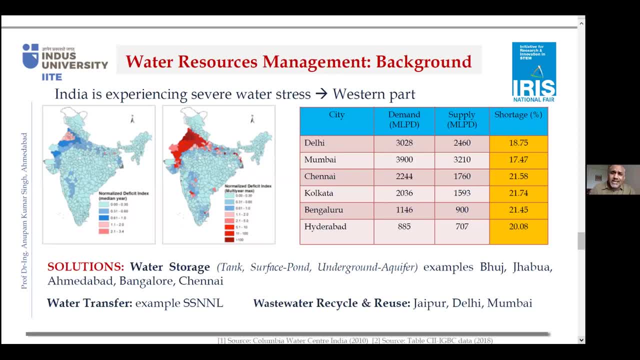 here in these areas, although these areas they have a very strong, rich tradition. it's tribal area and I'm telling you, the people are so nice and you know they are so pure with heart and so really in they have a strong, very strong cooperative practices and one of the practice they call it Halma. Halma means if somebody 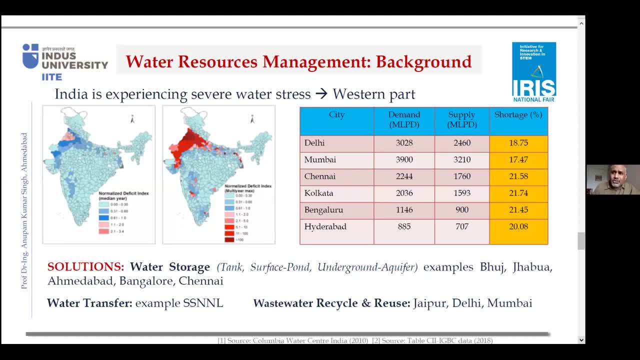 says that this is Halma means everybody is going to help that guy free of shells. the one important thing which I model, which I could draw out of the social understanding in Jabua, was that- and there are certain NGOs who are working in this area and they say that these people are actually very dharma. 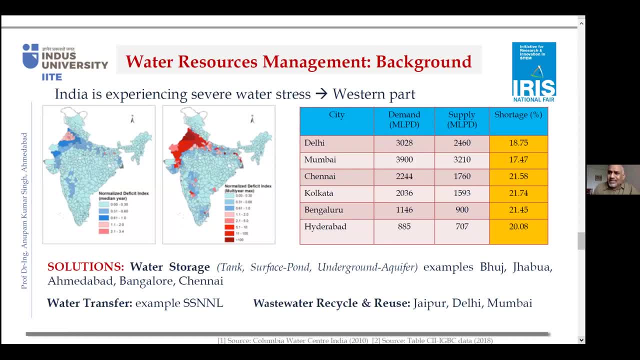 oriented. dharma generally means religion oriented they are. dharma means they are the one who you know consider work is a worship, yeah so. and then they consider Parmarth means helping others is their prime duty. they also say that they are very Swabhimani. 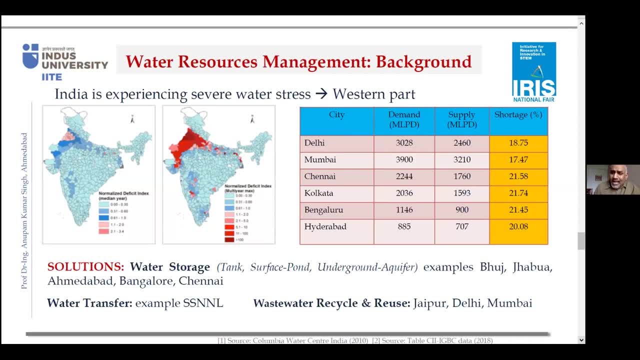 who are independent, you know, and also sorry. so Swabhimani means they are very respectful, yeah, and swablambi so they are also, know, independent And since Dharma Parmarth, Swadhmani and Swablambi when these kind of 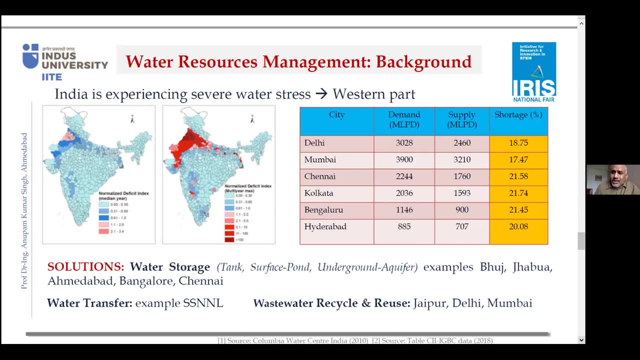 four things happen in anyone you know. that person becomes automatically, that area becomes automatically sustainable. So therefore, in Jagua area, sustainability was not a question actually till maybe 200 years back And when you know, forest was exploited when their 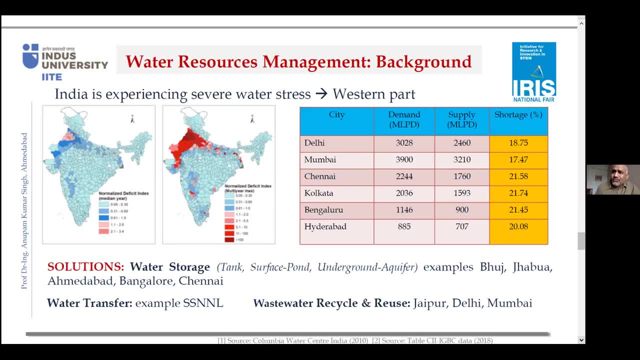 animals were killed, when their lands were, you know, taken and when there was no water, you know, the people's life, you know. and then again I get here five J: jungle, jameen jungle and jungle. 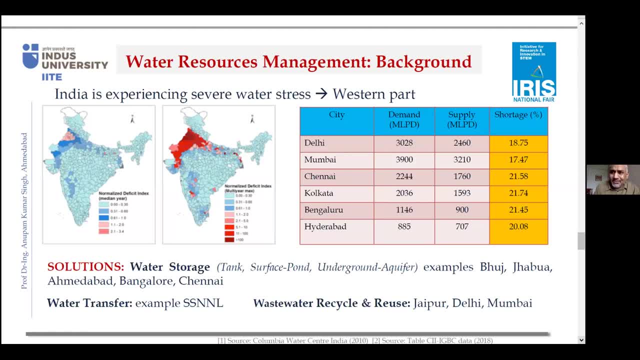 So this is the story of Jagua: This kind of integrated system, actually, when we are having, then a sustainability, actually will happen. Now, what they have done in terms of water, so what they did, actually, they have an approach which they call it actually ridge to valley approach. This means 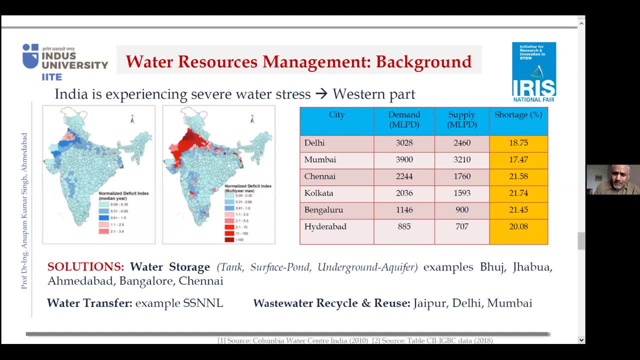 this is the GIS map which I have, and you can see here that from top until the bottom, this means until the river, And then you can also see in these figures which are there that some of these techniques were used in order to reduce the flow of water in these areas. And since water flow was reduced, 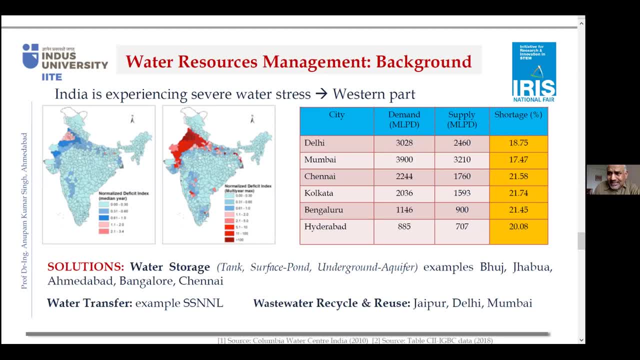 the water halting time was increased. This means, if you increase the water halting time, what will happen? The water start going rich has into the groundwater. And this is precisely the problem that makes the minorities that majority of our cities are facing today. 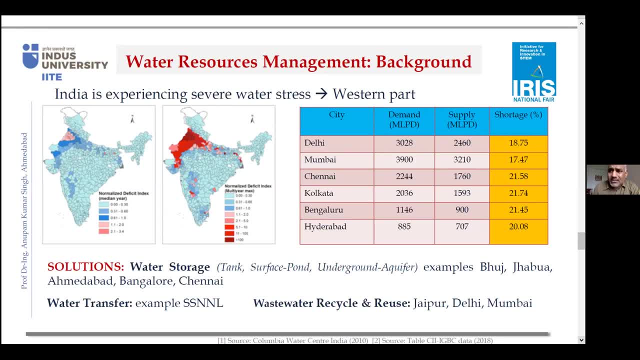 You see, Jaipur is under immense flooding. not Jaipur, I think all the towns. Delhi is always under immense flooding, Mumbai, I don't know what kind of decision makers we are sitting that we are unable to solve consistently the problems which are occurring. 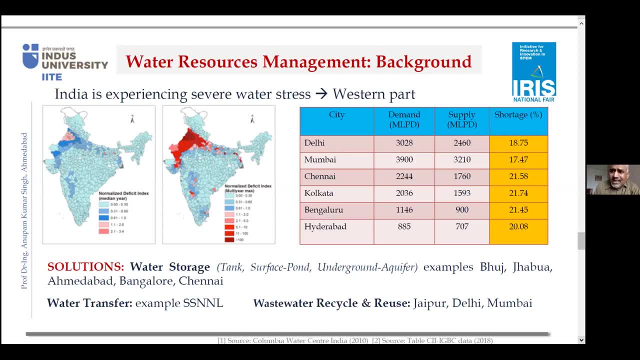 actually in our cities And so, you see, in the rural area, they started actually developing this kind of a water conservation in water harvesting techniques. And not only that, as I told you that people they do the halma, so they come together for helping others. 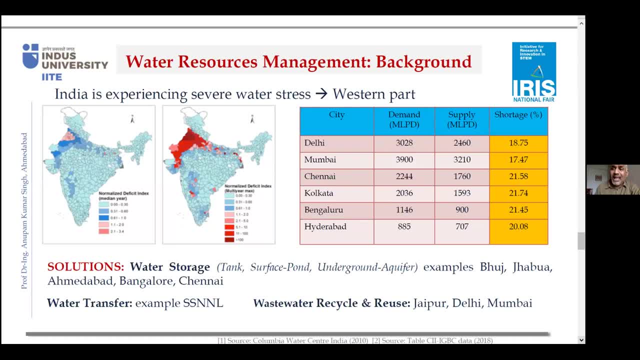 Now in cities we have lost that tradition of helping each other. So therefore I think there's a possibility to re-digit these technologies and see the implications and viability of these technologies under the city conditions. So some of these students can think of working. 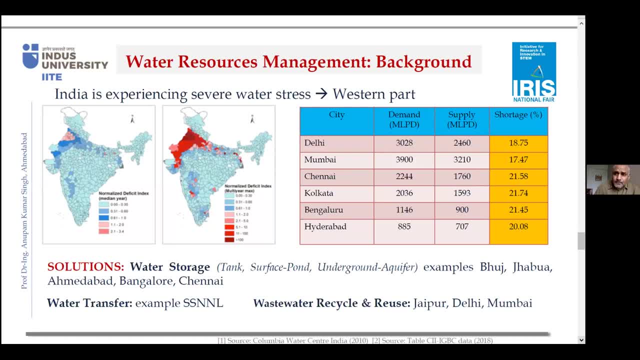 and showing them in some of the models of that Another example I want to bring it to a beautiful city of Bhuj, actually, which is very close to our Pakistan water, So Bhuj city almost 450 years back. if you see this Bhuj city. 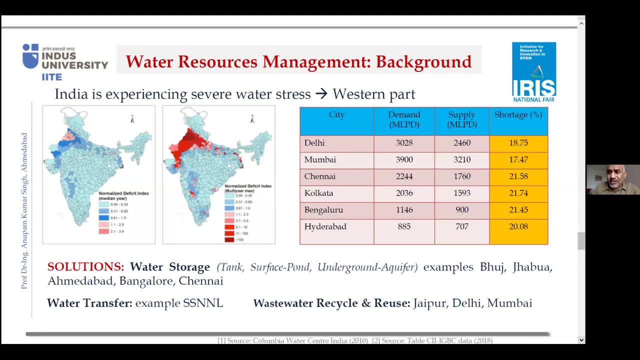 Bhuj city was having a elaborate water management system So they were taking water. it dropped, which was flowing from the hill, used to come down a little bit, Yeah, then further there was a dam, and then further, you know. 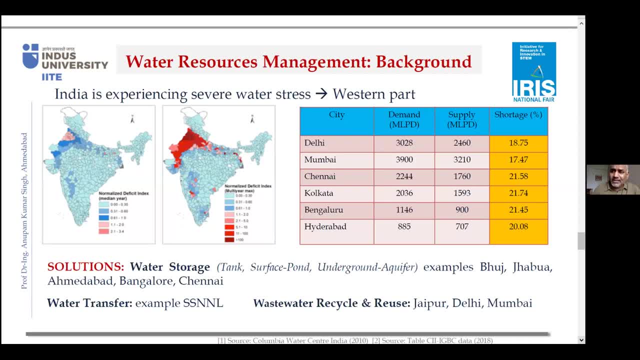 and then, finally, the water comes to the lakes, And not only one lake, it comes to a number of lakes And if you see, here I'm showing you that you know the rainwater collected in a series of lakes. So we have a Dhobi Lake, we have a Hamir Saar Lake, 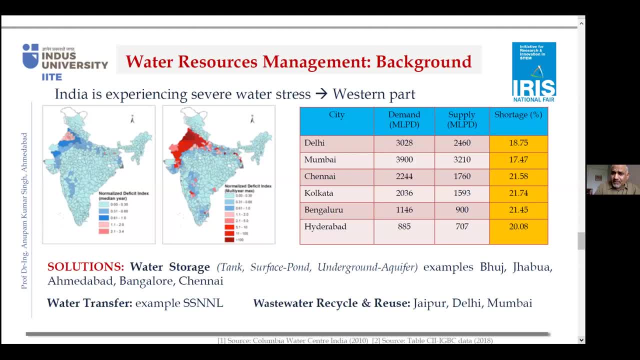 and then we have a Praga Saar Lake. Now you see that the cities were built in such a way. I mean, this Bhuj city is very, very old city. may not be the time of Dholavira or Lothal. 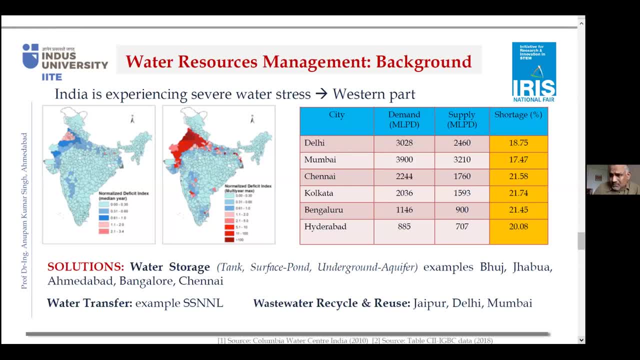 but this is also pretty old town actually, maybe at least 2000 years old, yeah, So if you see that town, I mean what is happening? that these towns were situated, you know that these towns were situated. you know that these towns were situated, you know. 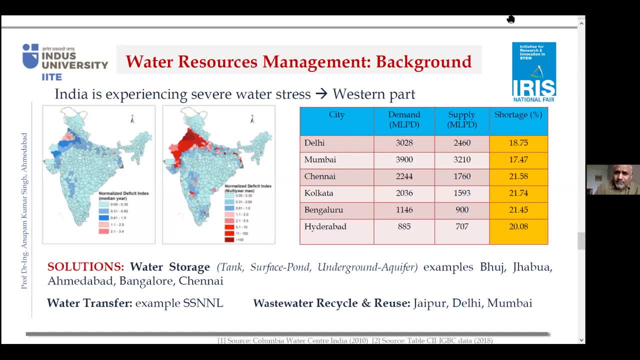 somewhere on a such a condition. you know where, you have a geology. So you see, here I put a geological map of that area and there are falls actually, And then you see that the underground slopes over the you know lakes are built in such a way, you know. 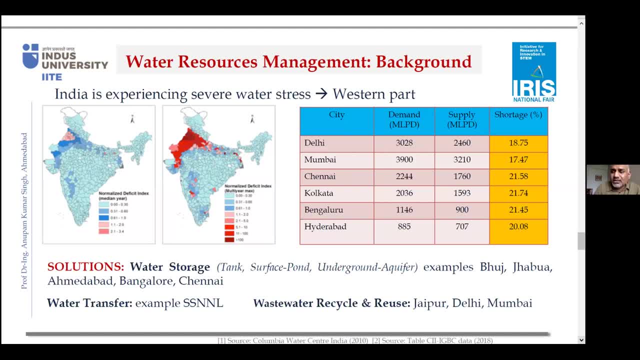 so that everything actually, at the end, falls on, you know, on that fall, yeah, and so therefore the water, because this layer is an impervious layer and therefore water can be very well stored. Now the population has increased. 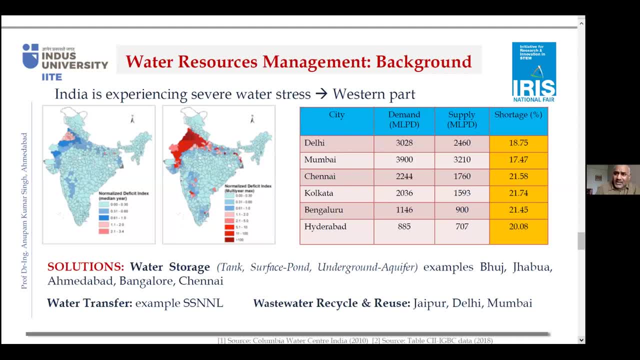 since population has increased, then we need to think about, you know, some degree of technologies for here Now, one degree of technology which is very important, and since this is a computer era and I do a lot of computer work and modeling work, 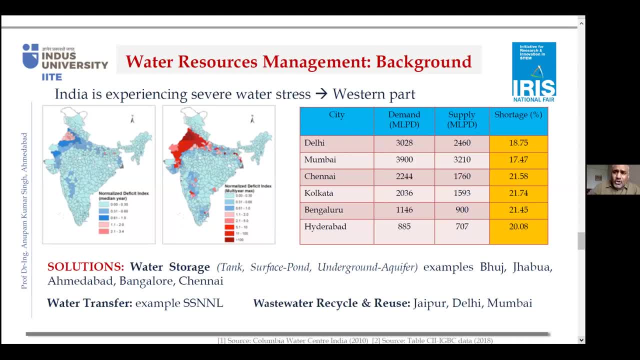 and therefore what I'm thinking, that some sort of a locational enabled water database system. So if we know that how much water is in which lake and how much water will be at the end of you know, one month, two months, three months, 10 months. 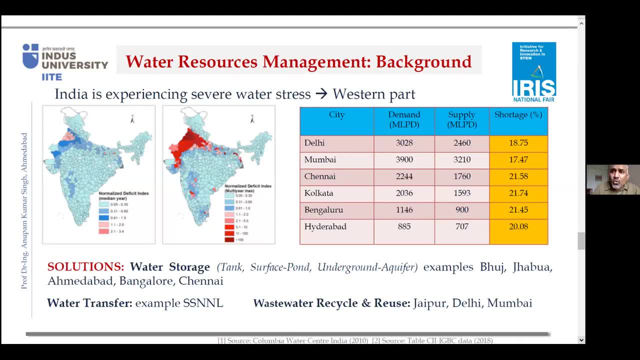 you know one year. therefore, you know, we can know, and if that information is available then we know that how to use that water. yeah, so that knowledge system actually we have to bring in the natural cycle And those who are good in- perhaps you know, in computer. 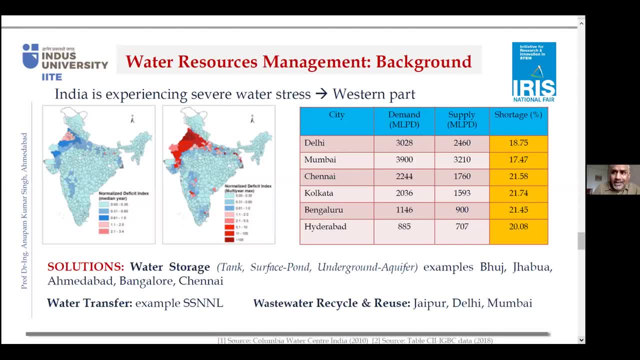 you know they can think of having certain degree of applications. yeah, So this means applying computer to the natural systems, and once you have a better understanding of those natural systems it is much easier actually to predict the behavior of those natural systems. 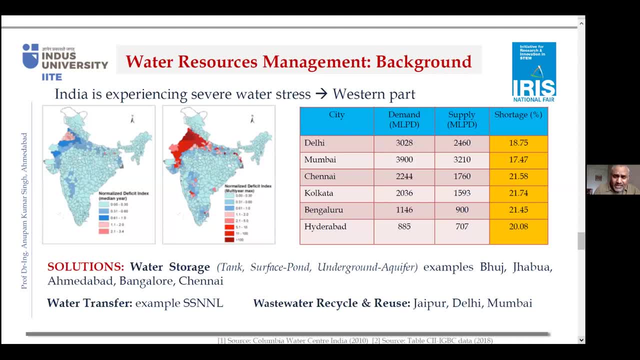 Lake conservation and cleaning could be one. yeah, And again, for example, floating boat. you know so, if a bend, you know when the boat goes into from one to the other side and automatically the bend direction changes, it comes. you know so self-cleaning kind of a system. 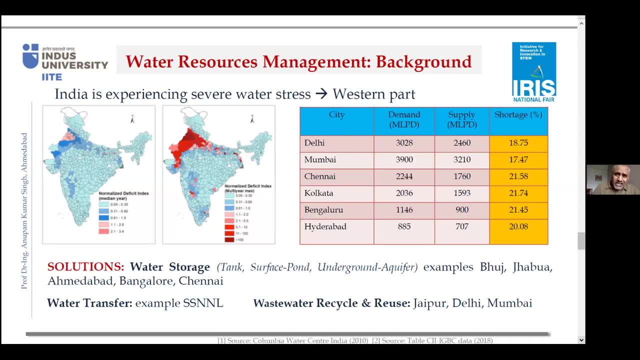 actually can be also installed. Some of you can think, based on Archimedes' principle, yeah, Flow measurement sensors, for example. we can, you know, install at various levels places, geographical investigation devices, for example. Today we calculate the electric conductivity. 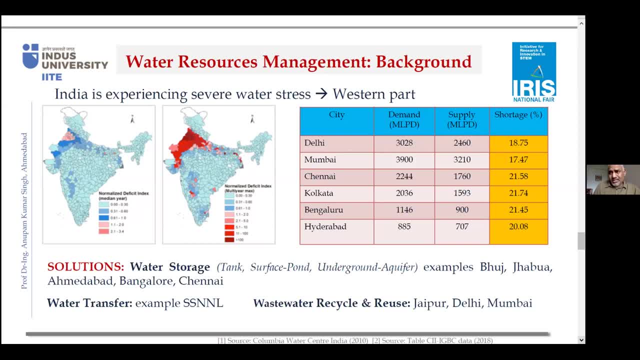 in order to measure, actually, the so-called geological profile and tomorrow maybe, if you can think something else, some other parameter actually in order to build those devices and those who are, uh, actually aware that even magnetic field, you know, if there's a water you have a high magnetic field. yeah, so if you take actually, 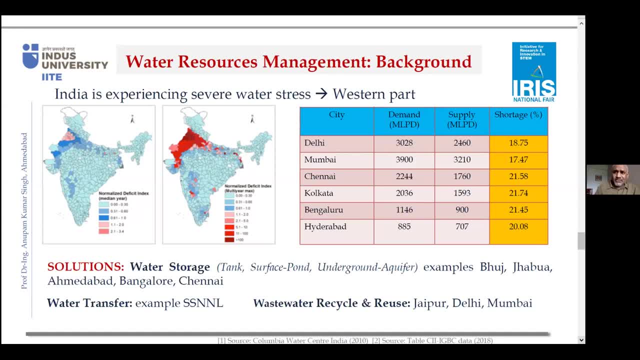 that magnet in the area, yeah, and if the water is there, then this water attracts actually the magnet you know towards- uh, i, i mean those kind of fuel theories are dominant actually in the so-called rural areas and villages. so some knowledge there. i think one can also have that knowledge together with the technology in order to make 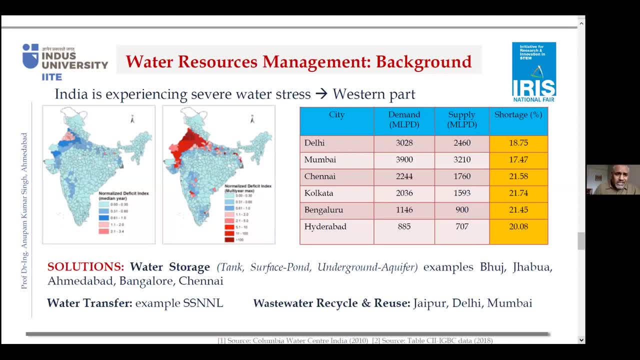 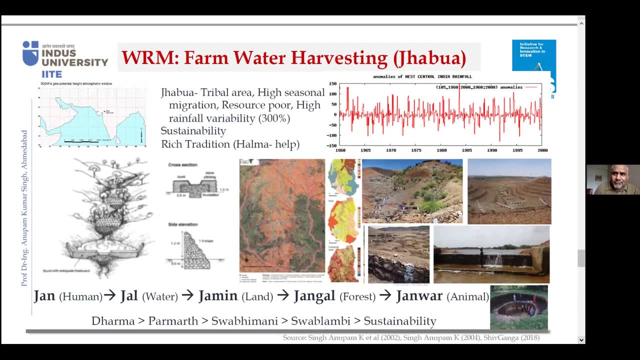 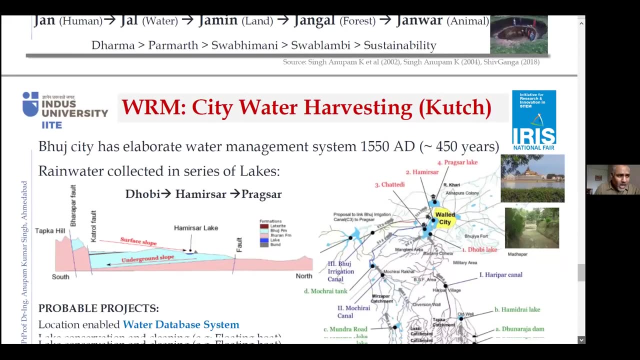 new devices. next one, please? yeah, so these were the technologies which i talked, actually, uh, with all of you, and i tried that i should not give you much clue, but i should give you sufficient clue to do something by yourself. yeah, and now, if you have to develop the project, what are the various steps which are essentially? 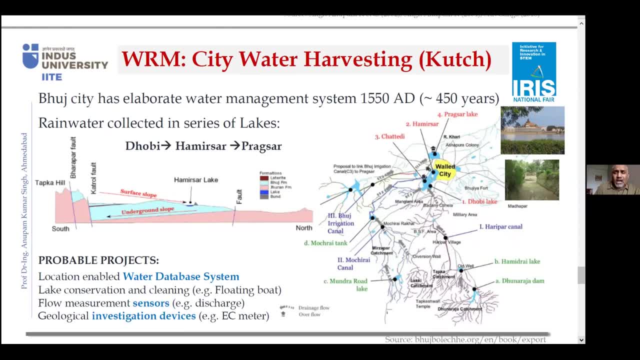 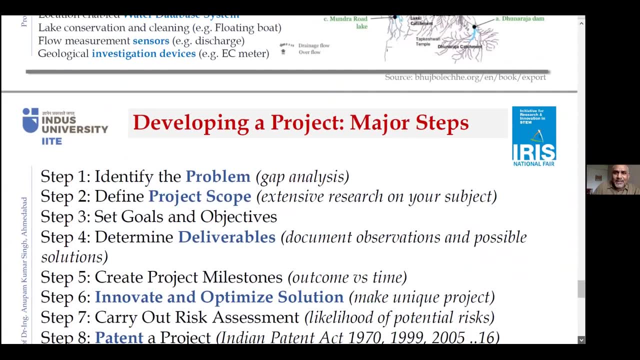 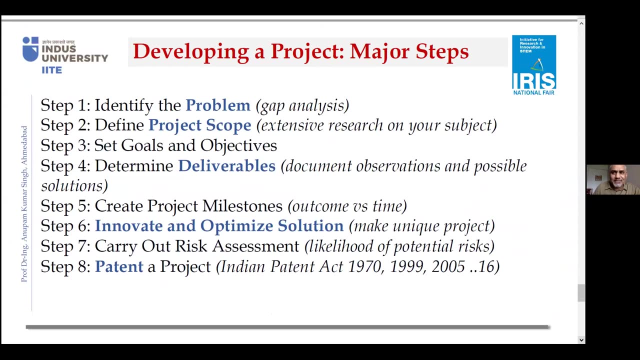 important for you to consider. and these are the eight steps. normally we tell our phd students, telling you these eight steps. yeah, so first step is to identify problem. now, identify the problem is the best way i have done. i have shown you, see, i have shown you the water availability. 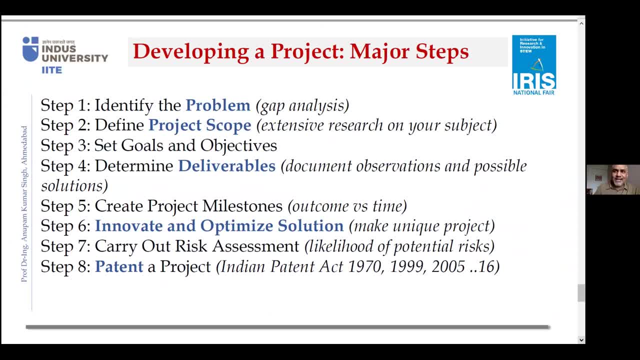 i have shown you the numbers, i have shown you the demand and, based on number demand, i have shown you what is the game now, in order to give address that gave, in order to fulfill that gave, what kind of project is needed. so therefore, you can define actually the project score based on this care. 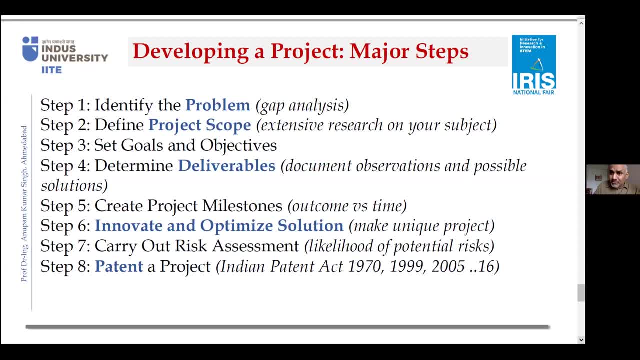 so, therefore, you have to go for extensive research work on the subject. yeah, and once you go through that extensive research world, then you can so-called set your objectives, that my objective is to develop a device, you know, which can major electromagnetic field. you know something like that. so this is therefore important. yeah, and then once you know, 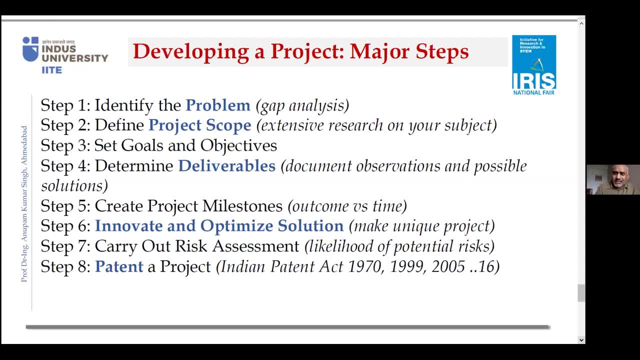 that, that this is my objective. then you think that what will be the delivery? deliverable is the idea, deliverable is a sketch. what is the deliverables? yeah? so therefore you see those observations and then see into the deliverables means possible problems, right once you know those. 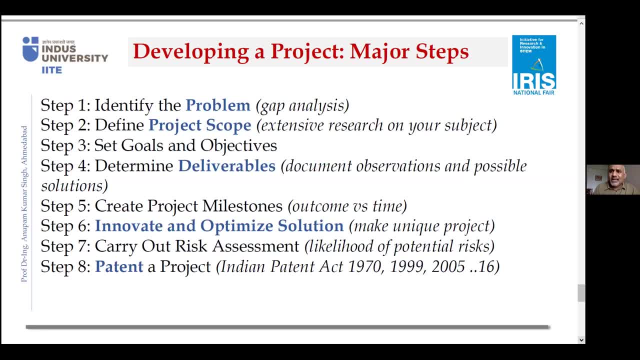 deliverables, then you have to define that these day will. so i bought time. this will take a month, two months, this will take six months, yeah, so like that. so, therefore, you decide so-called your milestones for the given project, yeah, and then what you do is that then you look for various solutions and you say that: 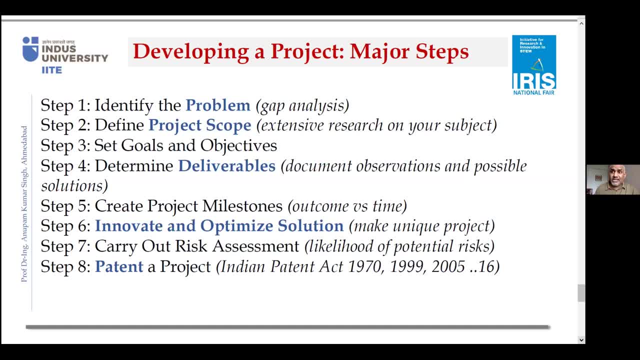 this solution is the best one. so maybe you have three solutions: solution a, solution b, solution c- so it's not only one solution. actually, engineering is never one solution. so it's not that physics problem can be solved only one way. no, it's wrong. physics problem can be solved into three ways. 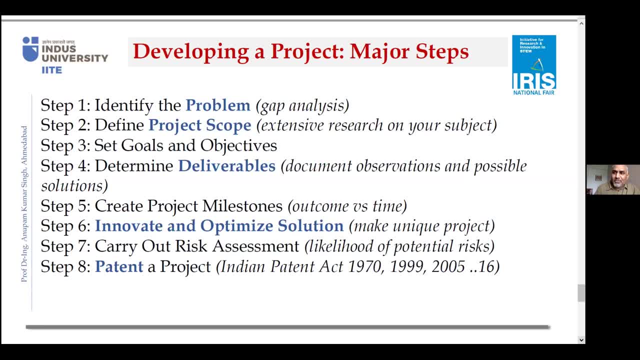 let's say, if i want to measure the height uh building, i can measure the height of the building simply barometer and measure the height of a building using barometer. so some guy can say that, okay, he will take a barometer, you know, from the ground level he will go to the top history. 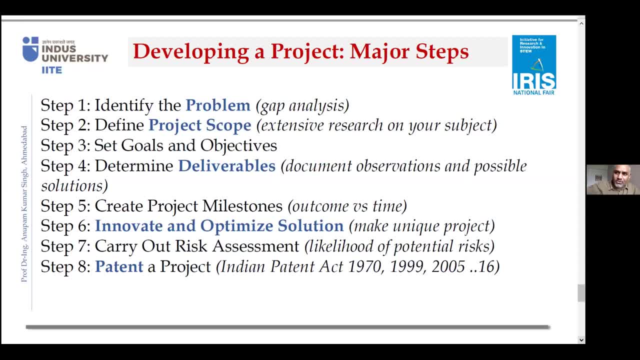 take a thread, you know, put the thread down, put the barometer actually in that thread, measure the height and take a tape and measure. yeah, somebody will say no, i want to look into pressure difference. yeah, that, what is the pressure here? what is the pressure on the top pressure? 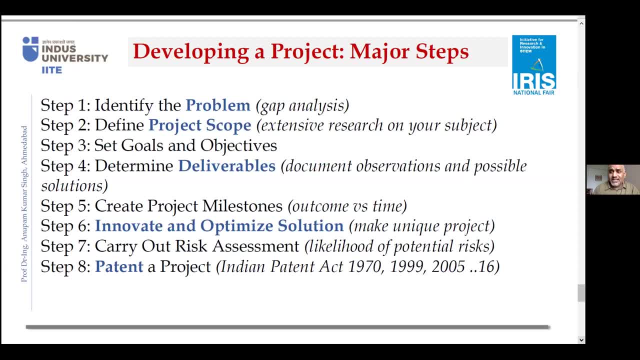 difference gives me height right. so when somebody will say that no, i will take the barometer one time, barometer second time, barometer, third time. so you keep on, keep, you keep on putting barometer until you reach the height. so there are so many solutions. what i want to tell that in engineering, 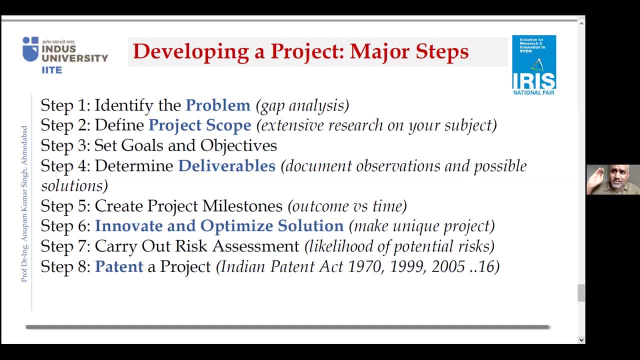 there are multi solutions. they are not. even this solution is not single, okay, so therefore, you innovate and see that which one fits you well and, as i told you, look into technology, look into society, look into the ecosystem, yeah, look into the economy. and when all these four, five things are, 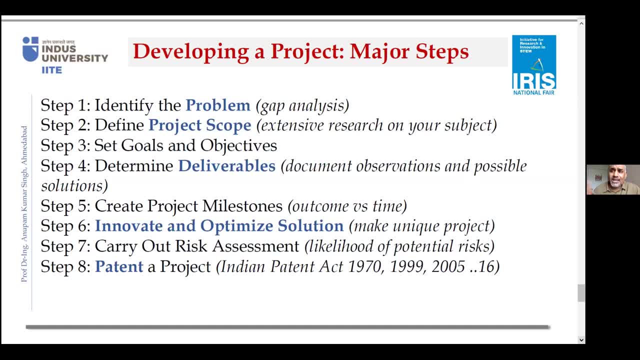 good and it's fine. today i have no capacity to buy. i have a capacity, let's say, to buy- maybe you know fortuna- but i have no capacity to buy mercedes. so tomorrow, when my capacity increases or decreases depending upon my decision, you know my decisions to be based on that. so therefore, we 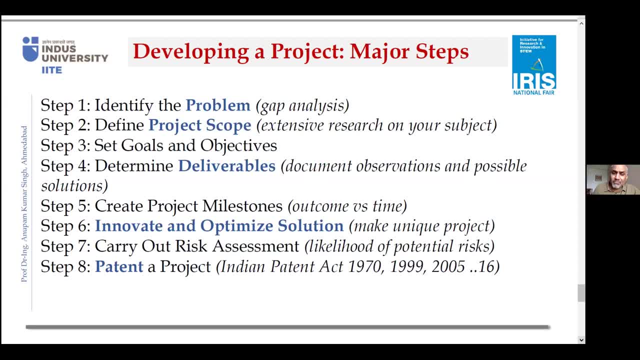 have to optimize those solutions. so optimization means that and also a carry out risk, because it's very important that whether somebody has risk appetizer, if you say that no, your project fails, then you know you should not lose heart. i mean, it's okay because you are learning, you are 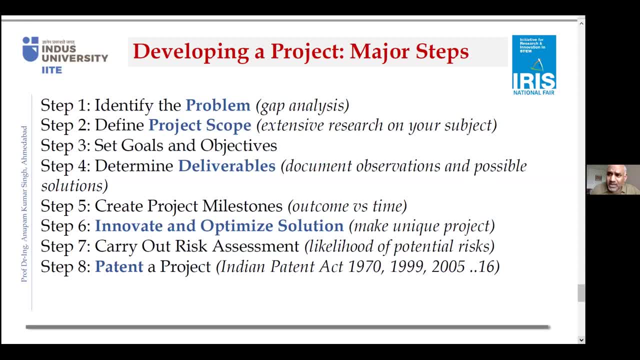 doing something. so that risk is very important and if you are into prototype and you are not able to make product, doesn't matter, maybe next time we will make. yeah, so that risk assessment and look into the likelihood that, whether the microchip, what is the success? uh, likelihood of success and also 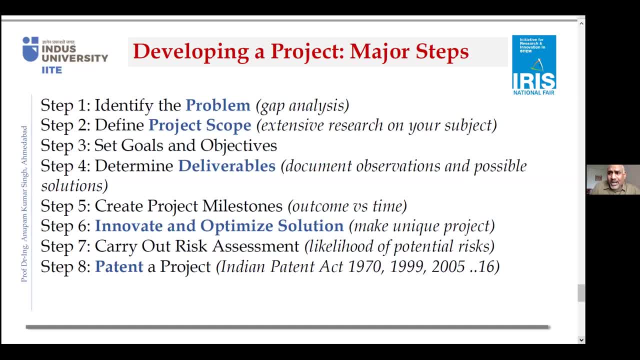 risk is important, yeah so, and then, once you have that so-called prototype, build your product, build. then you go for a patent. yeah so my students- let's say, at least you know, let's say phd students, almost 50 percent of them- they go for patent. yeah, so this means each year you know one. 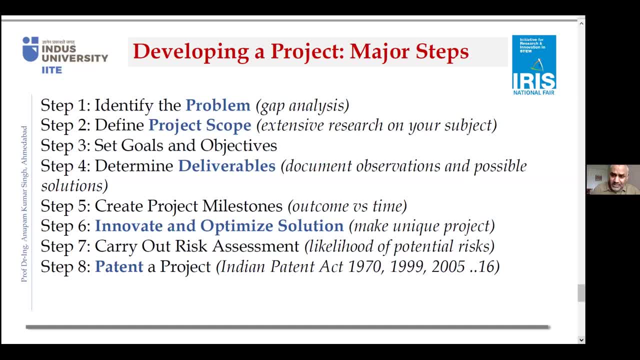 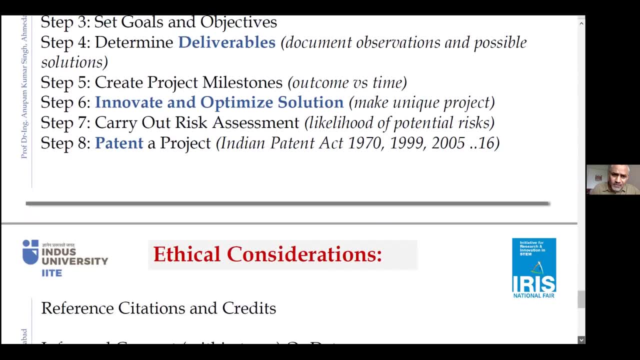 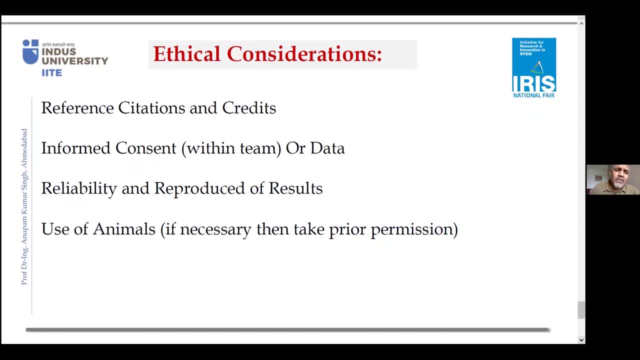 are. they say, second year we get one patent. yeah, so something like that it can be done. now there are certain ethical issues. next one, please. yeah, so there are certain ethical considerations and uh, because, uh, at this level there are not many difficulties. the only thing we need to keep in mind is that, if some thing is done, 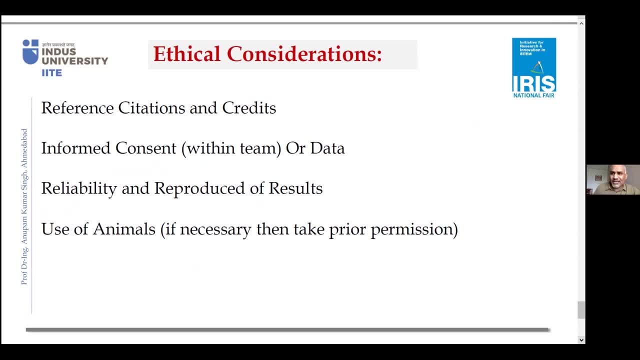 by somebody. please cite that and give it due credit. that's point one. that's an ethical issue. yeah, so, because it's not a plug region. yeah, so we should not collect that's one unknowingly what has happened, and it's okay. but you know knowingly we should not do that. yeah, it's important informed concept. 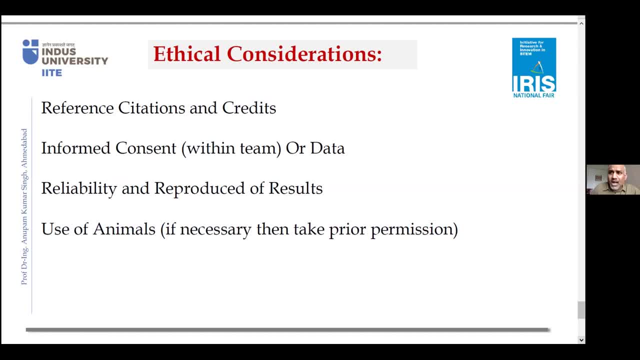 yeah, this means if you are working in a group, always have to inform everybody. so, for example, if i am writing a paper, yesterday i have submitted a paper to bailey- yeah, publisher in canada, and so i am having two more co-authors, so i must tell them that i have submitted this paper. 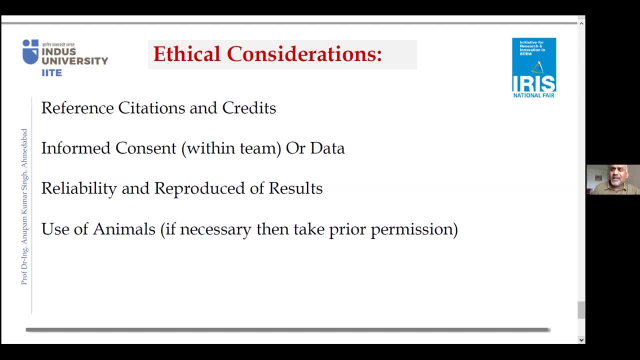 you know i'm the first author, yeah, so transparency within the team is very important and if somebody has given you data, then also please make sure you take consent, yeah, that you are using or not using. yeah, and then, whatever you do, reliability is very important- that if you have built something, 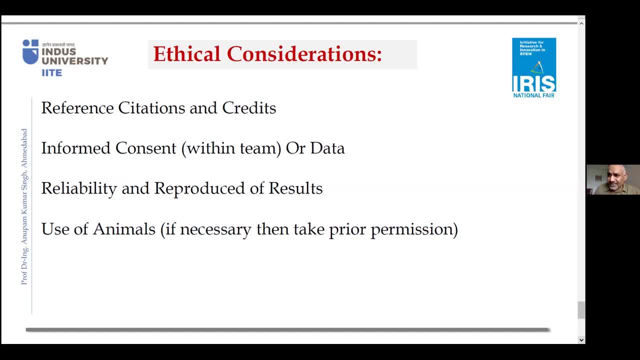 how reliable it is. you get 80 reliable, it's 90 reliable, it's 100 reliable, excellent and also not reliable alone. also reproducible? yeah, because in technology, reproducibility- because it has to come in the market- is very important. so therefore it must be reproducible, your results must be reproducible. 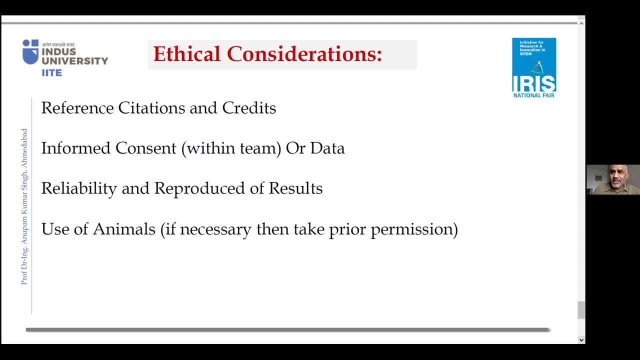 this means today, if i'm measuring x things with a tape, then my team must perform same after what i am doing, year after two years, after three years, right, and also try not to use humans or animals. i have written animal because don't do any experiment on humans or animals, yeah, and if you have to do it, 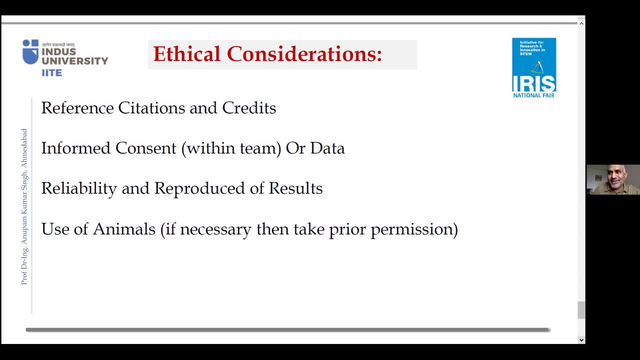 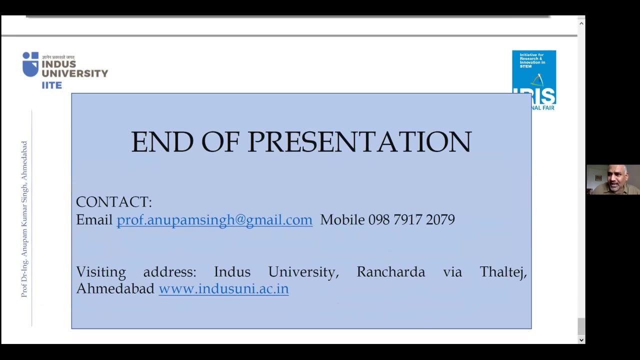 then please take a proper permission and then you can do that. yeah, so with these words, you know, i am, have you know, ended my presentation. i once again, you know, wish that i'm sure that you must have had a very nice. you know, understanding, and if there are questions, 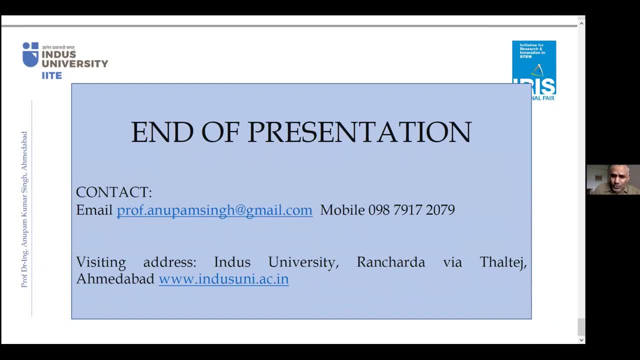 i will be very happy actually to take them and, as i told you that my email is also here, you know you can also talk to me. i also work with the ministry of india council of technical education and they do have, you know, sometimes some fears. so i do commit just there, but never. 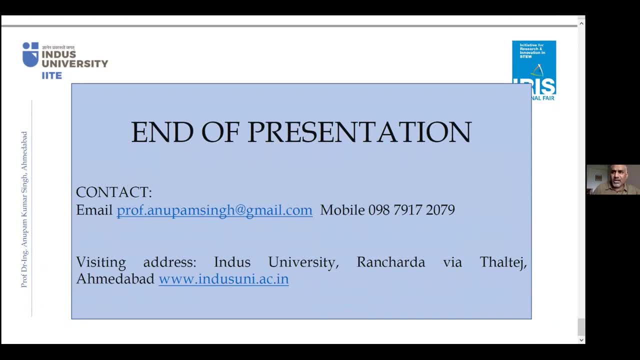 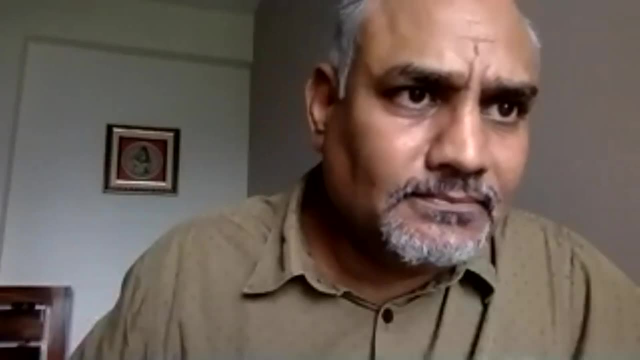 please you know. if there are questions, i will be very happy to to answer them. i once again thank shrey for taking me, i know, through this presentation over to shrey. thank you so much, sir. it was a real nice talk and we we are delighted to have you. 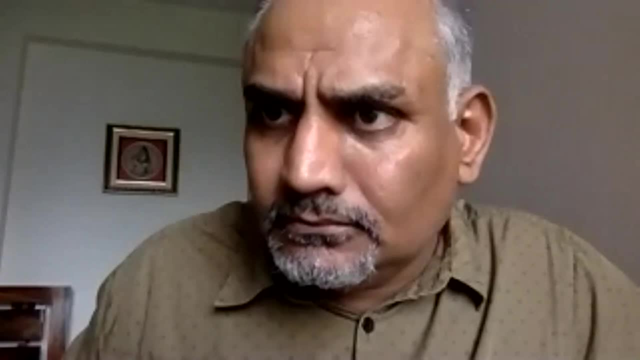 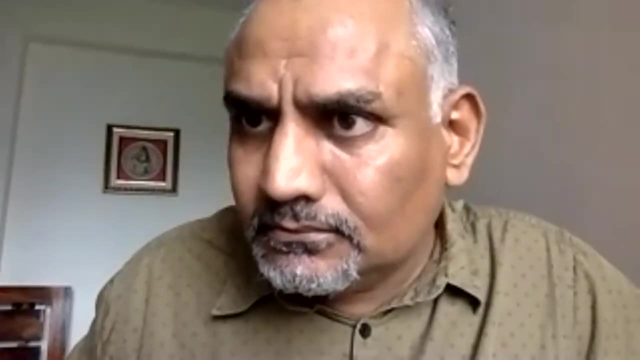 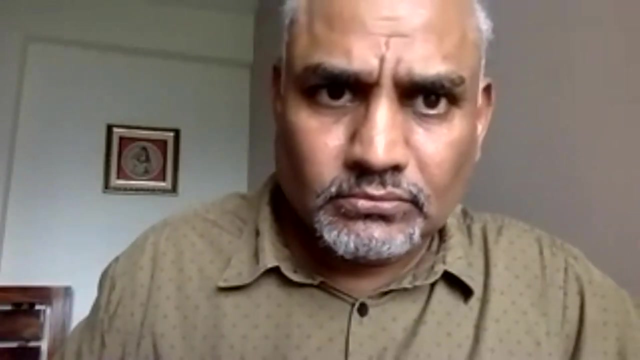 to have to share knowledge with the students on environmental engineering. so before we begin the q a session, i would like to play a small video for the students. one last thing before we subscribe to our channel. if you are new to the channel, i'm shrey and i'm also shrey. he is the chair of the organization of environment science at the university of india. 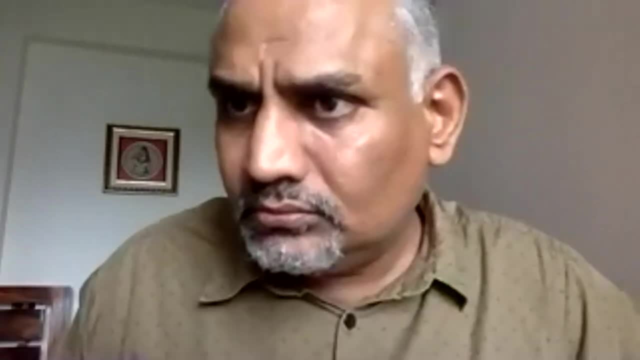 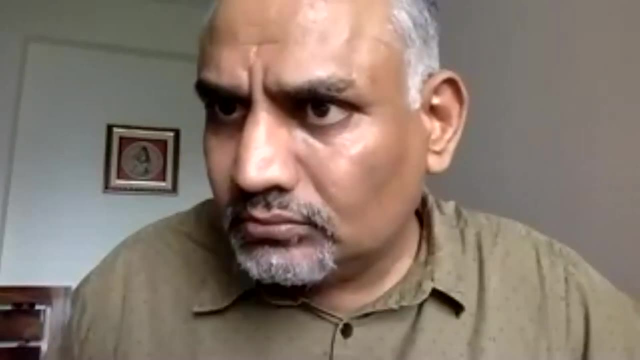 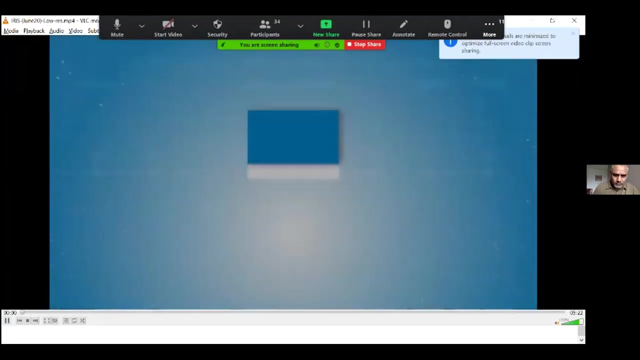 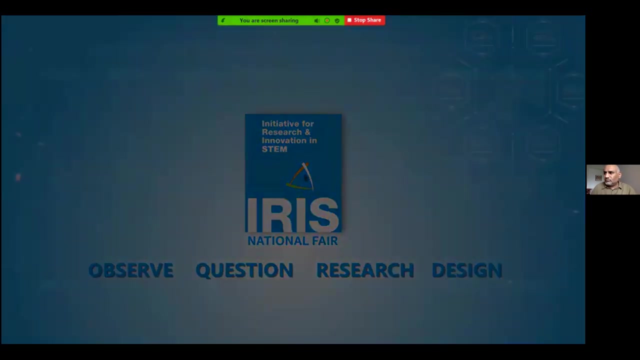 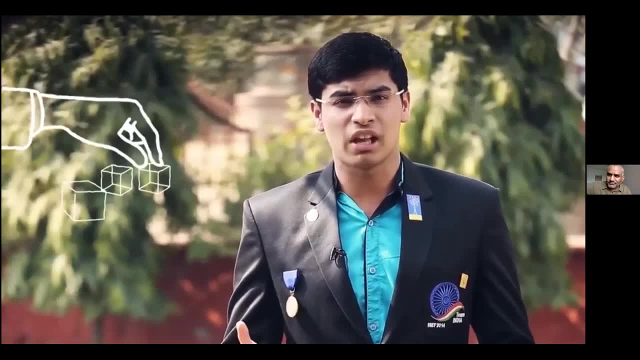 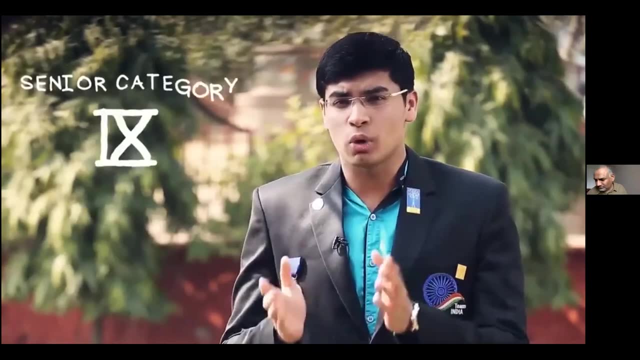 Your first step is picking a category you can enter by yourself or with a partner. If you are in 5th to 8th standard, you will be in junior category. If you are in 9th to 12th, you are in senior category and have a chance of making it all. 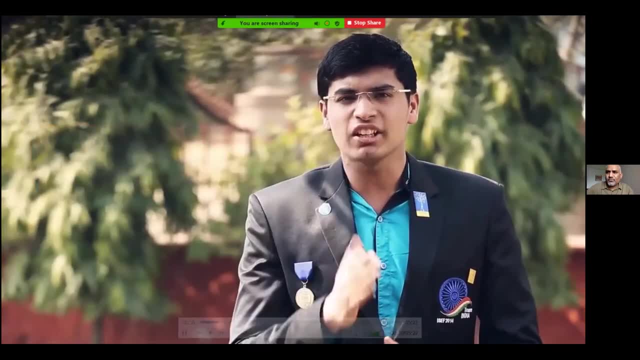 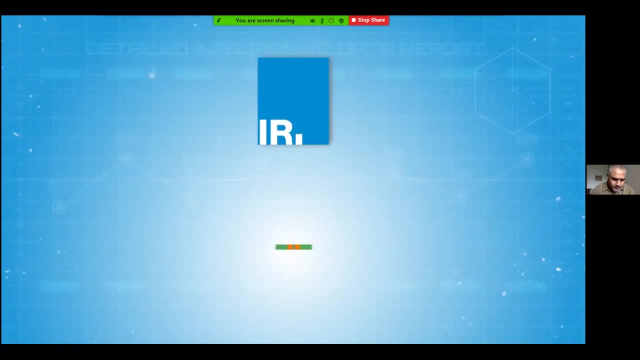 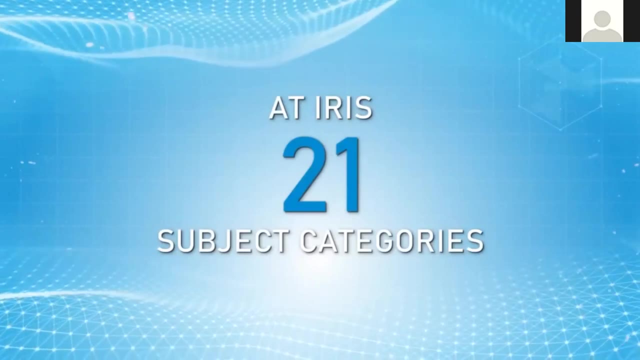 the way to ISAF. Now that you know which category you are in, it is time to find out which subject your project comes under. At IRIS, you have a variety of 21 subject categories to choose from. ensuring that your project has a category that fits. 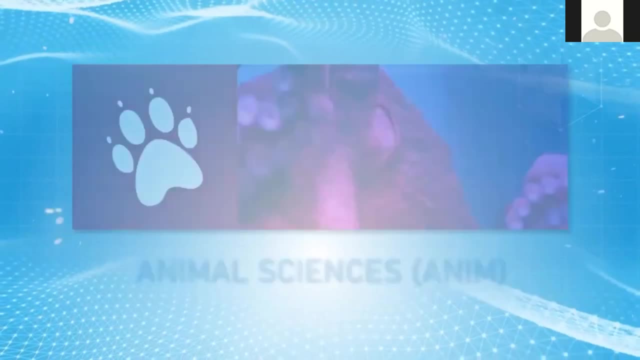 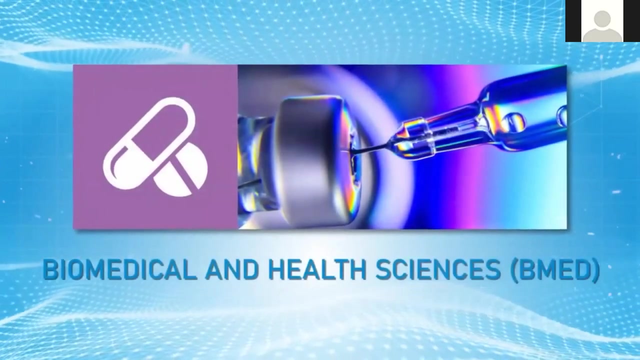 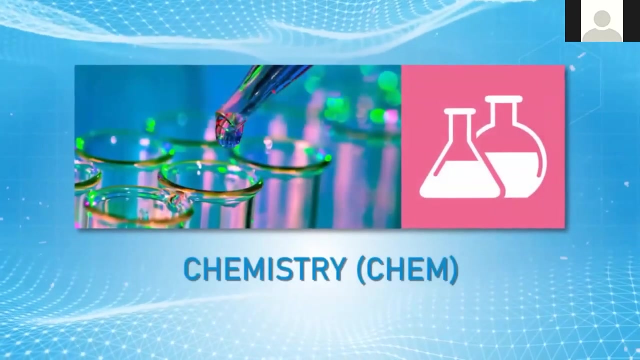 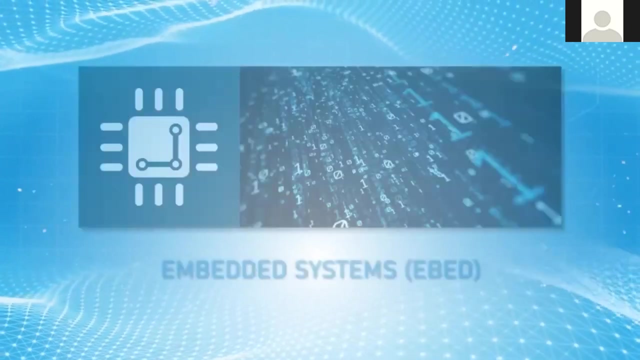 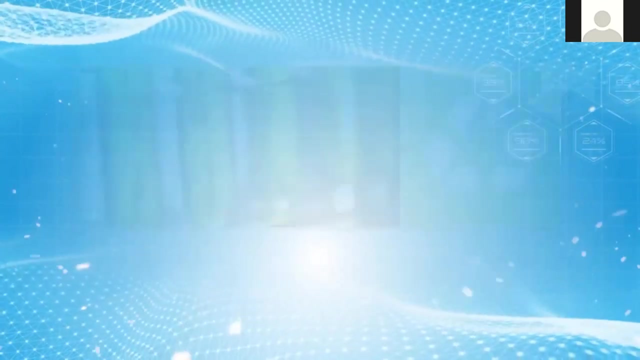 The categories include Animal Sciences, Behavioral and Social Sciences, Biochemistry, Biomedical and Health Sciences, Biomedical Engineering, Cellular and Biomedical Engineering, Biomedical and Molecular Biology, Chemistry, Computational Biology and Bioinformatics, Earth and Environmental Sciences, Embedded Systems, Energy, Sustainable Materials and Design Engineering Mechanics. 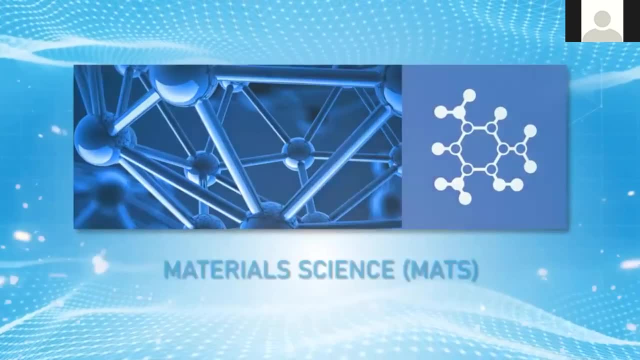 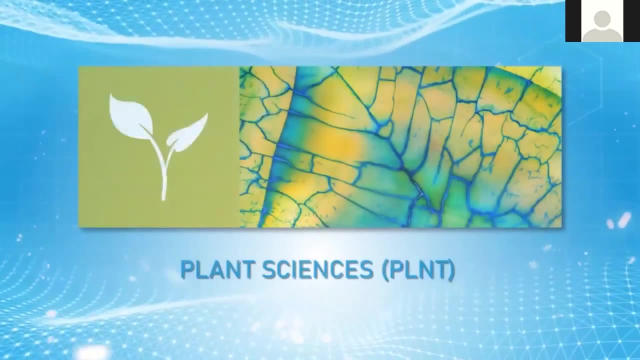 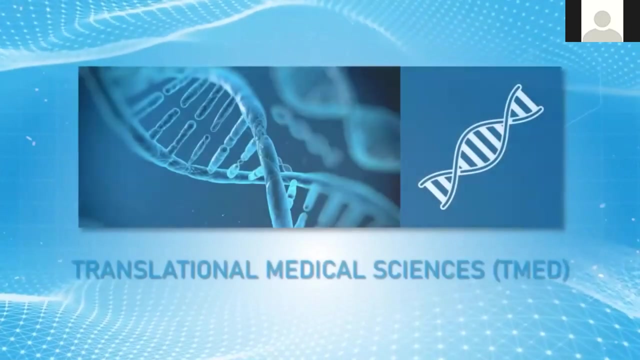 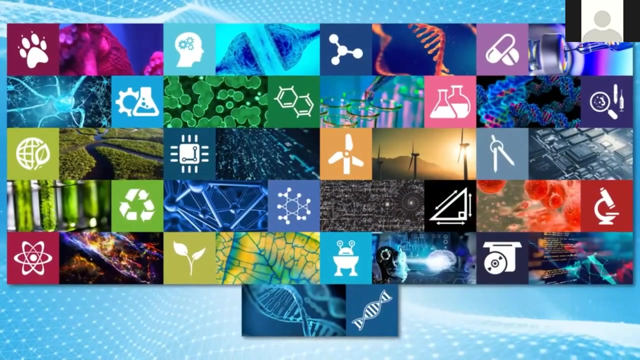 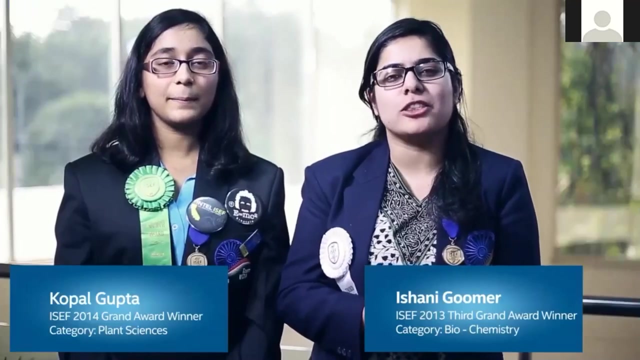 Environmental Engineering, Material Sciences, Mathematics, Microbiology, Physics and Astronomy, Plant Sciences, Robotics and Engineering. You are now ready to take on the challenge. Let's get started. A display shows the public and the judges what you have done. You are looking to attract and inform visitors about your project. 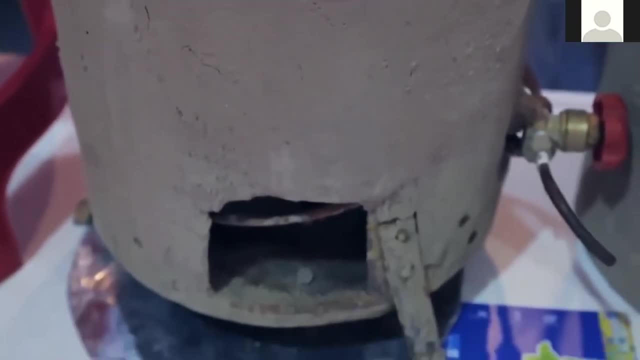 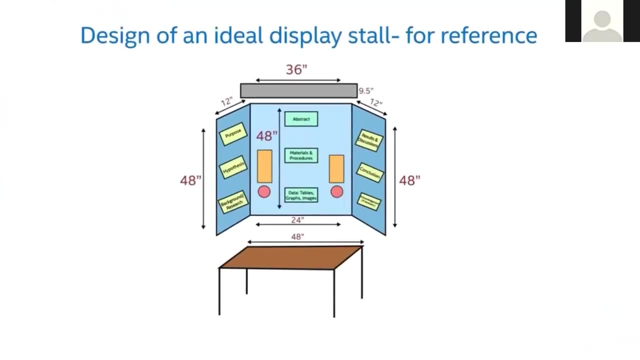 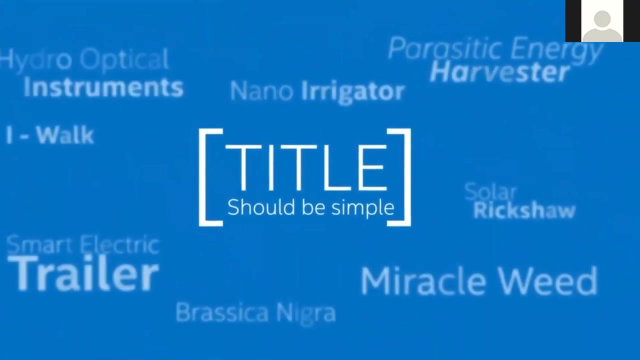 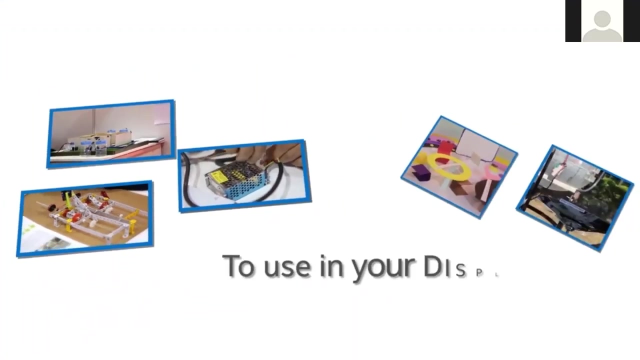 To make it easy for people to access your results by creating a clear, attractive and concise display. The focus should be the work. Take a look at this reference. Your title should be simple and must accurately represent your research. Take photographs or videos of important parts or phases of your experiment to use in your 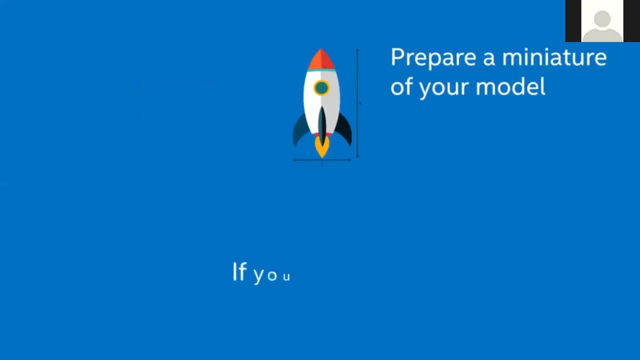 display. Prepare a miniature of your model in case your prototype is too large to be carried along. Make sure your display is logically presented and easy to read. Use neat cut-and-cut images of your model. Make sure your display is logically presented and easy to read. 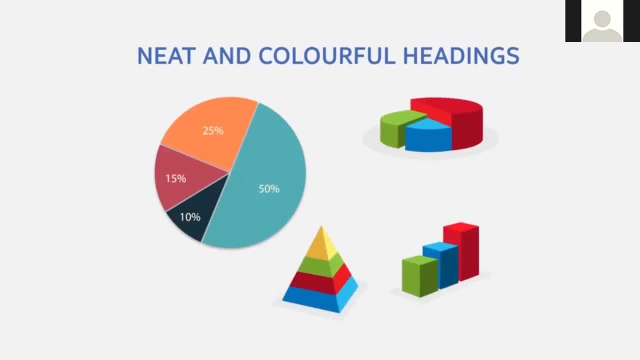 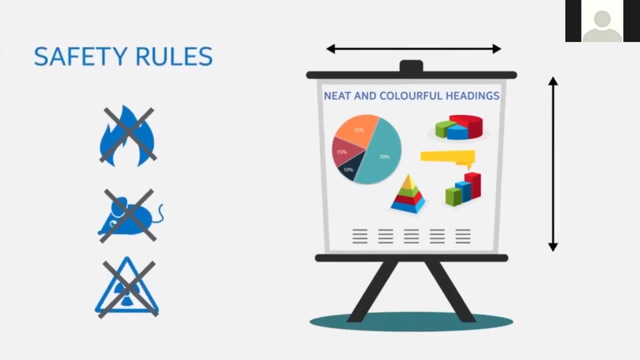 Use neat cut-and-cut images of your model. Use sheetrings. Use sheets of text to create a clear record of your entire experience. Use colourful headings, charts and graphs to present your project. Pay special attention to labelling. Be sure to adhere to the size limitations and safety rules when you're preparing your 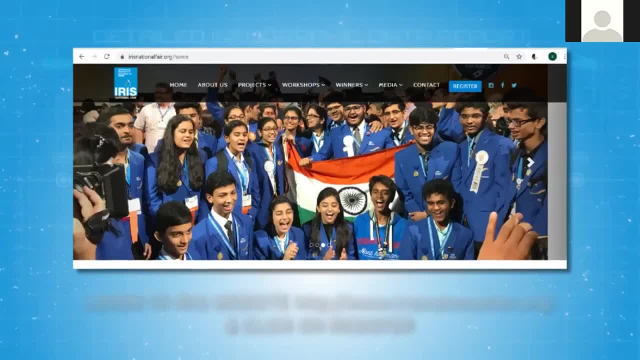 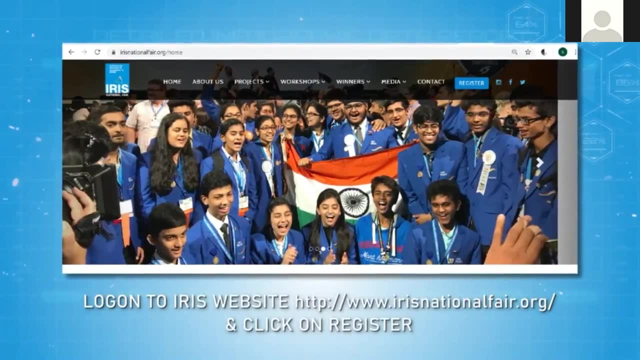 display. The iRis journey begins with registration on the website wwwirisnationalfairorg, with submission of online synopsis. with a sit down we shall cover complete authority, review and translation ofесьing childcare to reinforce��� paranormal history during 했던 events, such as red chalk animal, slnight of riverfront, brown cloud, cossack, daran. As a presentation, you will later get a translation of iRis on average, with contents may be softly version. or지r of Flint or cryptographic Russian characters. 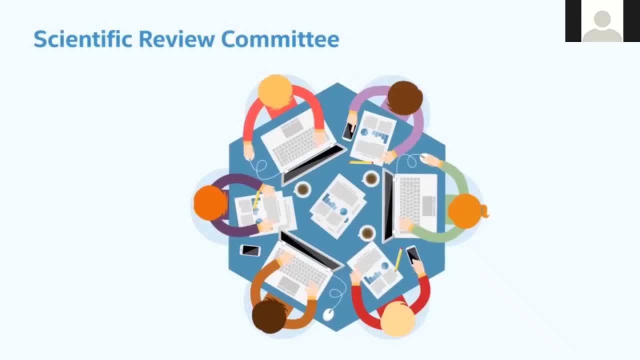 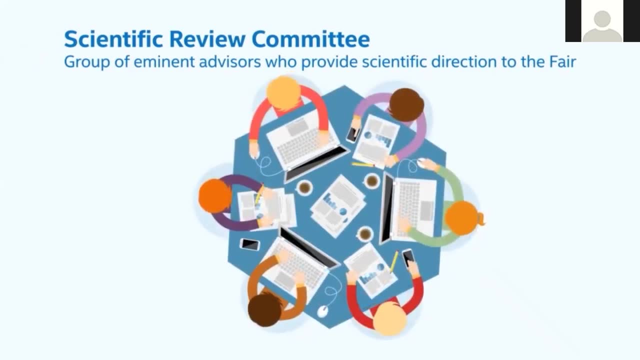 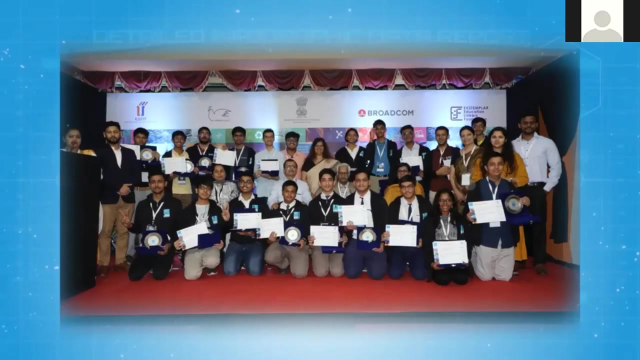 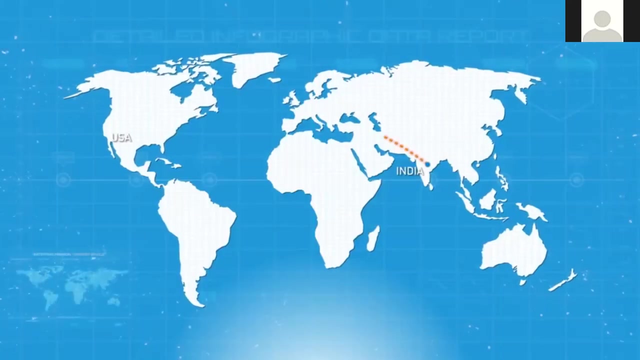 and supporting documents. these entries are prejudged by the iris scientific review committee and shortlisted projects are sent an email inviting them to participate in the iris national science fair. winners of the iris national science fair qualify for an intensive series of mentoring camps and get the opportunity to represent india at platforms such as the. 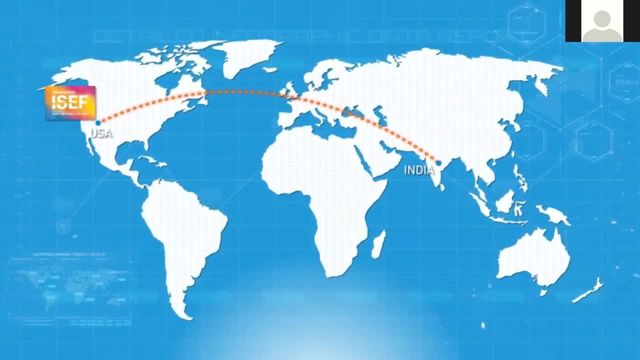 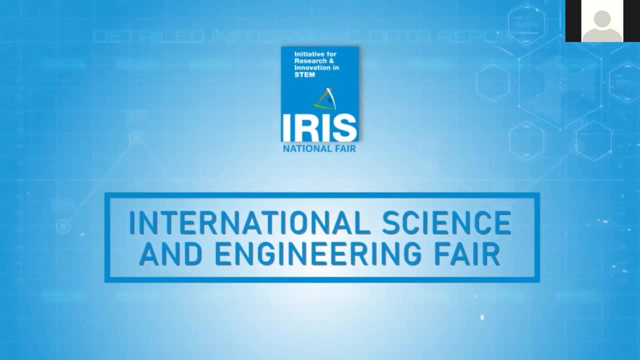 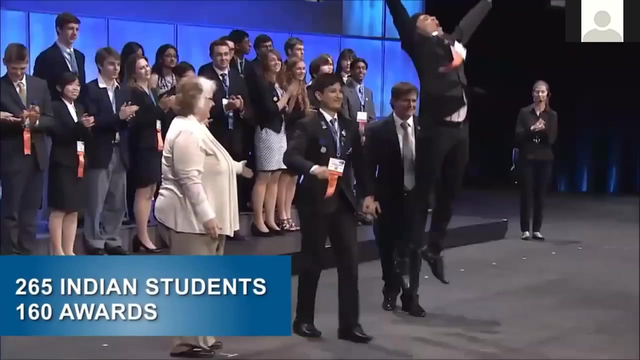 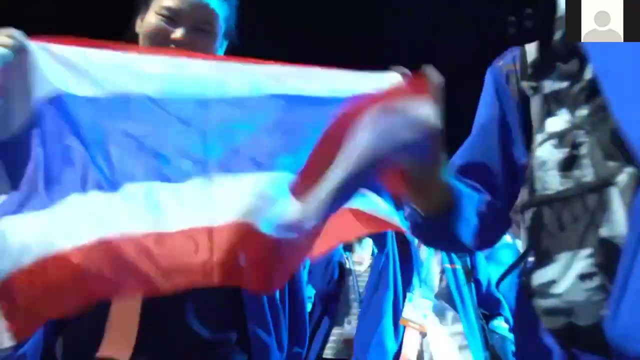 regeneron international science and engineering fair in the united states of america. isef is the world's largest pre-college stem competition. over 265 indian students have won over 160 awards at this competition, competing with over 6 million high school students from all over the world each year. not only are you getting a chance to make your nation, 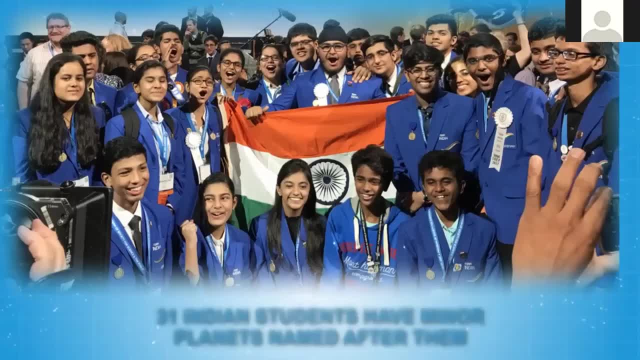 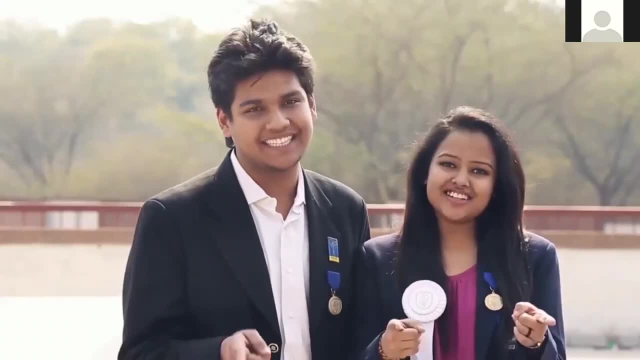 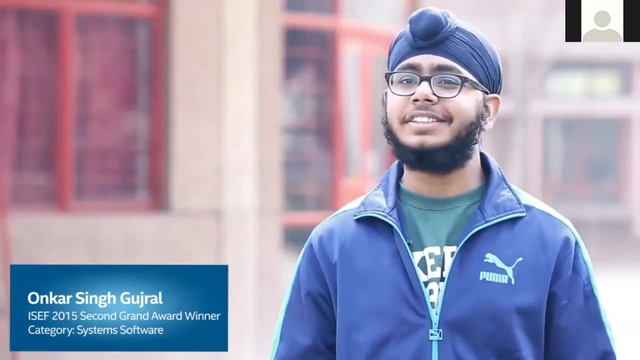 proud, but if you're lucky, you could join the 31 indian students who have had minor planets named after them. so, guys, please don't miss this opportunity. it's your turn now. if you're innovative and you really want to bring about a change in the world, i think iris is the right place. you enjoy science. 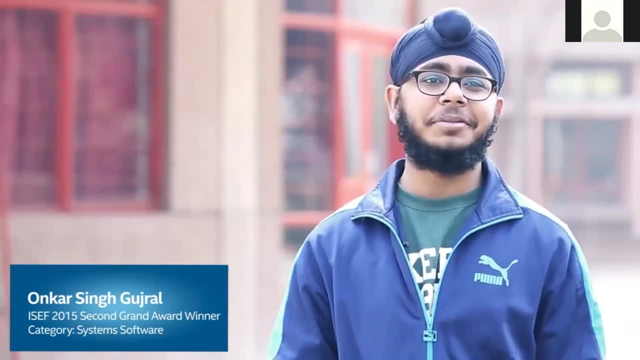 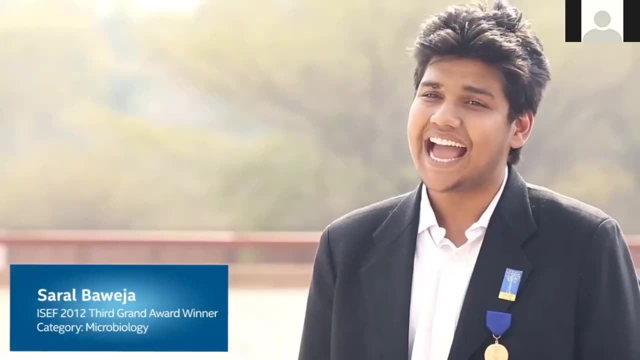 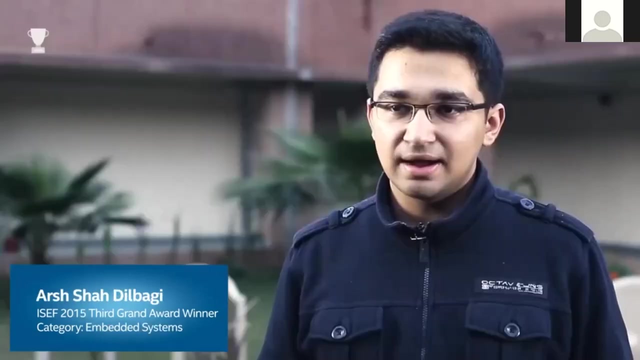 and math and computer science and so on. so i mean it gives you a platform to show what you've done and you have a chance to go to icf2 if science actually kindles your curiosity and you're really passionate about it. iris provides you the largest platform in india to show your talent applying to 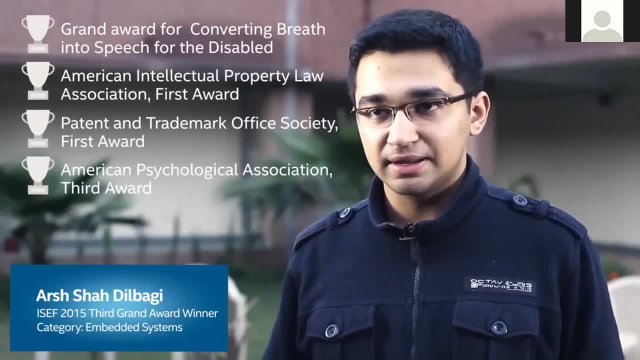 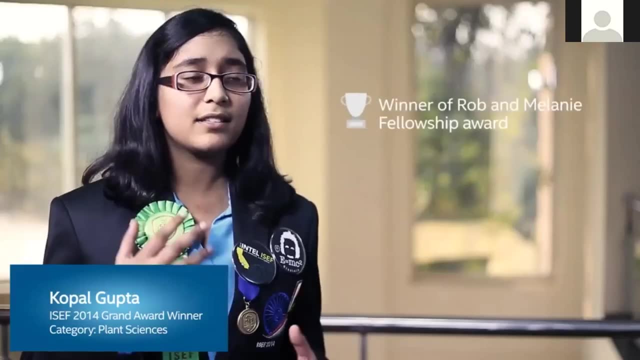 iris not only get to have a great experience, you meet great people and great mentors at that. they're not judges, they're not judging you, they're mentoring you, they're teaching you, they make you learn new things. in the end, it's not about winning or losing, it's about experience and iris. 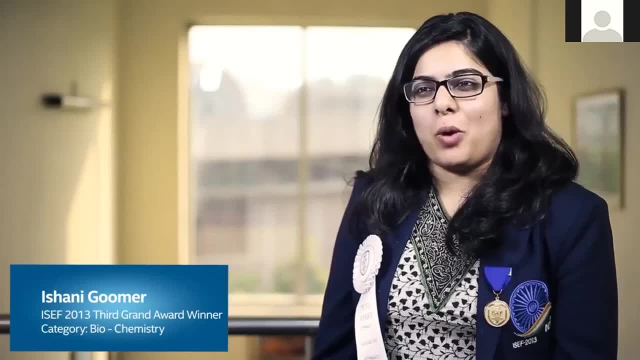 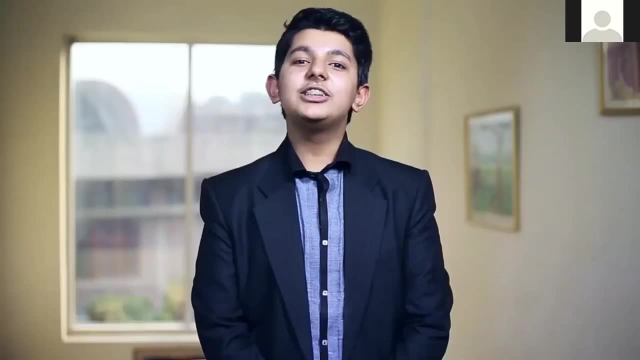 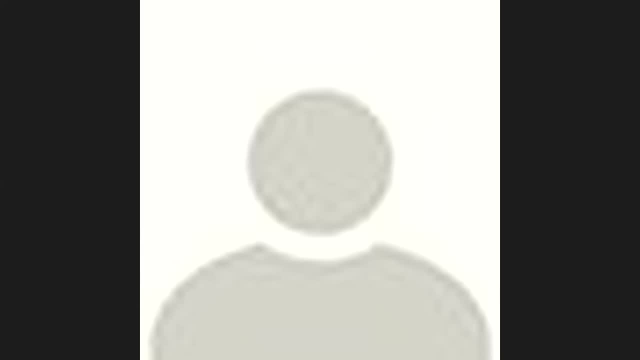 thank you so much. uh, now we will begin the q a session. may request sasha to students to please send their questions on the chat box and my colleague sasha do read out a question to sir. our first question coming in today is from ayushman sahoo. 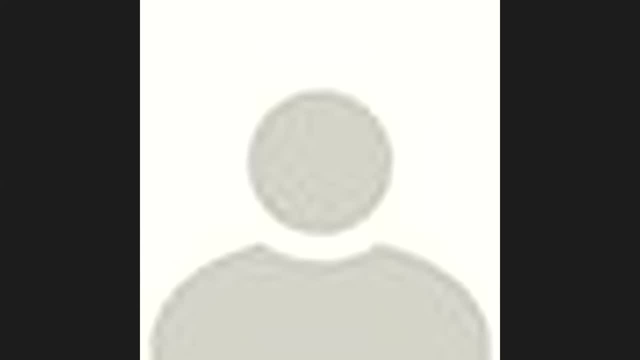 who writes: uh, his doubt was that plants react to our emotion means, if we treat them nicely, they grow. so, uh, the professor, uh, the question is to professor singh as to so what do you think about this? um, she is so there, yeah, well, i do agree with mr sahoo that plants do have emotions and and uh, but i am not a plant scientist or physiologist, so plant physiologist, so i think much. i cannot say. thank you, we have a participant who has raised her hand. uh, sandhya, i will now unmute you and you can ask, sir, your question. 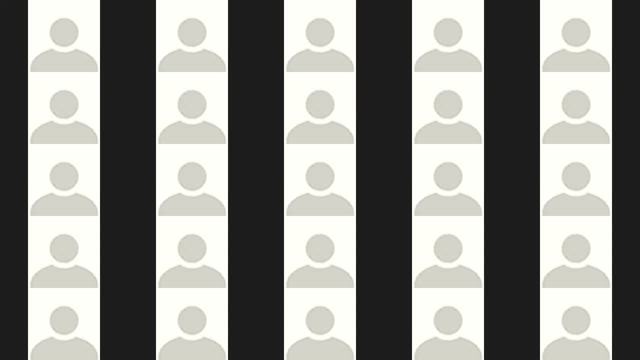 sandhya, please unmute yourself and ask so: yes, okay, am i audible? yes, you're audible. uh, good afternoon to all. uh, sir, my question to you is that, uh, you have shown us wonderful projects, uh, in terms of air pollution and water pollution, and but, sir, like the projects, what you discussed. 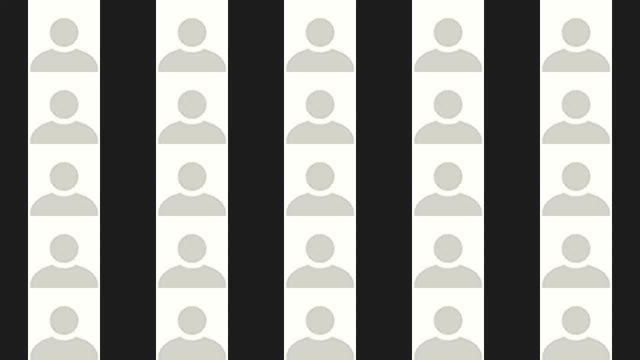 with us. that cost a lot and, of course, these projects have been carried out by the students, and and the students are very interested in the project. so i would like to ask you a question about the project- students at the university and college level. so, sir, i just wanted to know that. is it possible? 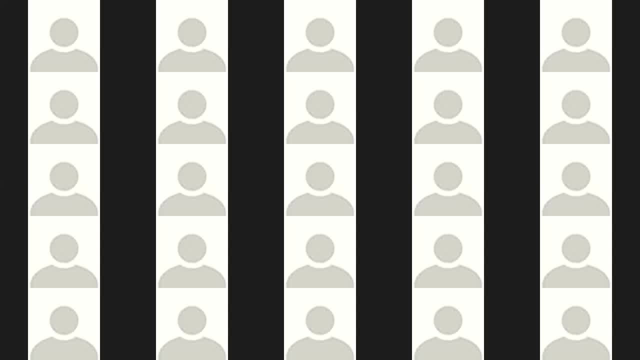 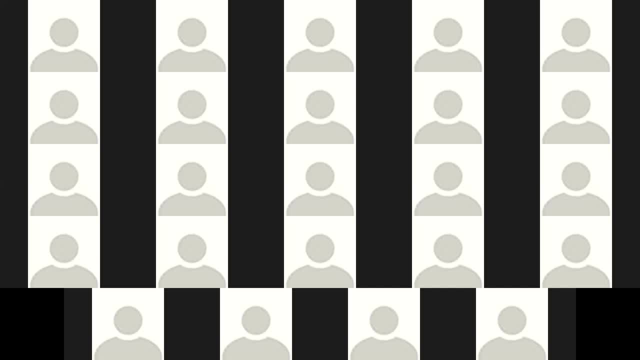 to have a small prototype of these projects at the school level. if we can work with our students, well, sandhya, i don't think that nothing can be done by these students. point one. so there's nothing. college, there's nothing, you know. so i'm 100 sure that any project which i'm 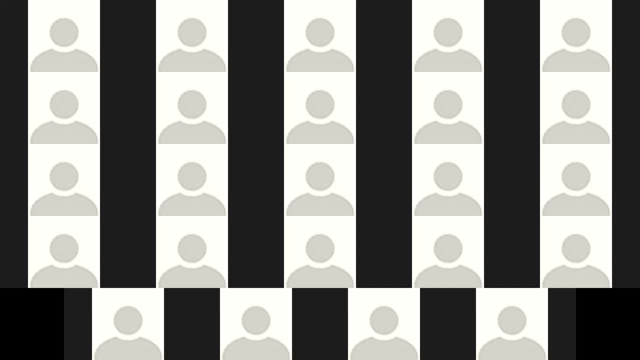 showing can be very well done by these students as well. so that's point one. and of course, uh, there are many, many projects, you know, which can be taken, and uh, certainly, actually, we can prepare a list as well, you know, and then we can circulate to these students. i will request saksha to uh, please you. 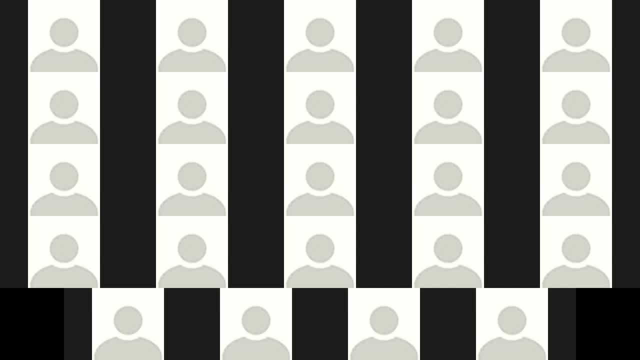 know, take a note of this one. and uh, we will certainly, you know, give those projects to these students as well. so maybe one additional uh list, i think we will circulate and they can do, but here there is nothing you know big, which these students cannot do, believe me, i'm telling you. thank you so much, sir, because we have worked in. 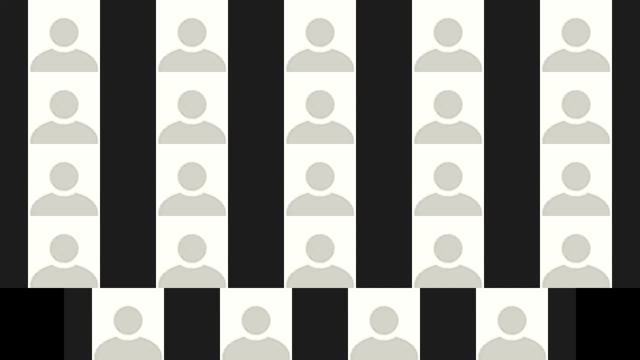 our school on a project, uh, namely biofuels. uh, what the slide. you had shown us that because of burning of fuels near in the nearby areas of delhi, the air is getting polluted over there. so we tried making the project over there, but due to many hindrances, and you know to find the right way to do it. 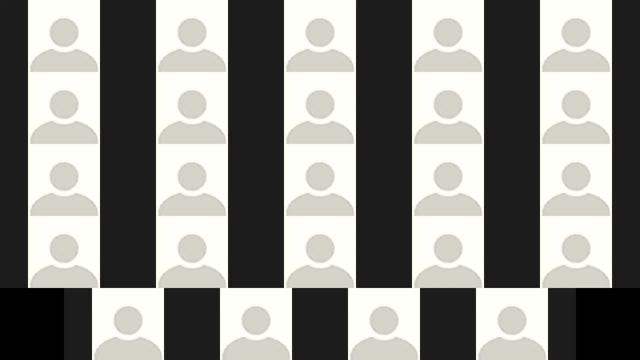 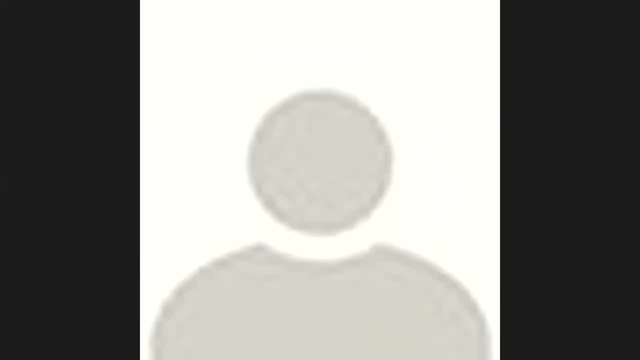 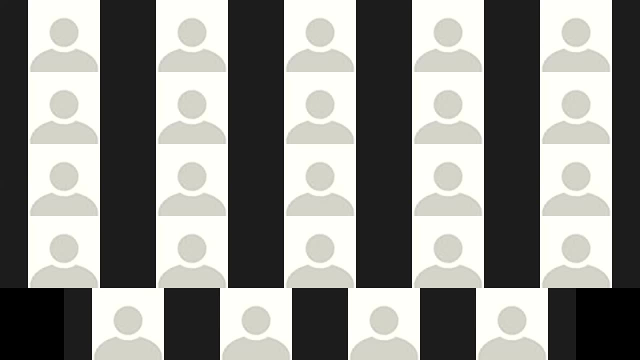 our limitations, we could not work more. so when i saw the kind of work you have shown us, that really motivates me to carry on the project once again. yeah, sandhya ma'am, i will request you that you please try once again, because many times what happens that you know we do not get time, or you? 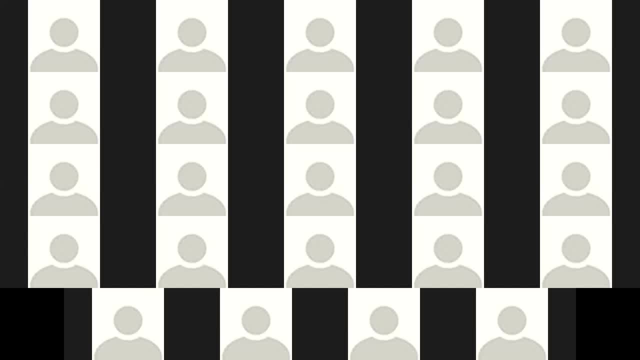 know, sometimes students get busy and sometimes something happens. but uh, please, uh, never. you know, my point is that underestimate the power of the students and, uh, in case, if you feel uh, and if shasha and shreya they are shrey, they are okay, i can also help you out, you know, in doing some of those projects. 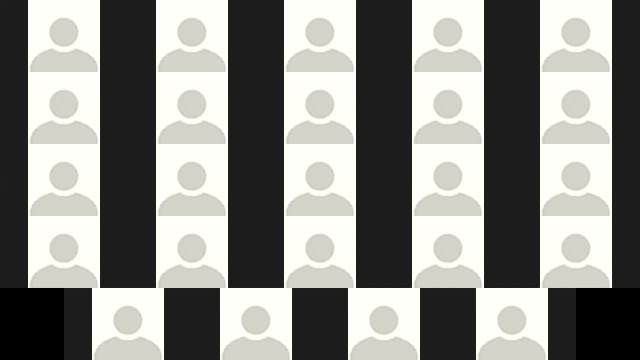 absolutely, absolutely okay. so it's no issue, thank you. thank you so much. there's a question coming in from dr yugender kumar kothari, for team iris. uh, sir, writes during covert period. how can you conduct the event? uh, so this is something that the iris team has been mentioning, webinar after webinar, that uh. 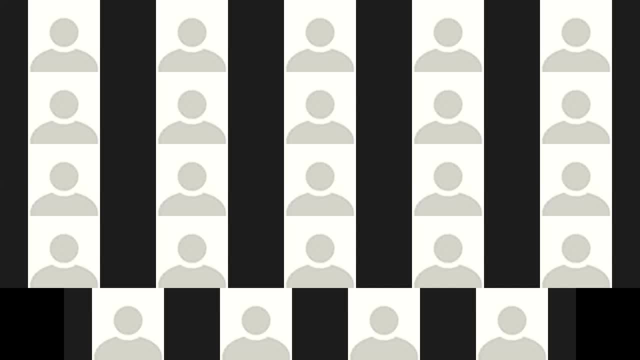 and according to the iris cycle, the iris national fair takes place in uh december and january, so we still have a very long time to go to to determine whether we're going to have the fair in person or whether it's going to be a virtual online fair. 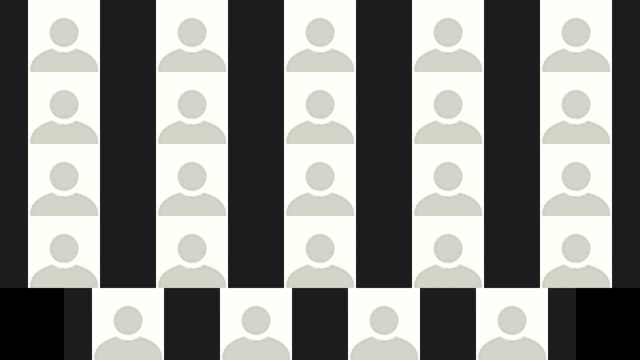 however, we are proceeding with the submission process and a pre-national fair evaluation as scheduled, and we will be putting it up on the website when it is uh time to decide whether or not we're going to have the fair in person. a lot of covert vaccines do seem to be in the pipeline. 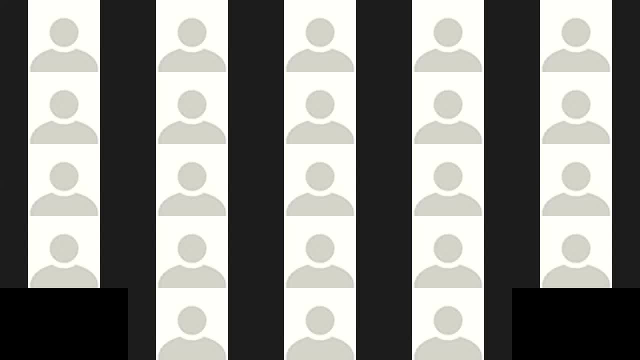 and hopefully by then we should have something that will permit us to have the fair in person. ayushman, you have your hand raised. uh, i will now ask you to unmute and you can ask professor singh your question. good evening, sir. sir, am i audible very well? 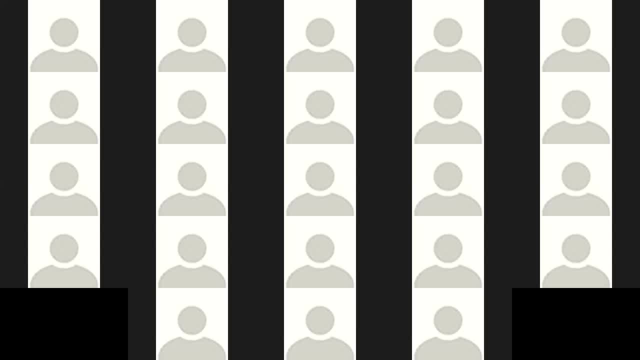 project that we can store water in plants, sir. what do you think, sir, can? uh, so the water? we will be nice when we will store it in plants, and will it be equal to the roof water harvesting which we do, or it will be much better than it? 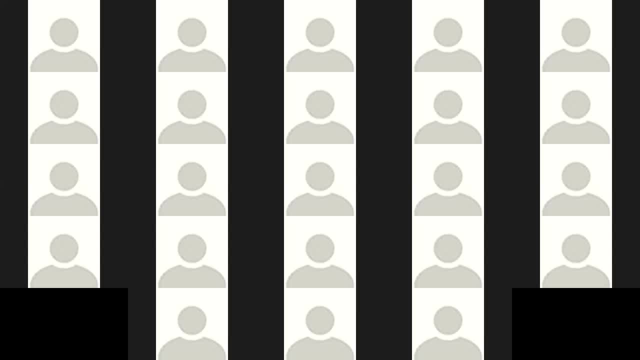 no, i mean, uh, the putting waters in plant in order, to you know, means so called remove certain metals and certain impurities from water. it's very old, actually, indian technique. we have been using, you know this technique almost for, i think, uh, at least three, four thousand years, so this is absolutely no problem. i mean, so you can. 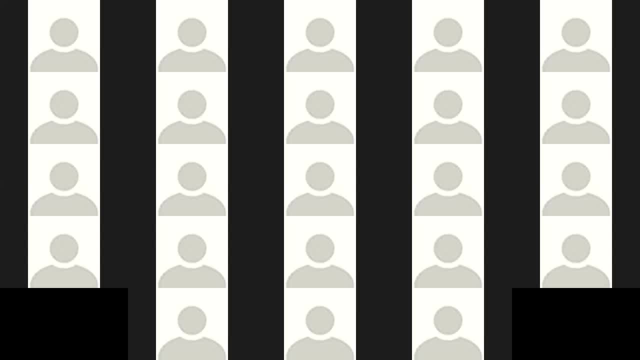 use that. uh, the only problem with the- you know this bioremediation comes that the volume of water normally becomes either half or, if sometime it becomes, let's say, 60, yeah, so this means you lose a lot of water actually. so, in case if there is a problem, then you can start to use your water in an 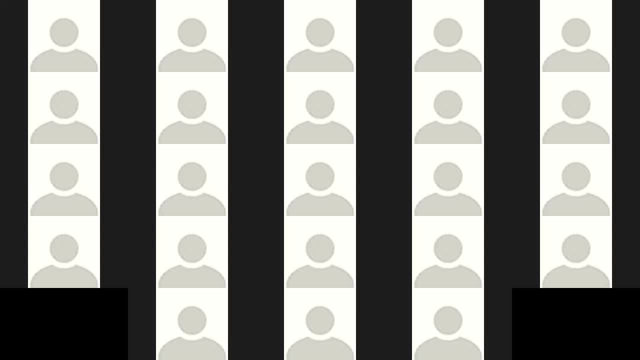 is a problem, and then I mean you should use the other methods. but, for example, if you're living in Orissa, where the water is, you know, much more available, then it's absolutely okay, and there are, you know, examples in Orissa where they have used, actually, I mean plants. 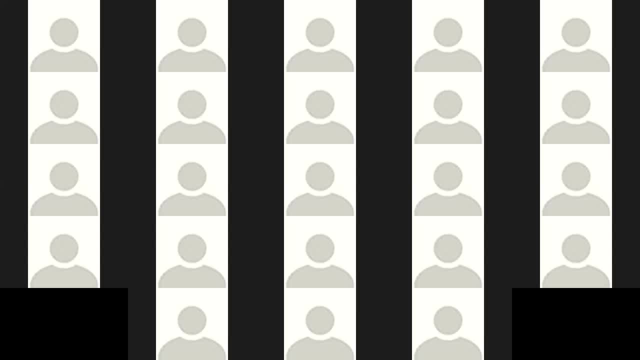 for I mean treating the water, base water. yes, I was thinking of storing the rain water in this, in the plants. rain water in the plants, yes, sir, okay, like in the hollow plants, we can store, yeah, but then again you know what happens, that let me tell you, Mr Sahu. 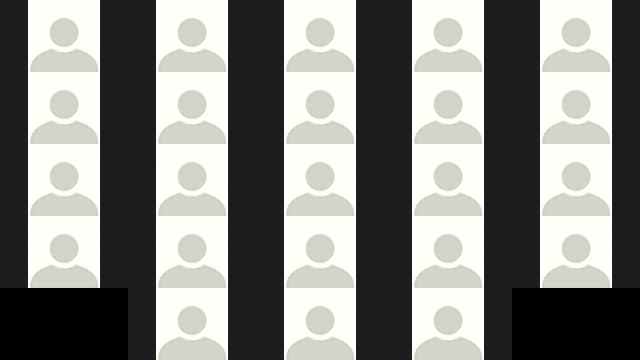 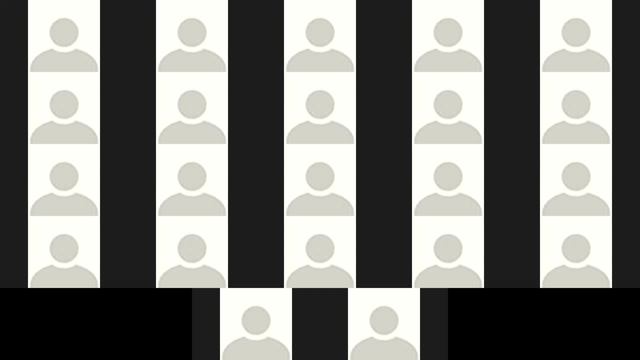 what happens that Ayushman, that plant, normally respite more water, respite, you understand. so one process is respiration. yeah, so this means plant drink water and if the temperature is high, you know, then they evaporate this water directly, actually in the atmosphere, and this rate of evaporation could be is high. 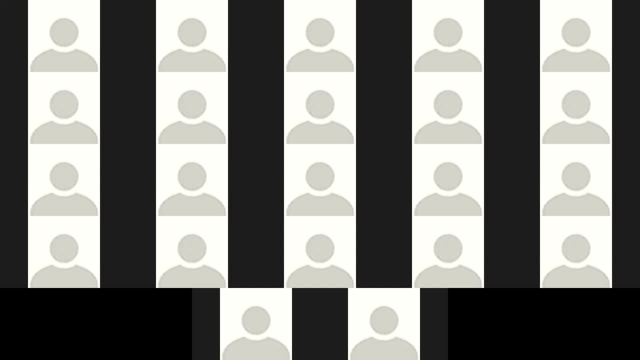 is, let's say, four, five millimeter, yeah, per day. so have you understood me? so this means each day. I mean, it's like almost like a lake, yeah, so if you have a lake and if you have stored the water and if the temperature is, let's say, 45 degree, then the evaporation from lake is approximately. 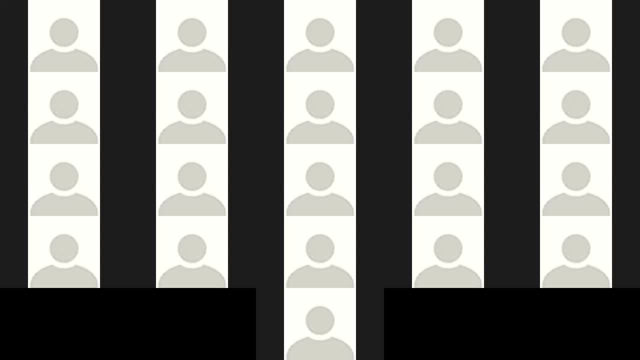 four, five millimeter per day, and if you have plant, and these plants will also throw a lot of water into the, into the air. so I don't think that this should not be a good idea. I mean, if your water is actually limited and but then how will you take out water from the plants? 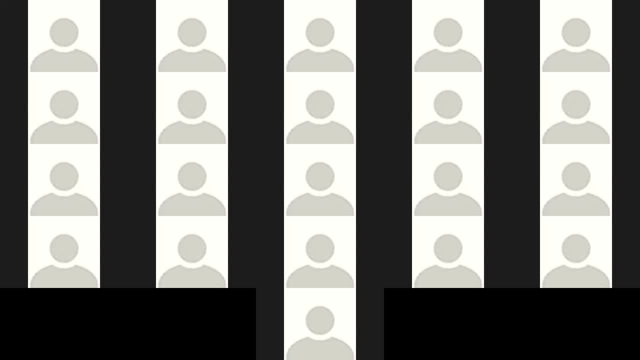 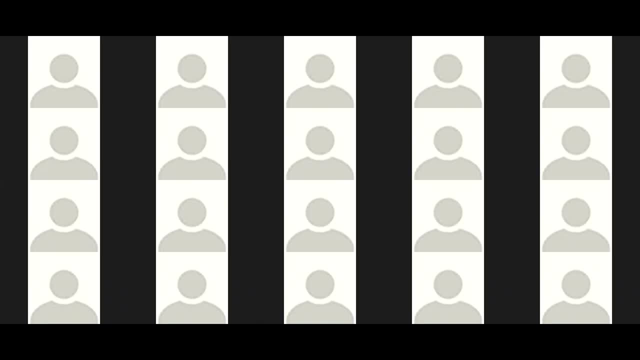 sir, I was thinking of some after the water is stored so we can, as I was thinking to, make a hole in that and use it one. I would just like to stop you over here because, at the end of the day, platform and we would request you to refrain from sharing any ideas that you 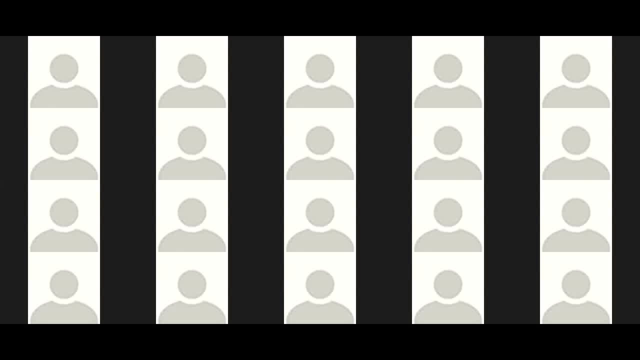 may use towards the development of your project. You can get in touch with the IRIS team on contact at irisnationalfireorg and we will get you in touch with Professor Singh if you have to discuss anything that is pertaining to a project idea with him. 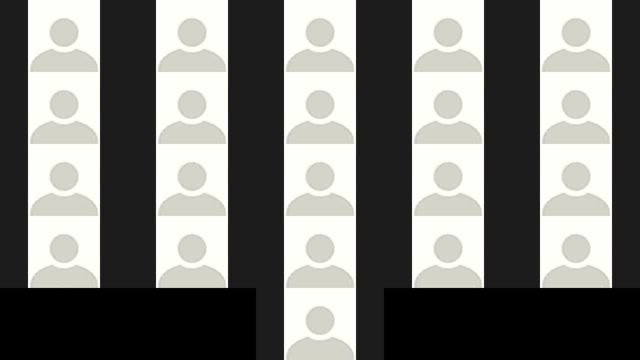 Yeah, Aishman, so I think it's a very good point. you know Shasha has mentioned, and I appreciate actually that ideas are always very valuable. So, you know, really keep them very close to your heart and also, while we are doing a lot,